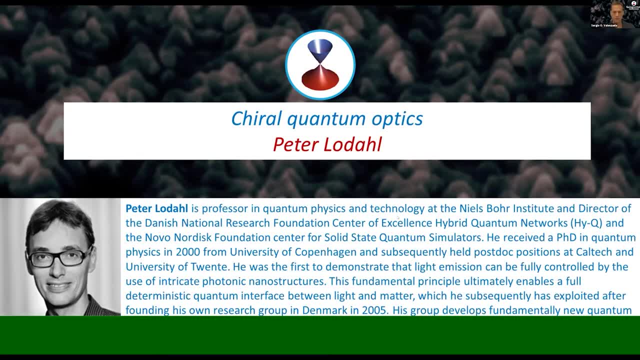 National Research Foundation Center of Excellence in Hybrid Quantum Networks and he groups develops fundamental new quantum hardware for the emerging field of quantum information science, such as thermonuclear single photon sources, single photon interfaces and quantum gates. Note that during the talk you can ask questions in two ways. One of them is by raising your hand. 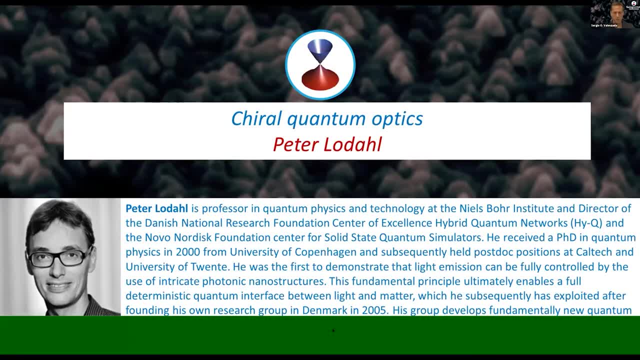 by clicking, at the bottom of the screen, the icon, or by directly typing in the the questions with the Q&A icon that you have also in the bottom, And then you need to wait for Peter to give you the the word for him to read the question, or let us give you the. 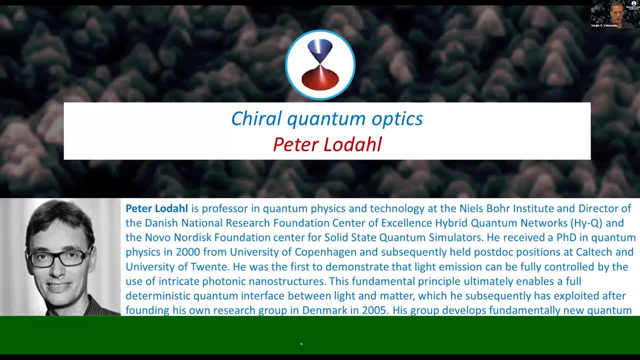 microphone, so you ask the question yourself. Now I noticed that there are many of you already connected in YouTube. Take into account that we will not be able to interact with you. Try to. if you want to make a question and interact with the speaker, please make sure to. 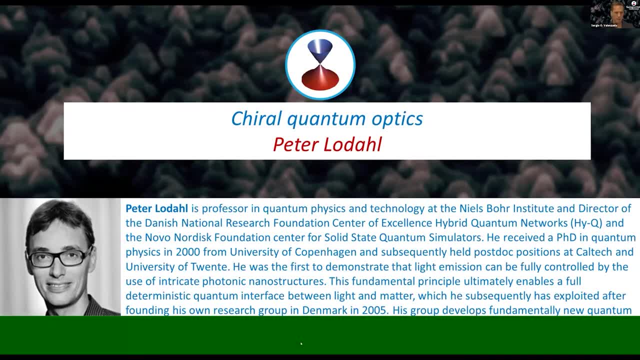 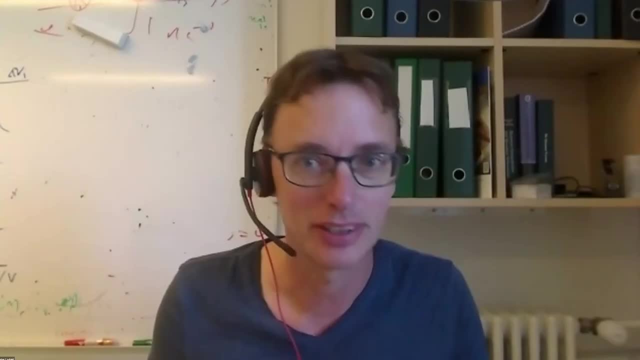 connect with Zoom. So with this, I give the the word to Peter and I'll let you share your screen. Thank you and welcome to the conference. Thank you very much, Sergio. You can hear me? Yes, Perfect. So thank you very much for the very kind introduction and the 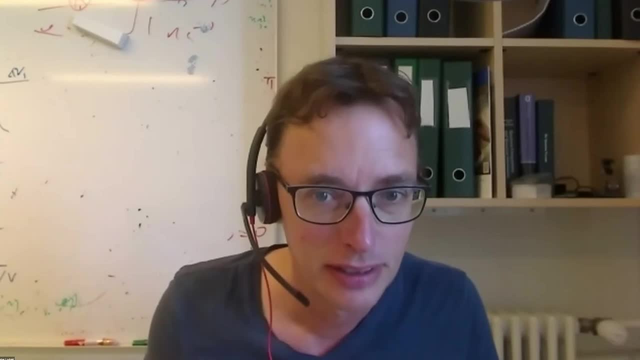 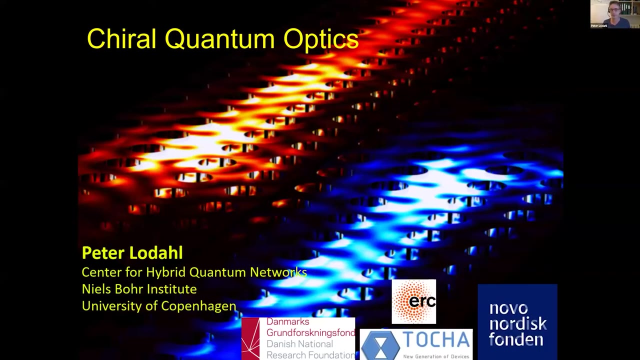 opportunity to speak. I will share my screen. Thank you very much for the very kind introduction and the opportunity to speak. I will share my screen. See the right one now? Yes, I think so. yeah, So let me just get the pointer also just a second. 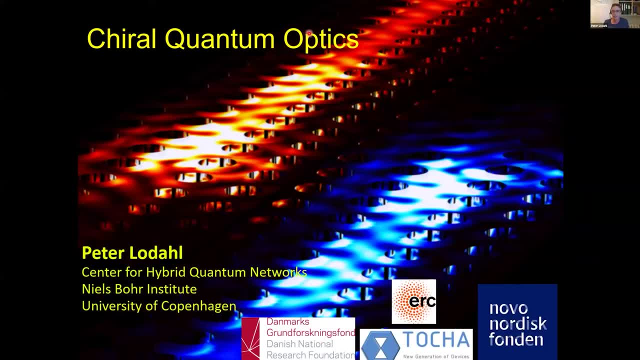 Yes, and I think we all said Yeah. thank you very much, Sergio. It's a real pleasure to give an introduction to the area of photonics and, in particular, also the quantum properties of light-matter interaction, and speak about introduce the concept that we call Kyle quantum optics. So this is really about 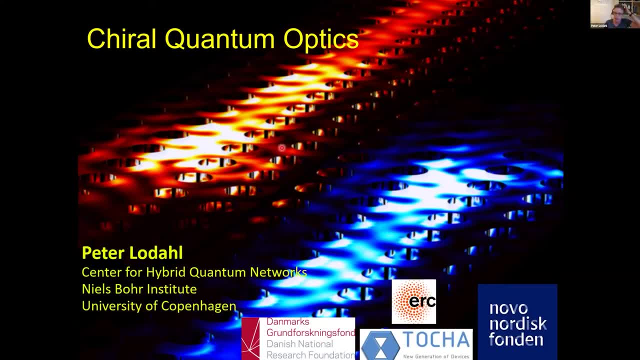 directional emission and directional light-matter interaction. It may be topological or it may be not topological. I'll return to that later. So what we're really particularly interested in is the ability to engineer light-matter interaction and play tricks with light transport. 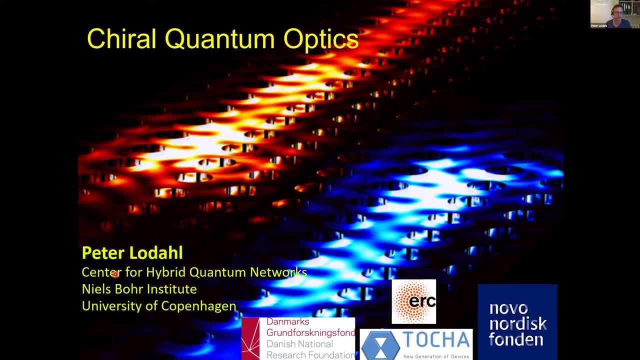 So what we're really particularly interested in is the ability to engineer light-matter interaction and play tricks with light transport and light emission. I'm headed here at the Niels Bohr Institute at University of Copenhagen, and here you see some of the founders, and indeed Todtje, that Sergio introduced. We are very happy to be part of that. 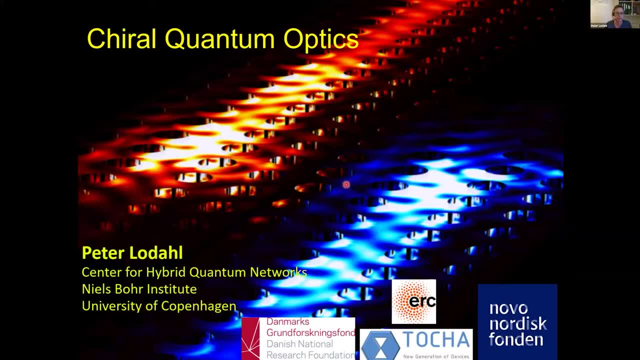 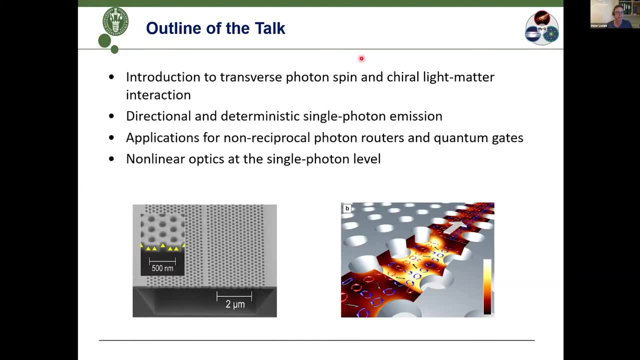 very nice and interdisciplinary project. So this is the outline of what I will be speaking about. I will introduce a Kyle light-matter interaction, I'll introduce the notion of a transverse photon spin and then I will explain in more details how that gives rise to directional photon emission and single photon emission in particular. 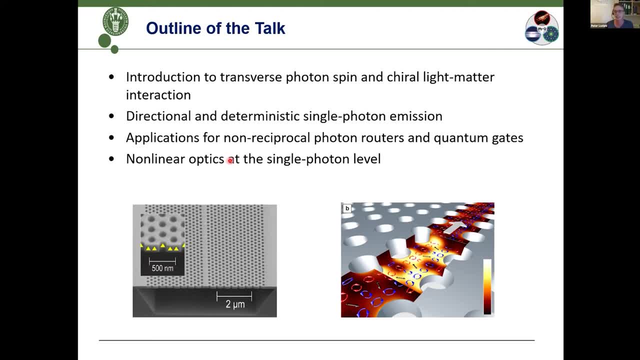 and also that this can be deterministic, and this is really the key of what we can do, also for the, to build technology based on this that you can really get single emitters interacting with single photons near deterministically. I'll say something about the applications that can be foreseen. I'll explain about how we can make non-reciprocal. 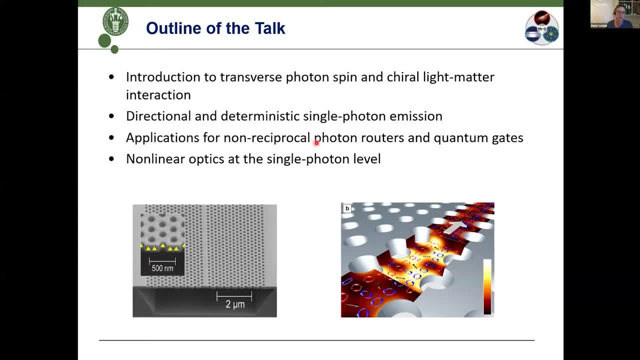 photon transport, So we can route photons so that there's a difference between back and forward, backwards and forward, and we can do it with quantum interaction. So that means we can also do it in quantum superpositions. I'll say a little bit about some of the applications in quantum. 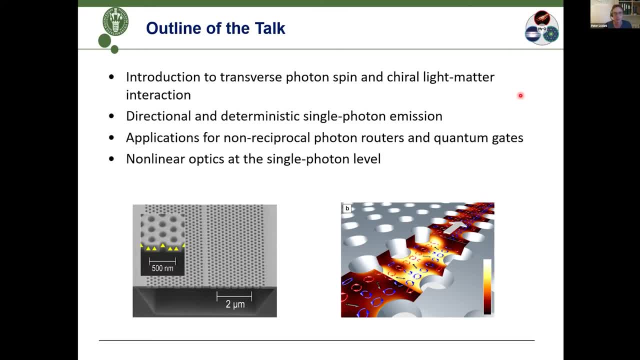 information processing that are foreseen. Probably I'll not go too deep into these details about how we can make quantum gates and multi-photon entangled state based on the some of these concepts I'll also touch briefly upon about upon non-linear properties of this light matter interface and how 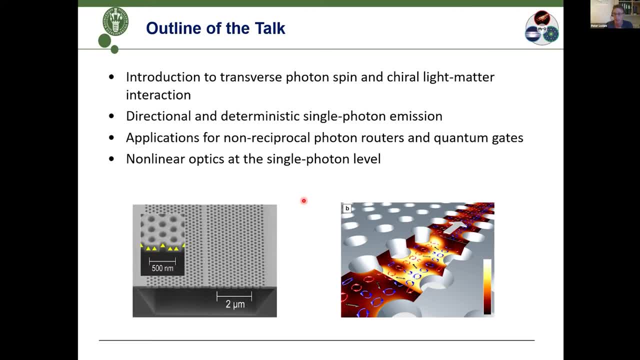 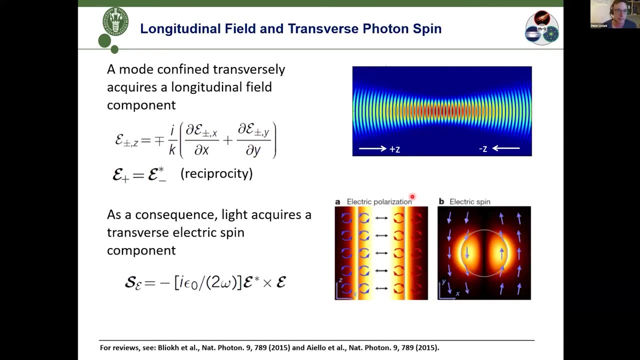 the non-linearity can operate at the single photon level and please, as Sergio already said, please just raise your hand and ask questions as we go along. that will make it easier for me to adapt to the audience. So light transport and the longitudinal electric field and the transverse photon spin, So 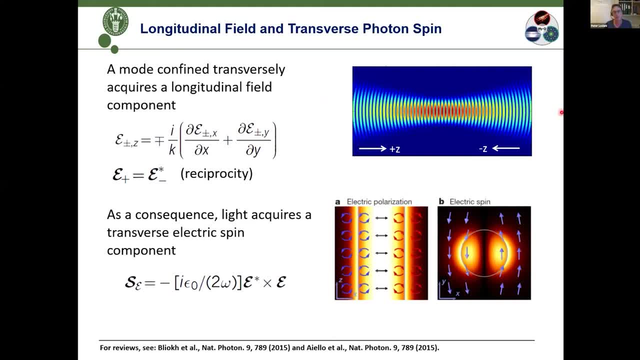 uh, in optics, uh, we are used to, uh, we have beams that are propagating. here's the gaussian beam that can propagate along the plus z direction or along the minus z direction, just for simplicity. So that's a gaussian beam that propagates. We're used to think of photons as our light, as being. 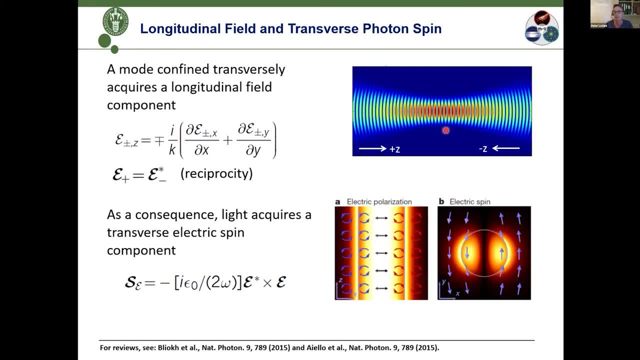 transversely polarized. So you'll have a propagation direction here that is in the plus z direction, and then you'll have the electric field pointing in the transverse direction, either in the x or the y direction, or it could be in the z direction or in the y direction, or it could be in the 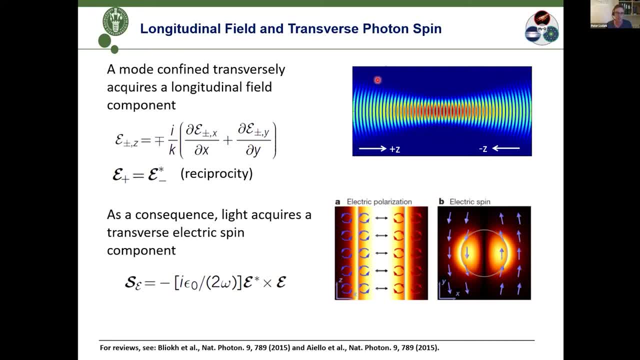 circular polarization, a combination of x and y. However, this is an approximation actually, because we know from Maxwell's equations the divergence of the electric field has to be equal to zero and free space and that actually means that you have a, so dd, dx, dx plus dy, dy plus dz, dz is equal to zero. 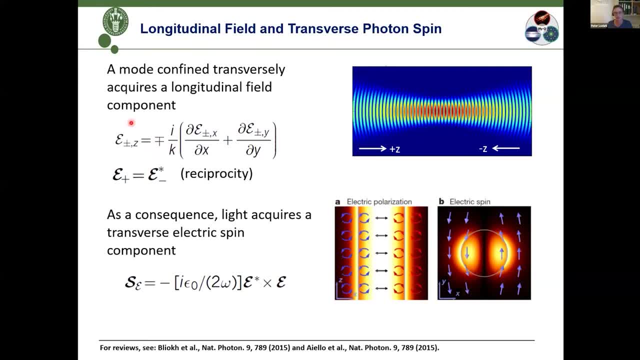 that actually gives a longitudinal component of the field, a component along the z direction. So that's just from from diverging to v being equal to zero, I get a longitudinal component that is equal to this expression here, and normally often we can neglect this contribution because 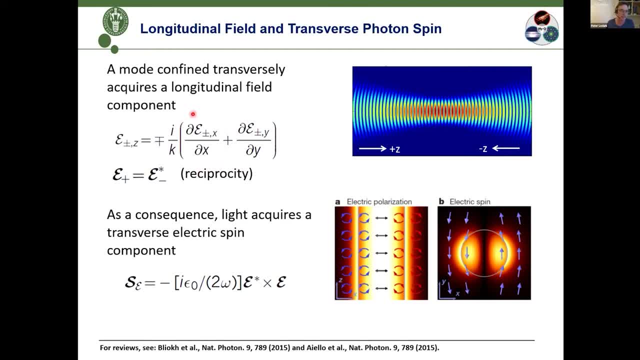 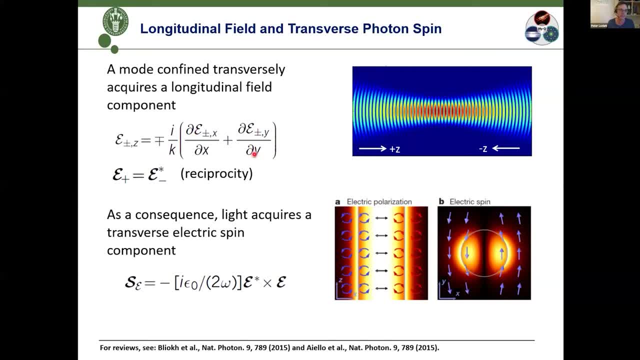 a length scale here. So if I have a transverse variation of the electric field on the order of the wavelengths, then I actually get a longitudinal component of the electric field as well. Often this is neglect. we can neglect that, but in the nanostructures that we are, I'll be 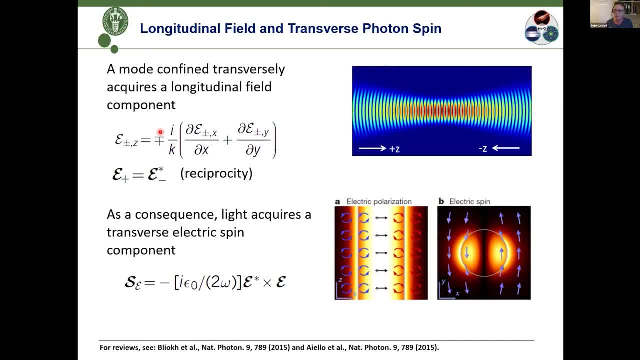 introducing here. we are starting to confine light to a link scale, to a spatial transverse link scale, here on the order of the wavelengths. and then we cannot neglect this longitudinal component of the electric field anymore. and the electric field is not fully transverse. i get a longitudinal component, okay. another thing we need to understand. 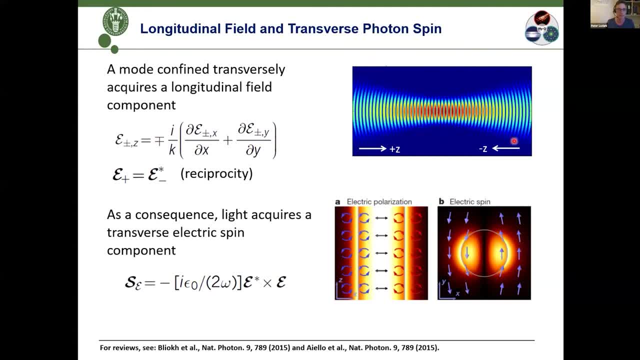 is that? uh, well, moving forward along this plus set direction and moving backward along the minus set direction. well, the electric field is a complex conjugate of each other, that's reciprocity of maxwell's equations. it's not that i'll have electric field moving forward and nothing moving. 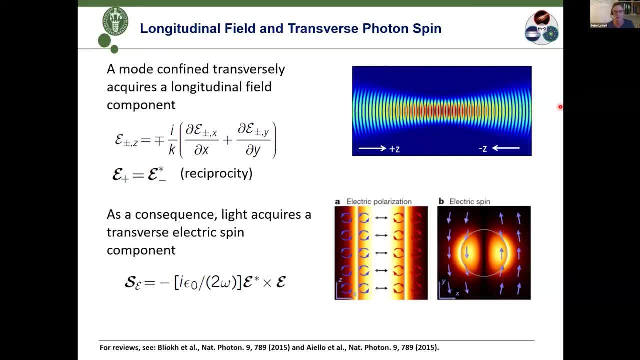 in the in the backward direction. that's not allowed by reciprocity, but i have a complex conjugation there. so that means the longitudinal components of field moving in the minus set direction gets a a sign change compared to the longitudinal component moving in the in the forward. 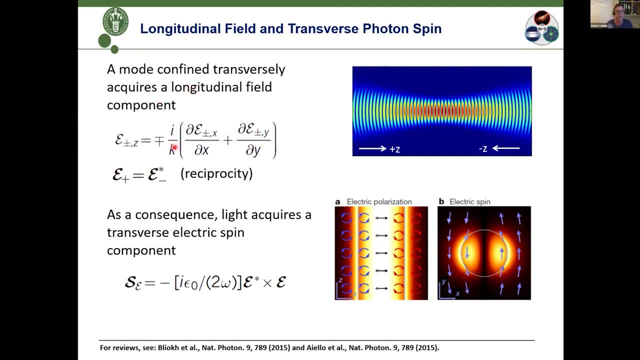 direction. you also see there's an imaginary unit here, so it's it's out of phase with the, with the transverse components, ex and ey. okay, so this is something that we are usually, or often just neglecting. in optics, we're assuming the field should be transversely confined or transversely. 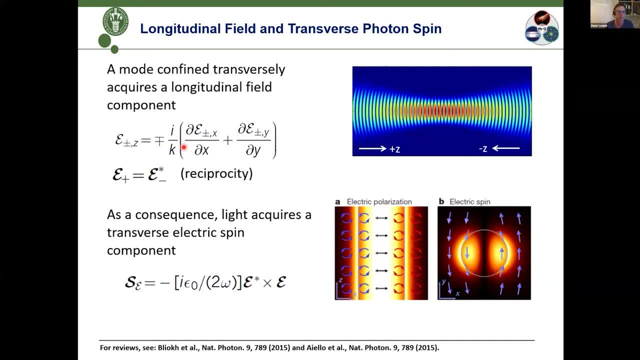 polarized, sorry, which is perfectly fine in many cases where we don't confine light to to these wavelengths length scales, but that's exactly what we do in the, in the photonic nanostructures, as we will be talking about today. so therefore, this longitudinal component comes into play. that also means that if i calculate the spin of the of the field of the 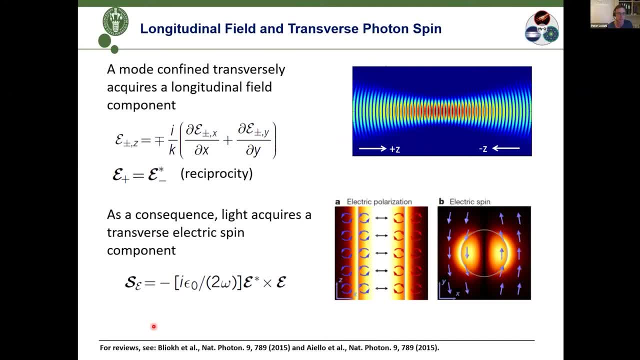 light field and spin of the photons. so you see the mathematical expression given here. well then, if i have transverse, like linear polarization for instance here, then i'll have a spin pointing along the propagation direction. but now i start to have an electric field. sorry, pointed along the propagation direction. that means 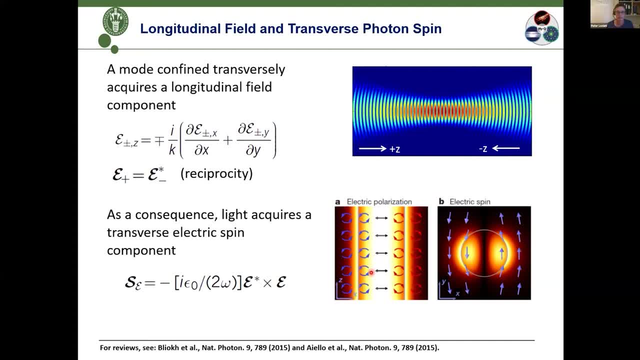 i get a transverse component of the spin as well and that you see illustrated here and calculated for a very simple structure. so this is just an optical fiber. you see optical fiber from from the top essentially so, but it's a fiber that is tapered to the to a length scale that is comparable. 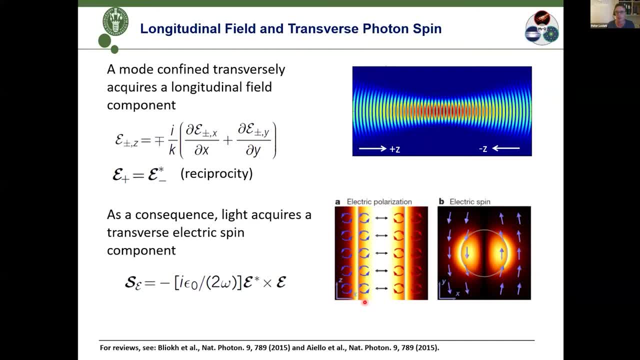 to the wavelength. so a few hundred nanometers or 500 nanometers would be a typical length scale in in photonics. and you see if i calculate the polarization well then it depends on where i am spatially here. she said it's a propagation direction, x is transverse direction. if you're here. 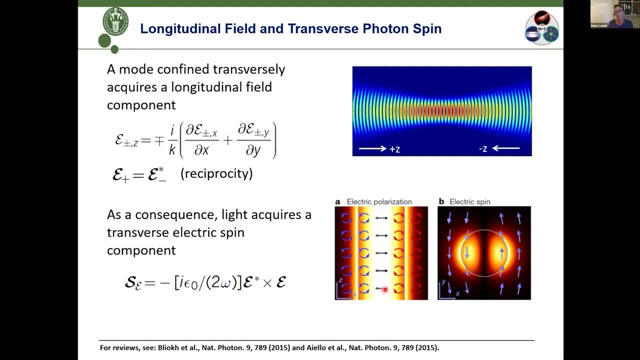 in the center of the fiber. well then, the polarization is is primarily linear. uh, you have a linear transverse polarization, but as you start to go closer and closer to the rim of the fiber- which is right here- then you start to get a more and more sizable longitudinal. 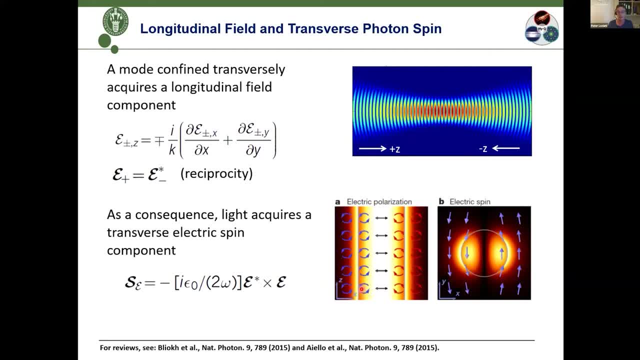 component than what i introduced before and you actually start can get almost circularly polarization: uh, here at the um, at the, at the rim of the of the fiber, uh, so you got get a transverse variation of the polarization. if i equate the spin then i mean it means uh, as i 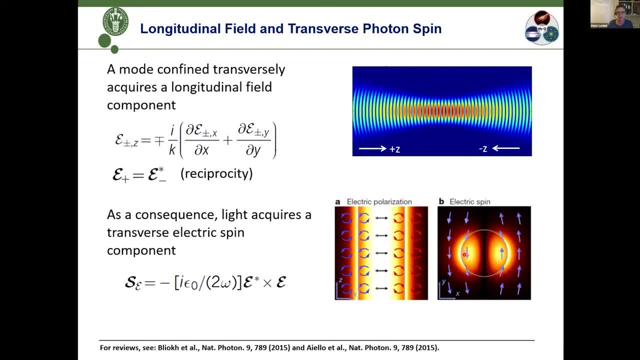 explained over here. you also get a transverse component of the spin. so here you see this transverse component of the spin now in the y x plane. so this is a cut through the fiber and you see, here, next to the close to the rim, you start to get a sizeable. 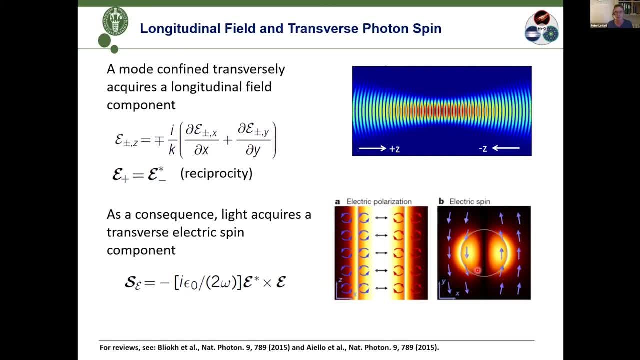 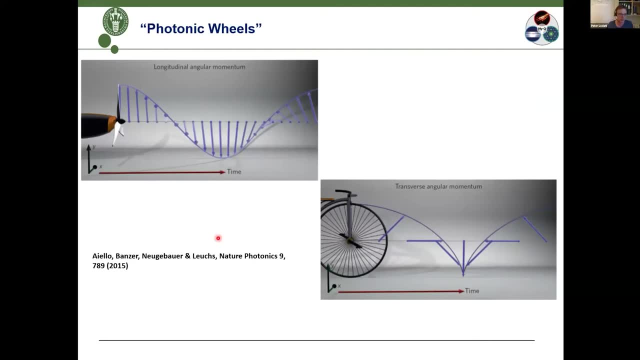 spin component and it changes sign going between plus x and minus x. Okay, so that was the basics of this longitudinal component of the electric field and the transverse photo spin. So there's a nice review paper written a few years ago by the group of 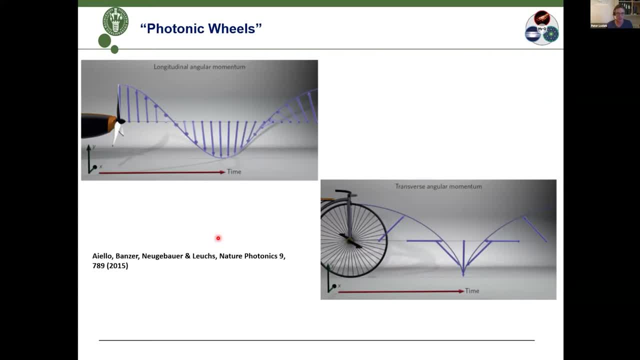 Gerd Loix, who's introducing these transverse spin and the longitudinal electric field, and speaking about illustrating it with these illustrations here, saying that the transverse polarization that we're used to, that's like this propeller field here, where the electric field is rotating transversely in the plane. that gives you a 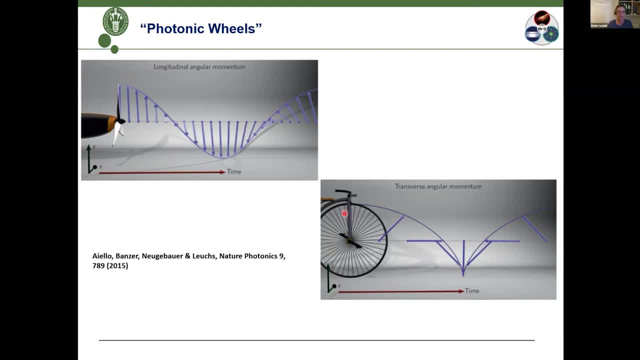 longitudinal spin component. But there's another opportunity: that would be like a bicycle wheel that rotates in the other directions, that gives transverse longitudinal spin component and then a longitudinal electric field component would be the electric field analog of that. Okay, so since we're doing quantum optics, we are very much interested in what are the quantum 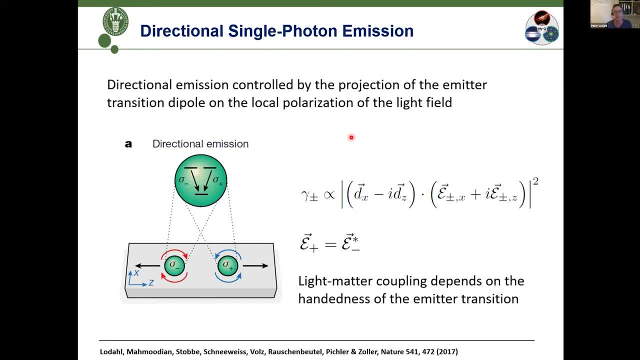 optics: applications or implications of this longitudinal electric field. And then we have to go back to our textbook, quantum optics. What is the essence of quantum optics? that is, how does light and matter interact with each other? The first thing that we say every time we give the 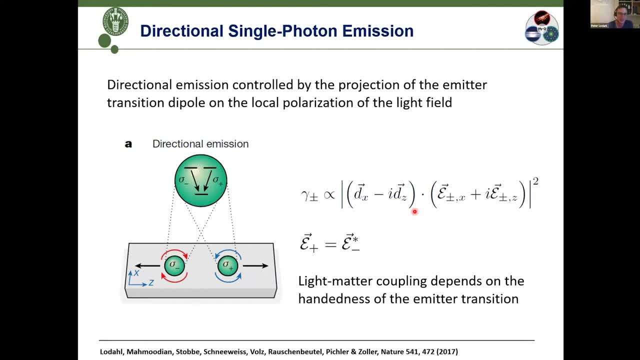 quantum optics lecture is that. well, you have to remember that light matter interaction, the interaction Hamiltonian is the is the dipole moment of the emitter that I place, that I want to interact photons with, projected onto the electric field. so it's d dot e, so d dot e an. 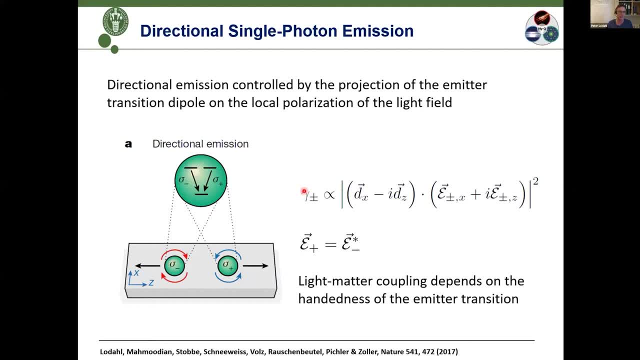 absolute square of that. that would be the decay rate at which this quantum emitter, quantum dot, an atom, your favorite emitter- emits light into a photonic waveguide, for instance, as illustrated here. so d dot, e, and, and now we have the setting. now we let's look at a planar setting, where I'll 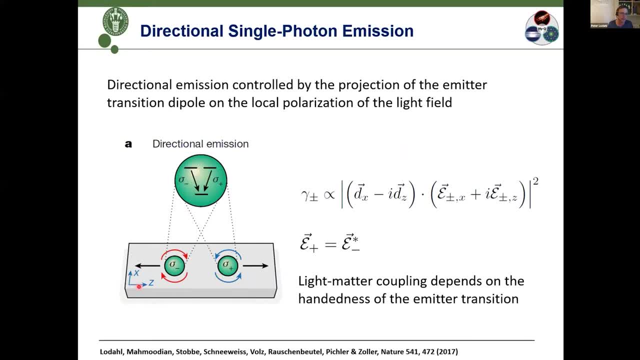 have a dipole moment, transition dipole moment in the plane in the x set direction. set is a propagation direction, just like before and, and, and in these structures. now the new thing is we have this longitudinal electric field component. I have not just a transverse component in the 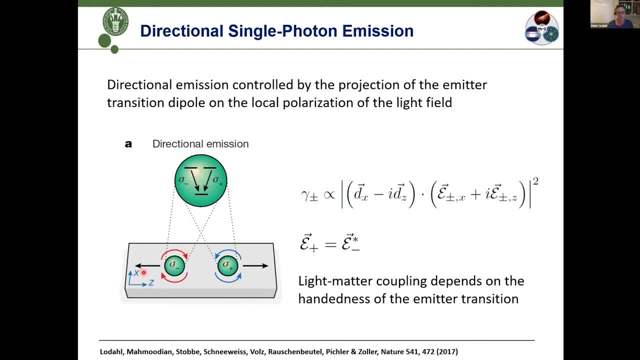 x direction. I also have a longitudinal component along the propagation direction here and I can ask myself if I take an emitter with a transition dipole moment. in the general case it would be a complex dipole moment. a circular polarized transition would be well, d d minus id you have just written. 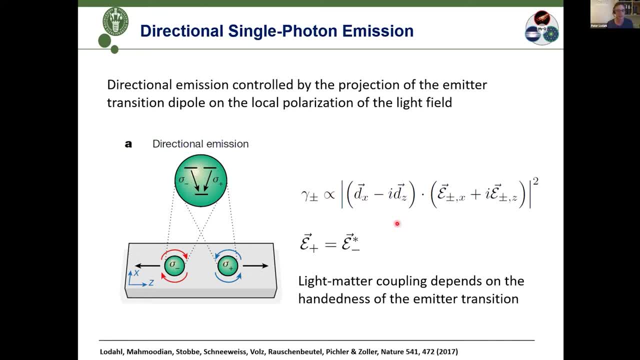 it as a very general case of any polarized emitter, and I can say: what's the probability for this to decay? well, that would be d dot e. what's the rate at which it's decayed? that's d dot e, absolute square. and now you can see, in these nanostructures we can 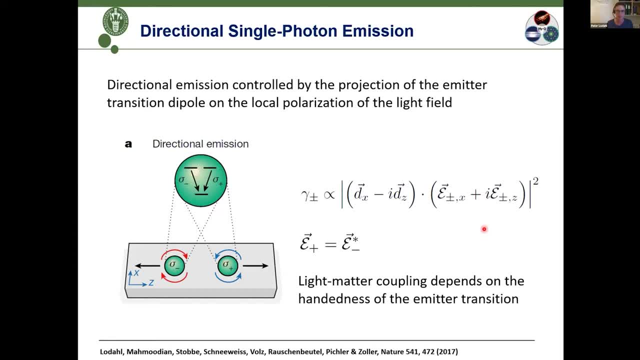 start to engineer this longitudinal field component. I'll introduce the nanostructure just in a second, but imagine that I can now totally engineer the local field and I think you can imagine that for for a certain dipole that I pick, a certain atom I pick, I put into the. 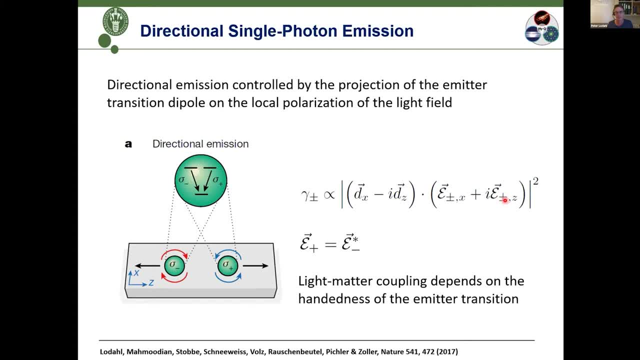 nanostructure. I could engineer the electric field and the longitudinal component in particular, so that this inner product between d and e is optimum. d dot e is as large as it gets, the electric field is matching the transition dipole and I can say that I can now totally engineer the local field. 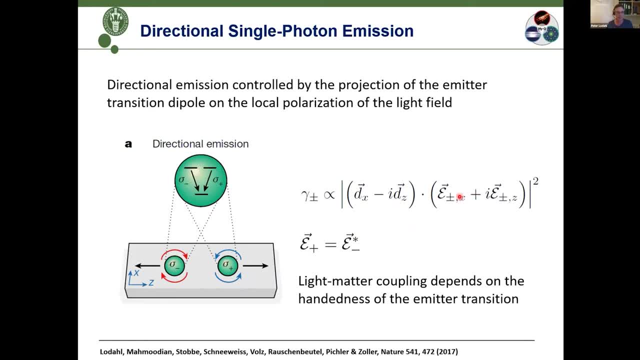 moment in the structure. So d dot e would be large, say for a certain direction. so let's say for the plus direction moving in the plus direction. But then due to reciprocity that I introduced before, if e in going in the plus direction is a complex conjugate going in the minus direction, 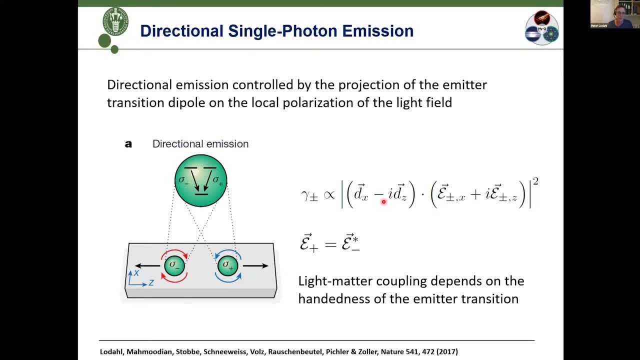 so you see, if I've engineered the electric field to be optimally oriented, with a circular, in-plane polarized emitter for a forward direction, d dot e would be large. then d dot e would be, could be, could be zero in going in the opposite direction. because, simply because of the 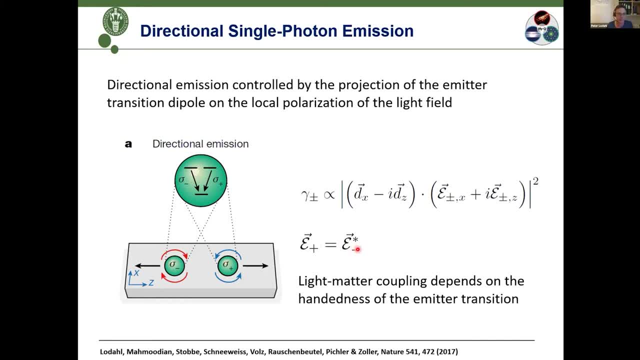 complex conjugation that I have here And that's a fundamental principle behind this directional photon emission. I could have d dot e for a sigma minus polarized transition, transition being very large, so that it wants to emit photons to the left here but it would not emit to the right. 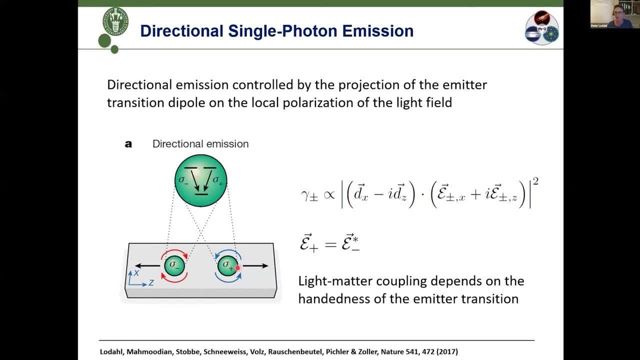 And reciprocity. if I take sigma plus polarized transition- I complex conjugate d here- then that would emit to the right and not to the left. So that's what we call chiral light matter interaction, That's chiral photon emission. 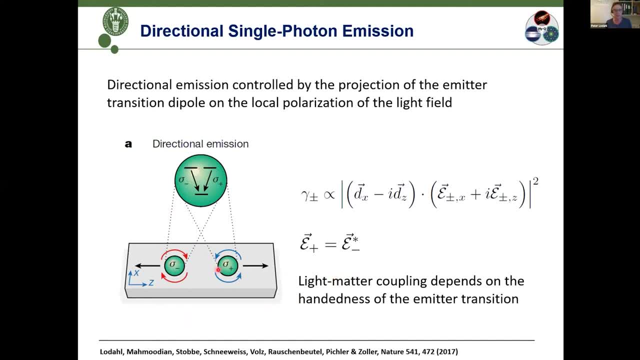 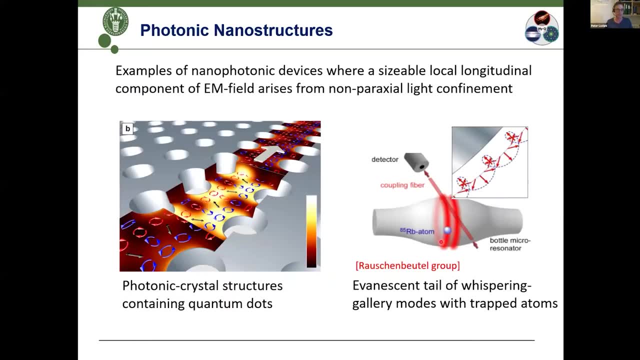 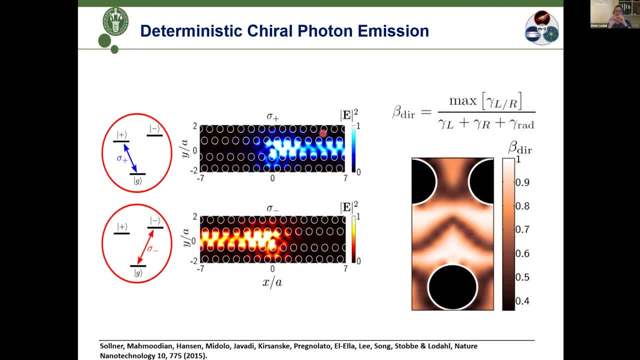 So let me introduce some of the nanomaterials here. So let me introduce some of the nanomaterials here. membrane actually means that, that that the cone of of k vectors you can couple to because of total internal reflection at the interface it's a very small cone, so there's not so much leakage. 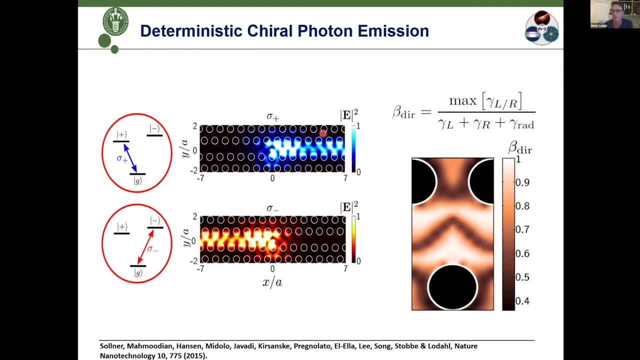 that's not so many k vectors to actually lead to. then there's another trick you can play in photonic crystals, that is, you can actually enhance the coupling to the waveguide mode. and that's exactly what you do in these photonic crystal waveguide structures. so here you see, the 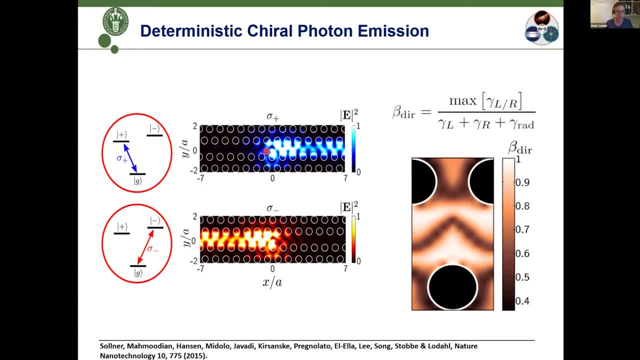 the, the glide plane waveguides. so you see, we have broken the mirror symmetry and and we are asking. so this is just theory, we are calculating how efficiently does a circular polarized sigma plus polarized emitter emitter to the right in this direction as opposed to going to the left? 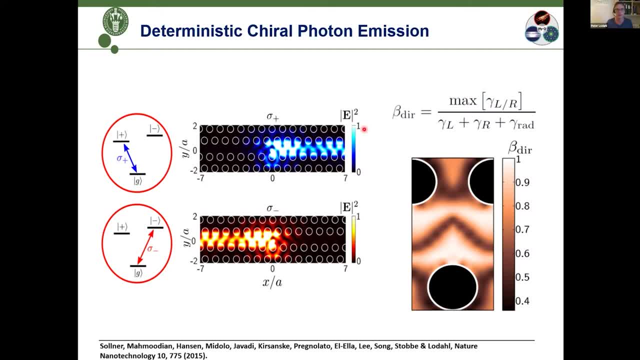 and as opposed to going leaking to any other mode. so that's what the beta factor tells you. so that's a leakage, that's a coupling to your preferred direction, as opposed to leaking to any other mode. and you see a calculation of this directional beta factor. this is within the unit cell of the glide plane for tonic crystal waveguide, so it's a spatial. 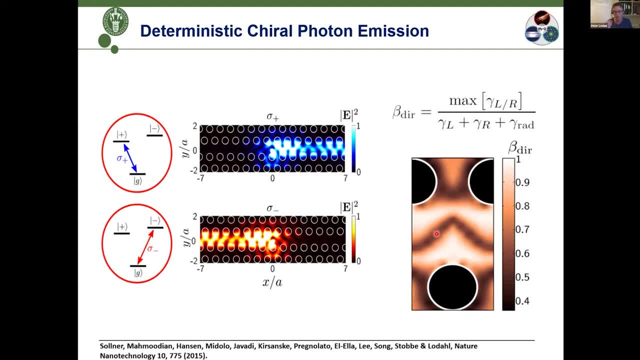 map of that and and you see so everything, as i pointed out, varies spatially, but the glide plane waveguide structures are engineered in order to have a preference for this circular polarization over large spatial areas, and that's why you're seeing that, that the beta factor here is high. 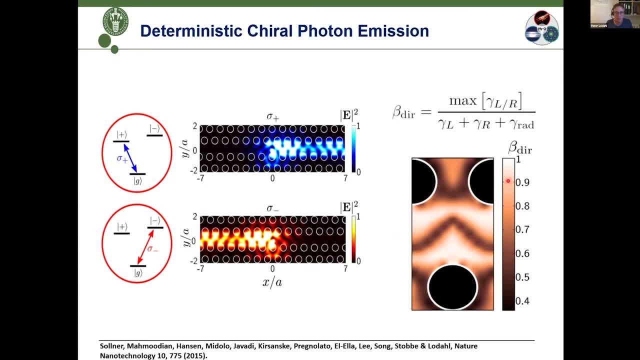 i mean the the numbers are. they'll be many areas here where you are. you are in the high 90s of this directional beta factor and the highest point here would be 98, so that that really means that that only in two percent of the cases you lose a photon to coupling vertically out of structure. why did? why does? 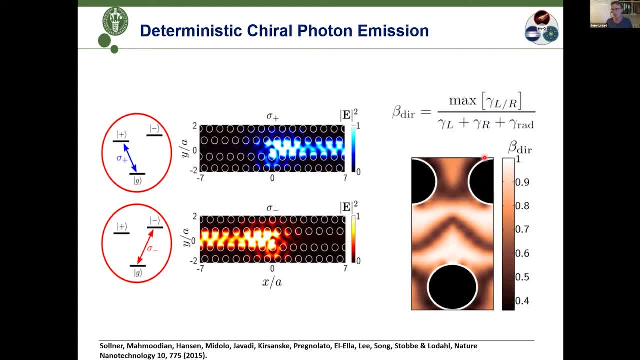 it work so well? well, because this membrane leakage that i mentioned, uh just before. but another point as well is that we can do purcell enhancement. uh, we can exploit purcell enhancement, which is enhanced coupling into the waveguide mode, meaning that you know, i'm suppressing this coupling to radiation mode. 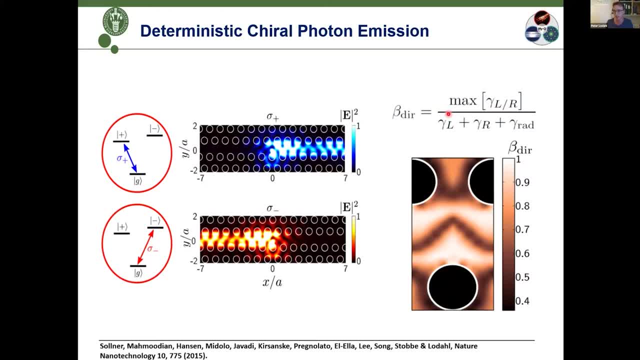 but i'm also enhancing the coupling to the mode that i'm interested in, to the lift going mode, for instance, or to the right going mode, whatever direction mode i'm interested in. i'm enhancing this as well as suppressing that, and that's a way to get beta to go very high. how do i enhance this? 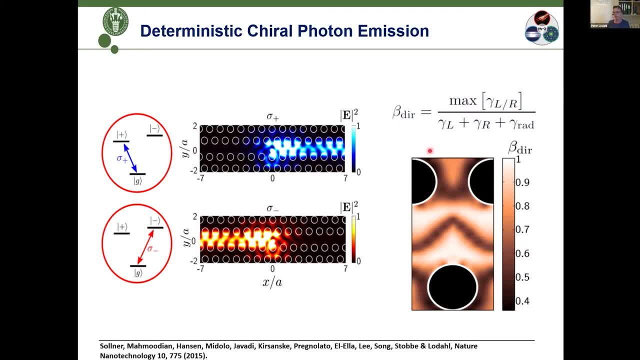 well, that's called the purcell effect and many of you have heard about the cell effect in cavities. if i put an quantum emitter into a cavity then it decays faster and there's a purcell factor that is proportional to q over v. so if i have a high q factor on a small mode volume cavity then this: 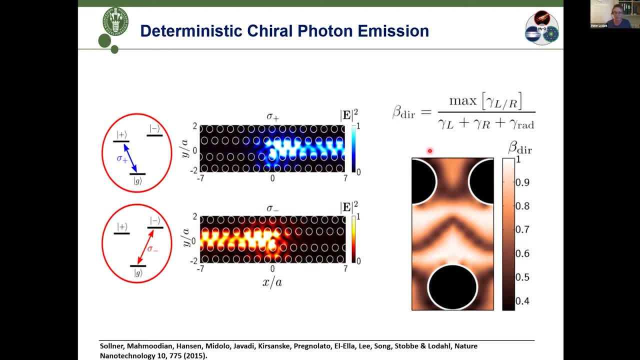 purcell speed up goes faster and faster. the quantum emitter likes to emit a photon into a mode that that that that is small and has a high q factor. the local density of states is enhanced for this mode and that enhances the spontaneous emissions. spontaneous emission is not just the property of the emitter, it's also the property of the environment. in the waveguide we 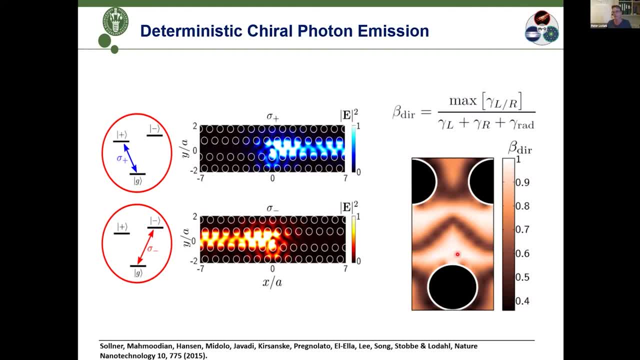 have a similar effect, but in this case it's not a q factor, because there's no mode being resonated here. there's a mode, a propagating mode you're coupling to and this propagating mode has properties like, and one important property is: is the group velocity of that mode? and it turns out: 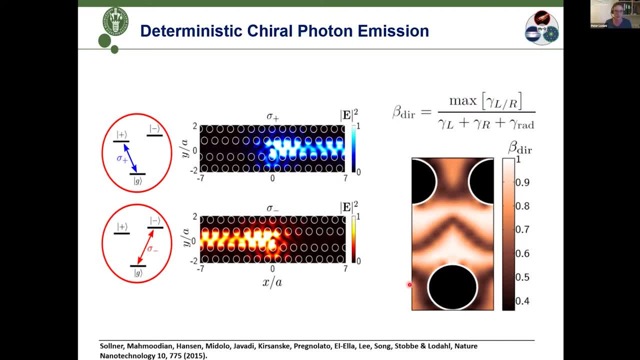 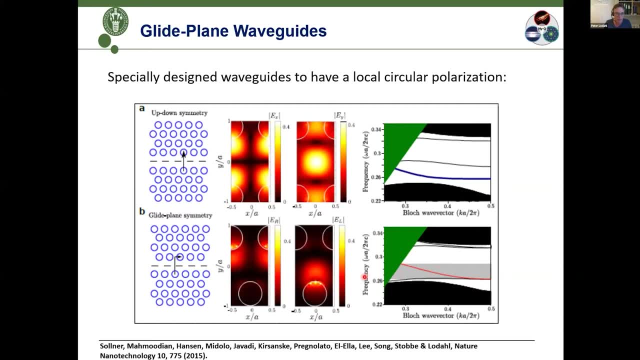 so the group velocity is d, omega decay. so if i'm going back to my description here, you can see that this is the waveguide mode that we're interested in. this is omega as a function of k, and you see that that that that we have engineered the dispersion of this light. 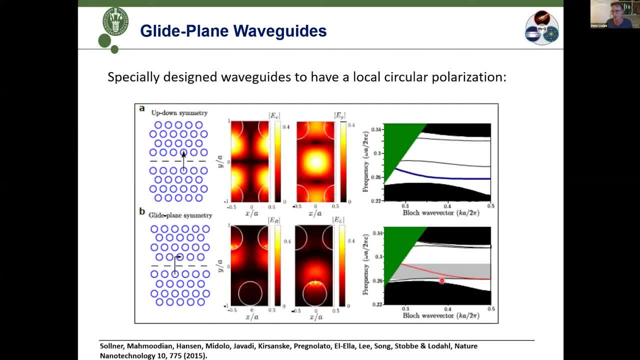 omega doesn't depend linearly on k in these photonic crystals like it would in in free space. you have a non-linear dependence of omega on k. that means the omega decay is actually, so the group velocity is lower than than you would have in free space, so you're slowing down light in the 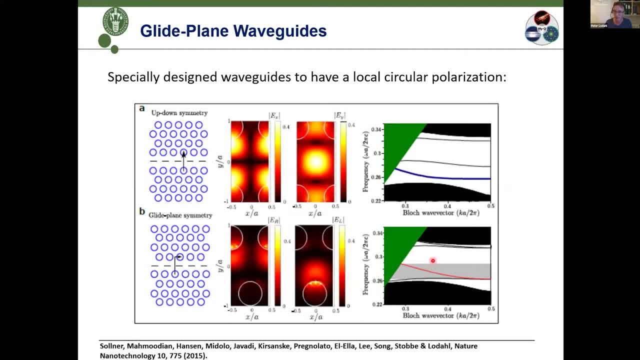 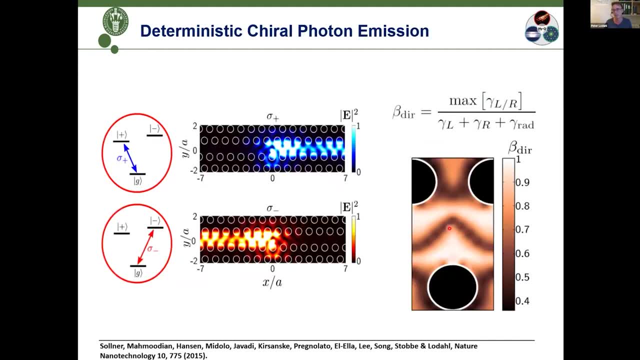 these photonic crystal waveguides. if you're slowing down the light you're enhancing the density of stage and you get a purcell enhancement from slow light. so you can say the quantum dot likes to emit it for its photon into a slowly propagating mode because its density of state. 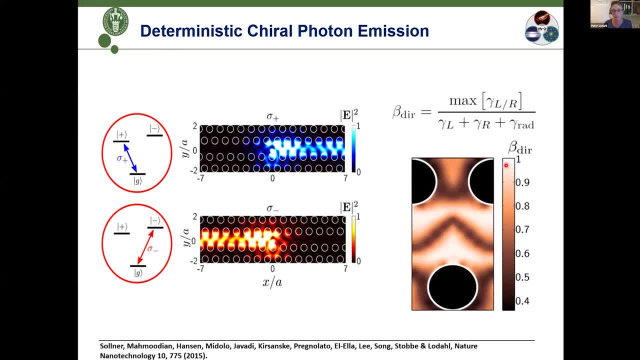 state is higher. so that's a purcell enhancement in a, in a photonic crystal waveguide, in a wave guide geometry, which is generalization of the purcell enhancement you will have in cavities. so that's a trick we are playing to. that was a long answer to a very good question. 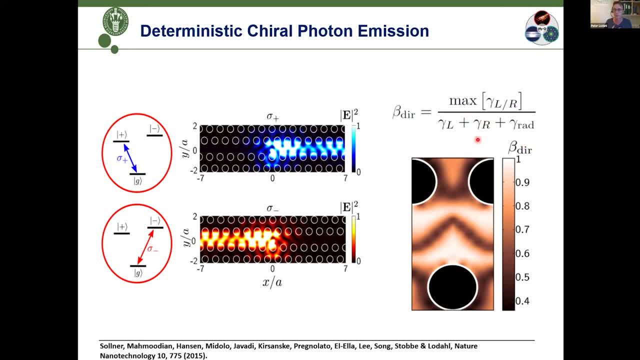 so to avoid leakage, we're enhancing the coupling into the waveguide mode. by this slow light enhanced induced purcell enhancement, we are suppressing the leakage to all the other other modes. that's what the photonic band gap does and that's what the these membrane structures do. 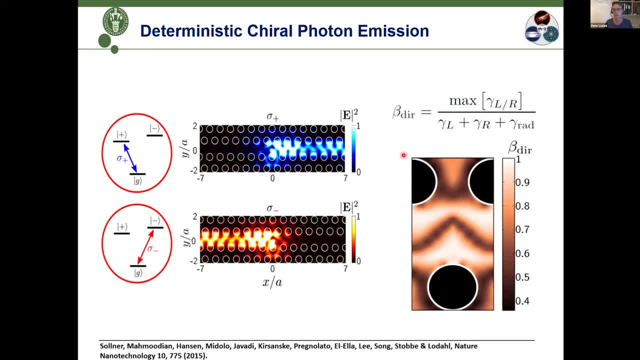 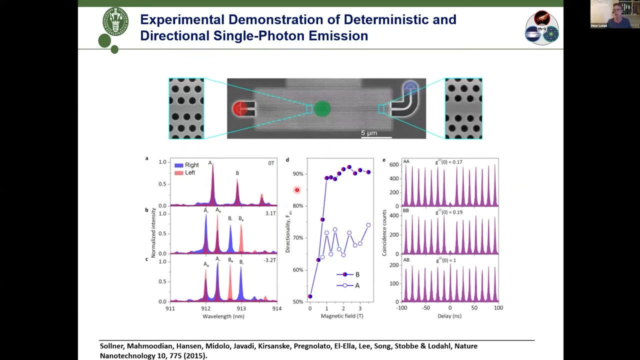 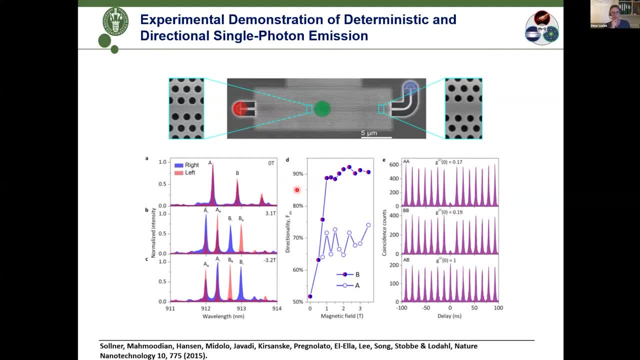 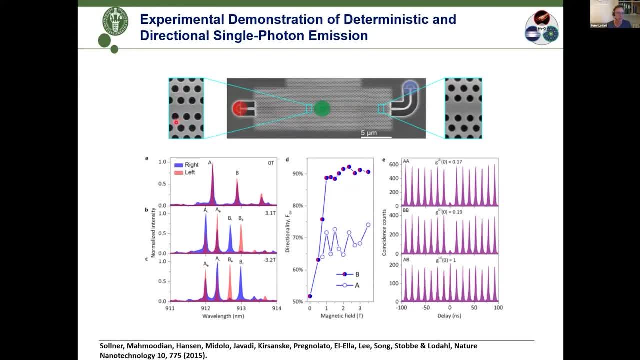 part of the device. so so if you look at zooming in, you'll see that the this mirror symmetry is broken here, close to the center, and then, when you go further and further out to the side of the device, we're gradually changing the hole, so we're going back to regular photonic crystal. 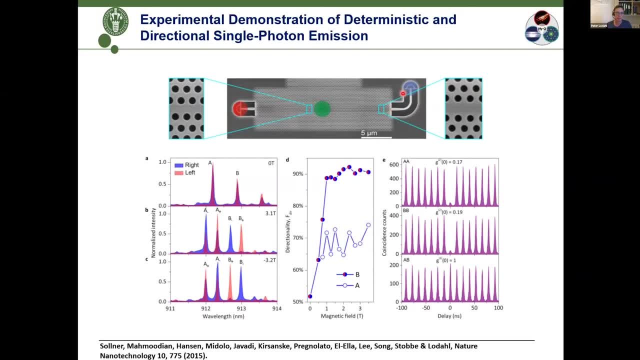 symmetry, because these block modes we can better couple out to to regular waveguides and now to these grading couplers that i that i talked about. so this is really showing some of the engineering again you can do in these structures that you can, you can design, uh, the, the, the. 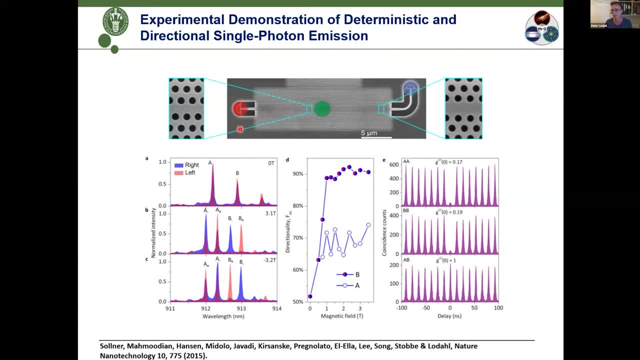 the waveguide and the properties of the waveguide the way that you would like. so how do we show the directionality? in this case, we identifying single quantum dot lines a and b here in particular, and we are then simply looking here to the left and to the right on the 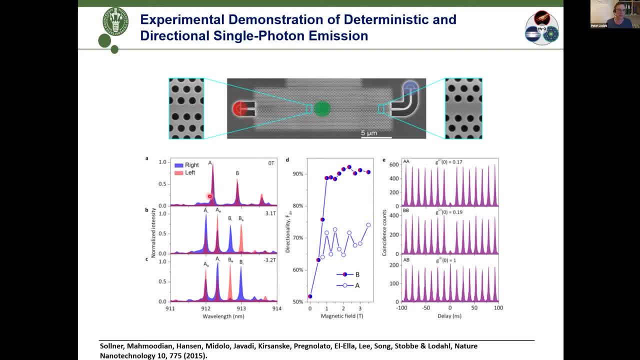 those two gradings here, whether a quantum dot emits to the left or to the right. and you see, here, in this case, where we are not applying any magnetic field to the system, we are collecting from quantum dot a line, we are collecting photons both on the rate grading and and on the blue grading, so it's emitting. 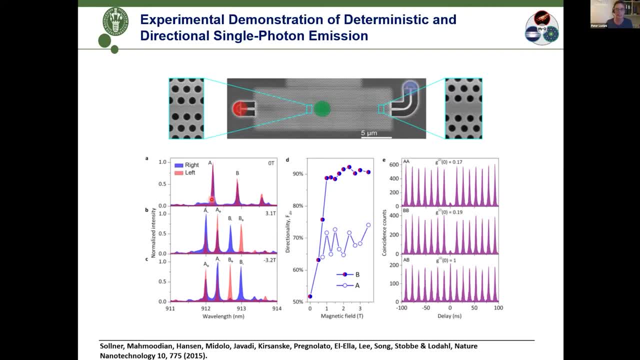 uh, half the time one direction, half the time the other direction. in this case it's a linear dipole transition. so there's that, there's nothing? um, uh, it has to. you have to a circular polarized transition to, to, to, to get this directionality. and this is exactly what we see when we are starting. 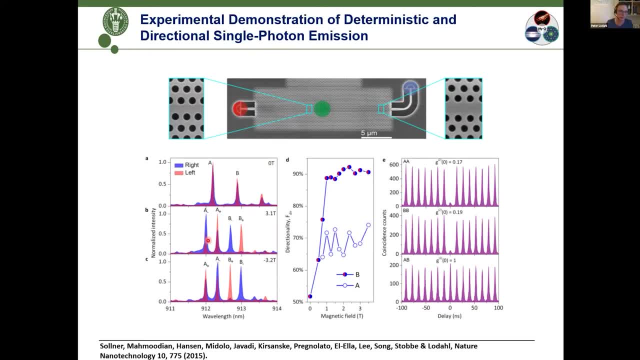 to apply magnetic field in the in the growth direction of the quantum dot. you split the lines. one of the lines would be a sigma minus transition, another one would be a sigma plus and you see for instance here the sigma plus image almost exclusively to the red grading here. 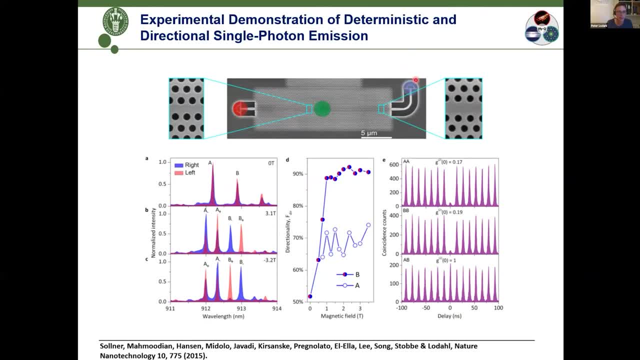 and the blue. that's a little bit of grass here, so it hardly collect any photons on the blue grading and vice versa for the sigma minus transition. and then, just as an experiment check, you're flipping the polarity, you're you're instead of having the magnetic field in the plus direction, you. 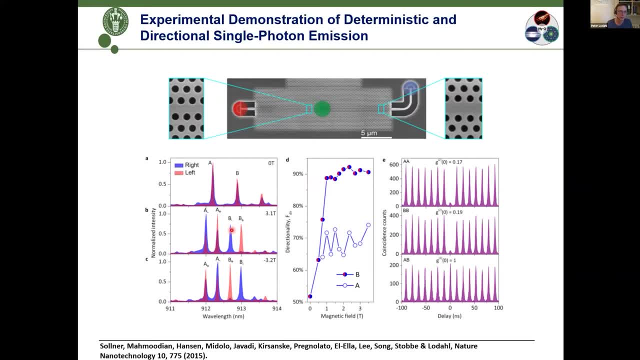 put it in the minus direction, that flips the polarity so that minus becomes plus, sigma minus, sigma plus, and indeed we then also see that this also, and i mean the sigma plus, wants to emit on the red grading and not in the blue. you can, of course, in extract this directionality and quantify. 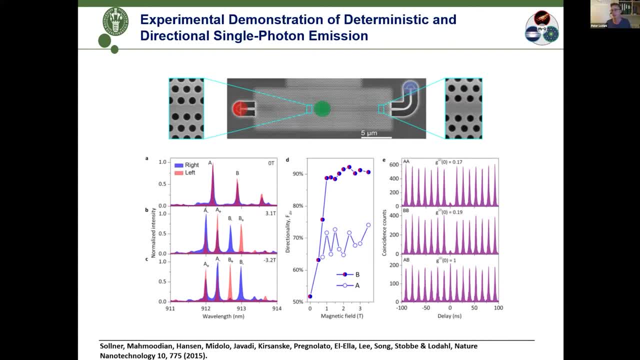 it as what is done here and and also prove that this is really single photon emission. so these are single quantum lines emitting single photons. you do this in optics, what is called a hamburg brown twist experiment. you take the light on the beam splitter 50- 50. 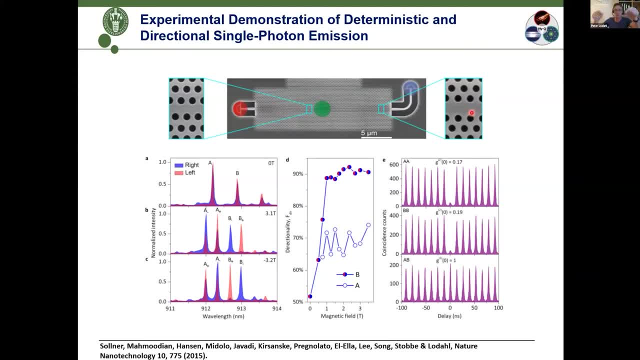 please, please, send it out to two detectors and you do coincidentally detection between those two detectors, to see how often do I detect a photon in each detector at the same time. If it never happens, then that was a single photon source. this was a single photon. 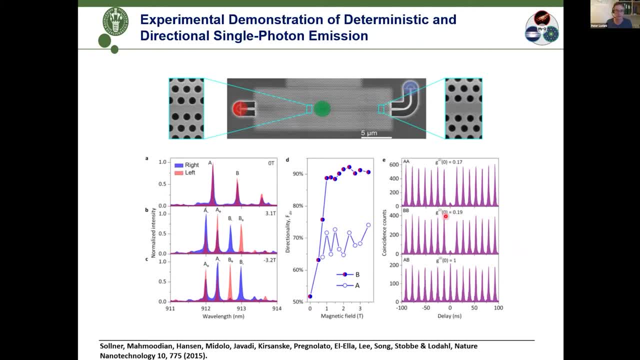 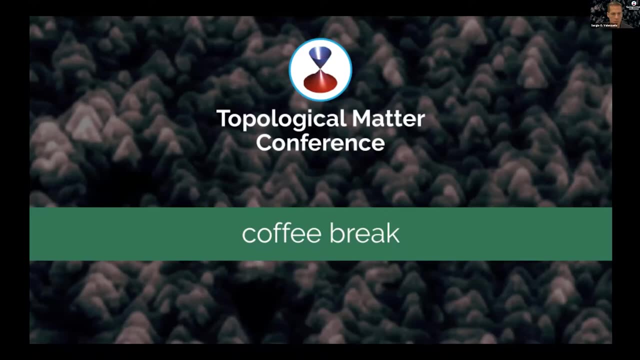 pulse that we have generated and, of course, nothing is perfect in real experiments. So here you see a little bit of multi-photon contribution in these experiments. Good, so I think we'll take a break here. You will need to share your screen again, Peter, once you start And there is a question. 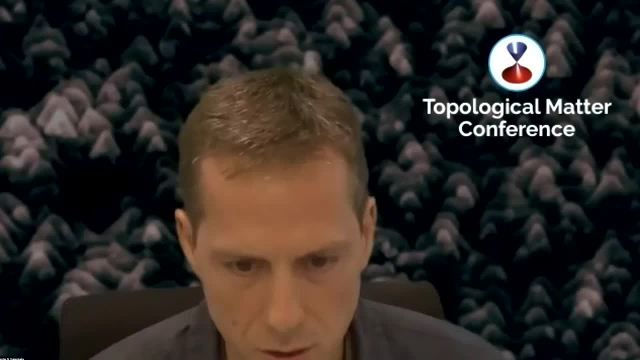 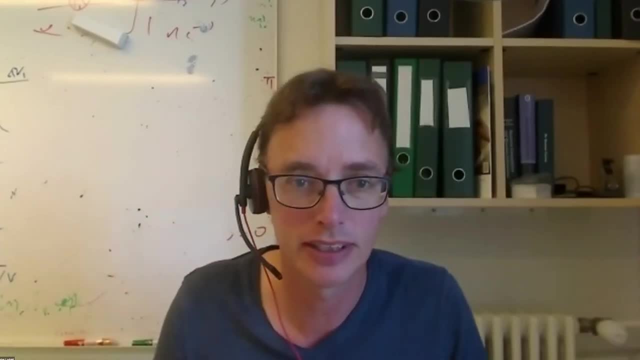 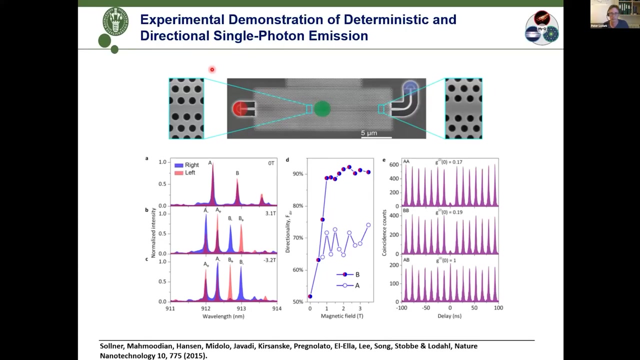 by Ramesh. both in the chat, In the Q&A, you can find it. Yes, I see it. thanks, I need to share my screen again. Okay, I think we start again, so you can still hear me. So there's a question from Ramesh. 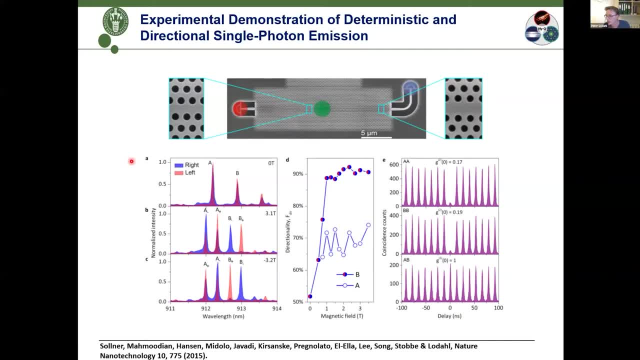 Jamanka. He's asking: why is the intensity at A and B different without the magnetic field? And referring to the experiment that we had here? this is a very good question. Indeed, if you look carefully at these plots here, you'll see that, well, the red and the blue curves here are not. 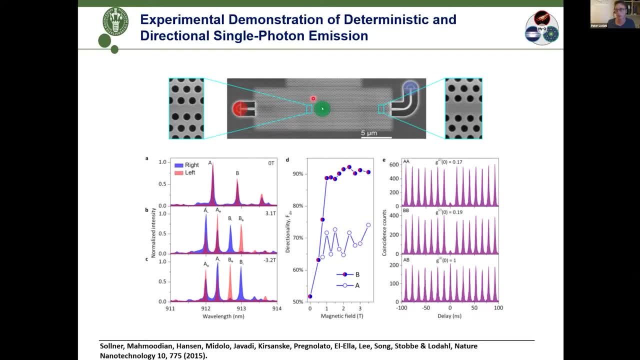 exactly the same height. So if you look carefully at these plots here, you'll see that well, the red and the blue curves here are not exactly the same height And that really has to do with asymmetries in the experiment. So you'll see that there is some. 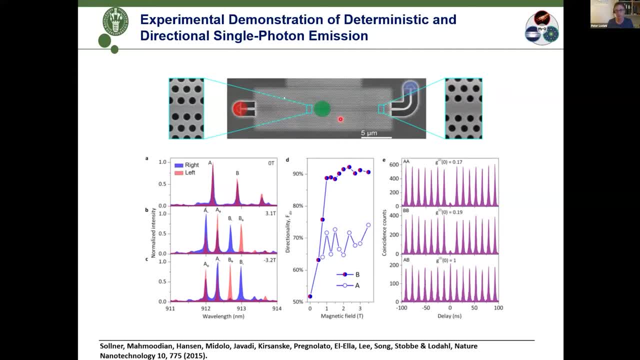 the photons are propagating out of the region and into the grating And there will be some slightly different propagation lengths And I think most importantly also is that there will can be a little bit different coupling out of the grating and into the actual microscope objective. 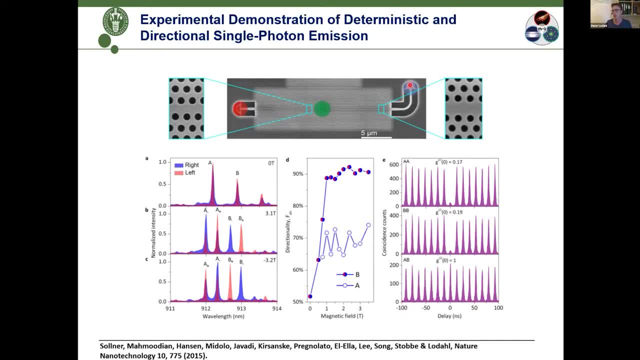 that we are using for the measurement. So that will give some asymmetry in the data. So this is a very good point. So that's uncertainty in here. But then when we are applying the magnetic field we are seeing very pronounced change in this overall intensity. 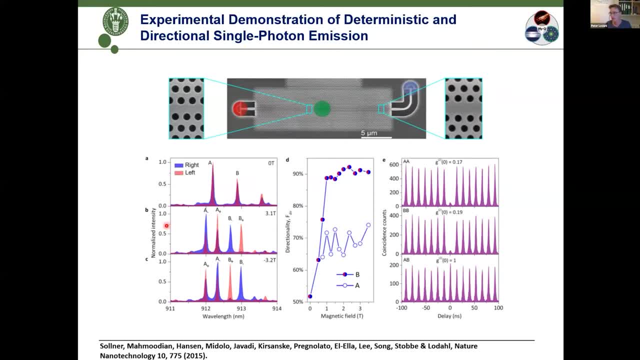 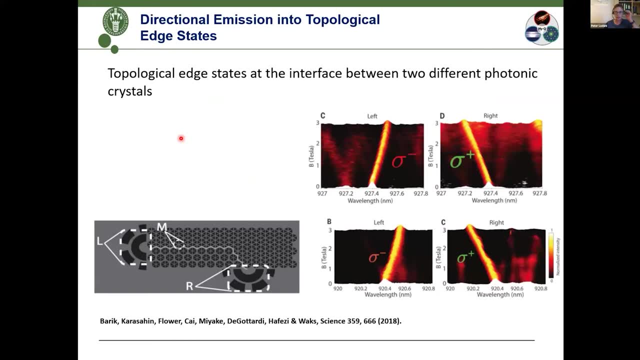 while not changing any parameters, Thank you. So let's return here to slides. This slide helps. Yes, so I'm missing something here. I think That's something missing from the slide. But that's it, I think it's all right. 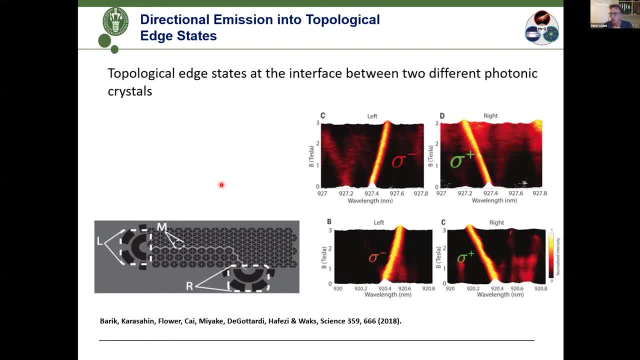 So topology, So there's also topological photonics, There are opportunities of. so far I spoke about light plane waveguides, So although there's nothing that is topologically non-trivial in these systems, but there's an opportunity also to make 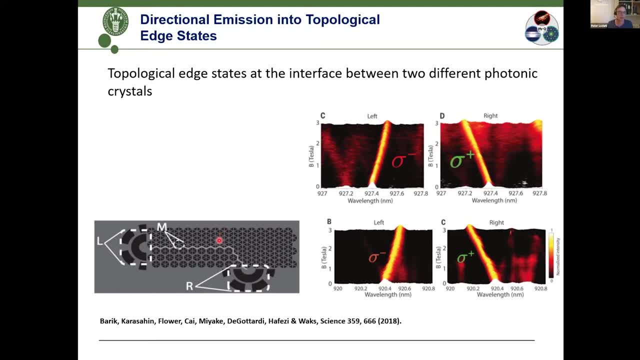 structures, photonic waveguide structures, where you are combining, interfacing, two photonic crystal sections that have different topological properties. So that would be. there's an example in the literature from Edouard and Mohamed Hafizi where they're taking two lattices. 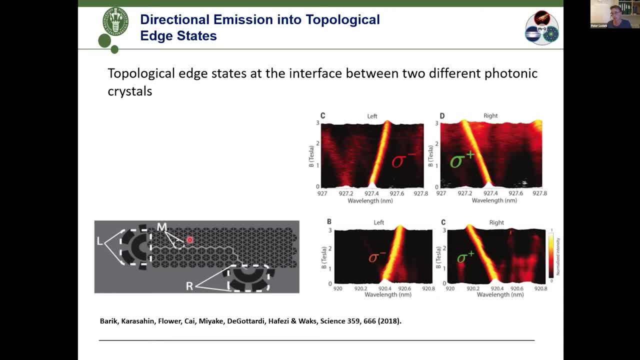 and there's a turn number associated with each of these photonic lattices And you're combining those two that have two different turn numbers And at the interface between those two lattices you can start to have waveguide modes as well, Just like in what I've spoken about before. 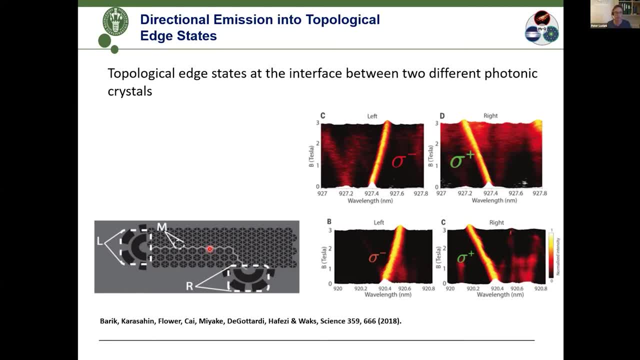 I mean we are deliberately leaving out a row of holes and that was our waveguide mode. Here it is the edge mode featuring that shows up in between the regions of those two waveguides with different topological sections, photonic crystal sections with different topological 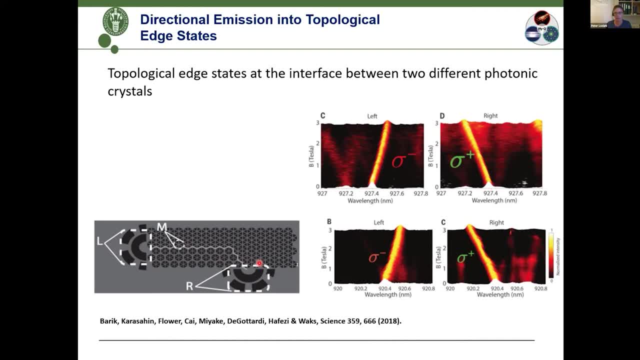 properties, And this is really an interesting area where the same physics that I've been spoken about so far, I mean this directional emission, also shows up, And this first experiment proved that this is an experiment just like what I showed before. You're applying a magnetic field. 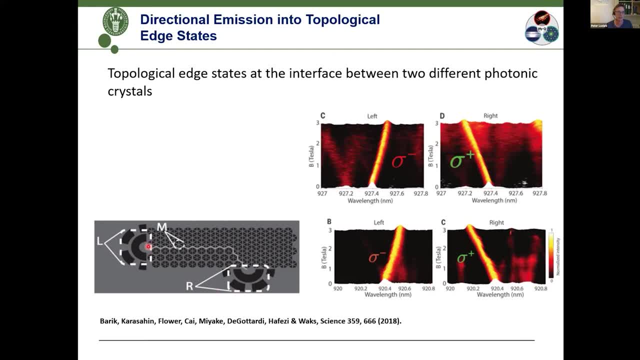 and you're having a sigma plus and sigma minus transitions and you're collecting photons from different gradients here And you're seeing that sigma minus goes to one gradient to the left and sigma plus goes to the other gradient, And then they can also make bends. 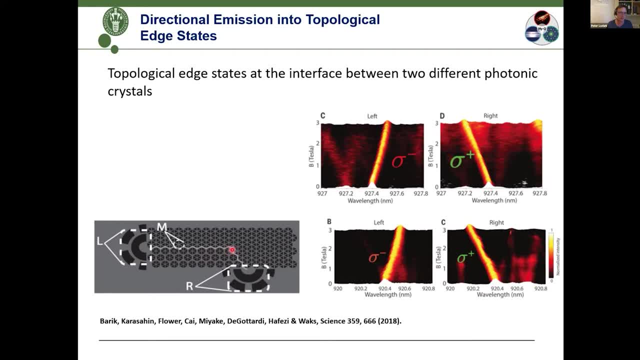 in these structures, as you see here. So if you're starting to, if you're introducing a structure like that where you are extending this photonic crystal section- and I think I should shut this down- You're extending this photonic section. here You can actually have a waveguide bend, a 60 degree waveguide bend. 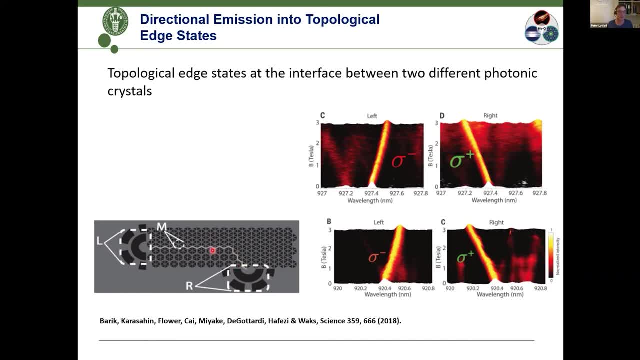 like that, but they also showed explicitly that it works, and I think there are really some interesting questions about what are the photon transport properties of these topological systems here, and could it even could it be that there would be some advantages in terms of these backscattering links and processes that I was briefly mentioning before, maybe these topological way that would be better. now there's a question: which symmetries? 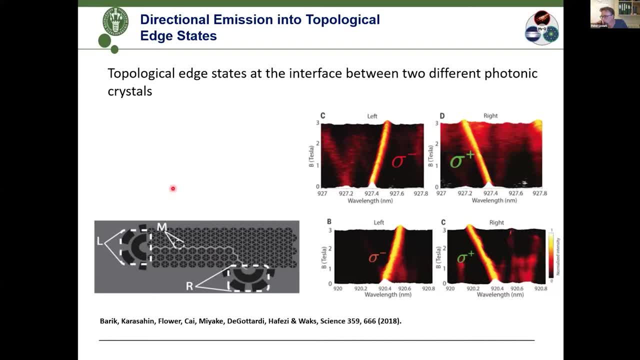 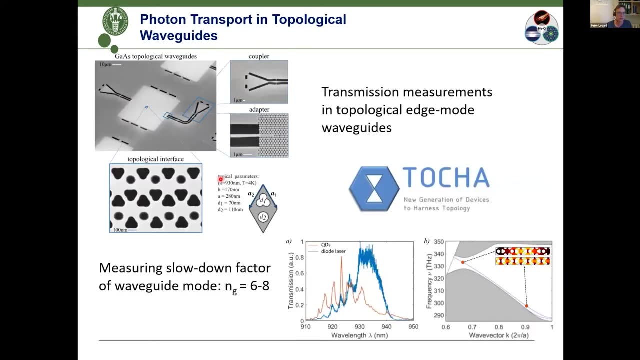 are broken in the photonic crystals, so maybe I will show it on the next slide so you can see more precisely what, what, what, the way guys look like, and so this is what we are doing in this direction: within torture, the project that's a curious is leading and that. 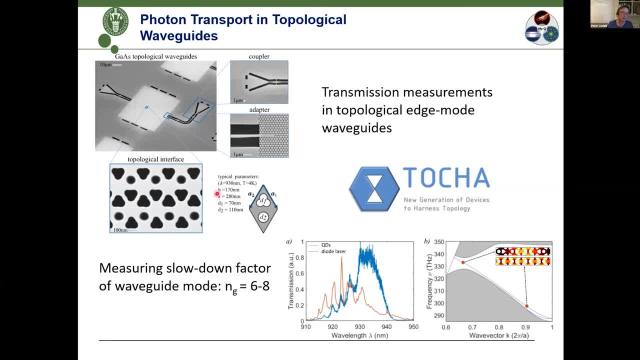 he introduced In the beginning. Now we are starting to make these kind of topological interface structures And you see here, really close up of the of the, of the structures that we are. we are making So here, you see, you see really the unit cell, and and and and he has one for turning. 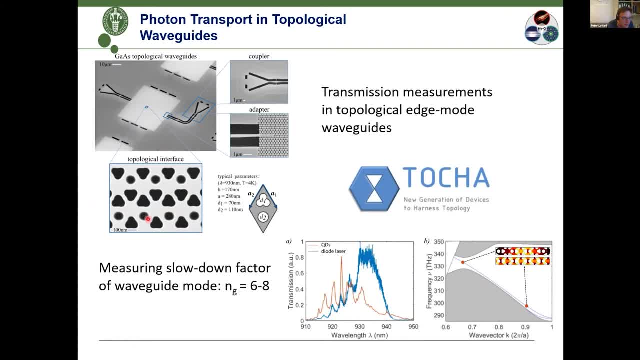 crystal up here and he has the other for turning crystal down here. and you see we have translated by half a lattice constant, so making this glide plane wave guide trick as well. And then we have mirrored also the unit cell. So that's a two operations that are being done on a on a unit cell. 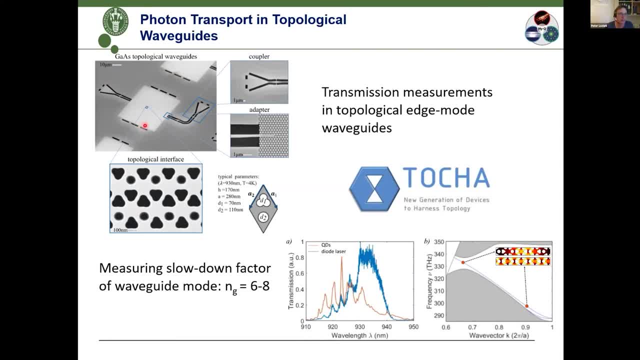 And and you see these structures like you saw before, that would be such a. now it's a topological interface where the photons are guided in this region. it doesn't just look in the image. you wouldn't think that photons would be transporting there. that's really. 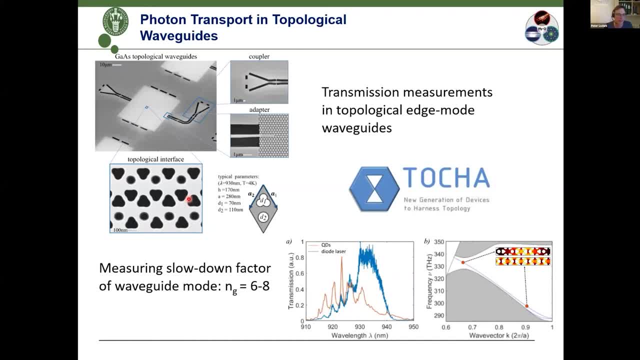 not Not a wave guide like like what we had previously, but but there are two for turning crystals with that that have different churn numbers and and at the edge of those two structures you can get a photon transport, just like in the in the wave guide structures that. 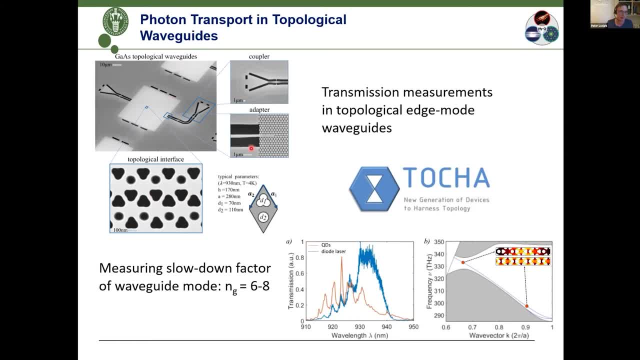 that I introduced before, And you see, we make again these advanced devices where you are. okay, then then there's a question about what is a mode of this? Okay, then there's a question about what is a mode of this? Okay, then there's a question about what is a mode of this. 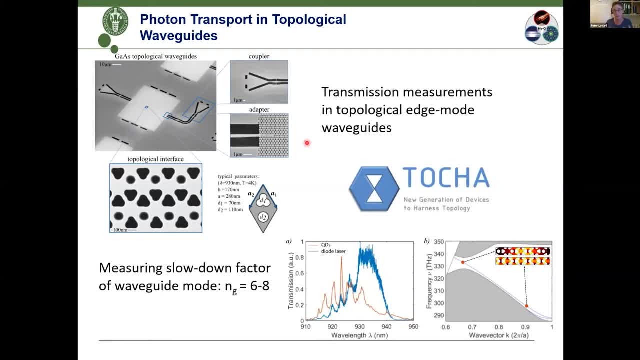 Okay, then there's a question about what is a mode of this At this topological, at this interface? you, How does this both look like? this can really be a. you can calculate them and you see some images here. let's not go into to all the 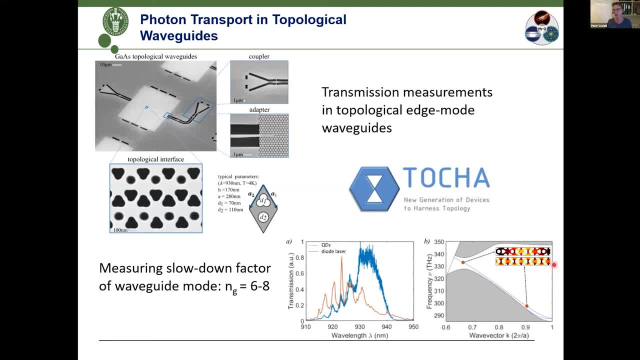 details about this. but it can be quite a complex mode because you're really starting to to to do quite advanced engineering of your, of your unit cell, of your for tonic latches, You wish. So can I cover this mode out and and can I cover it out to these ratings and eventually, 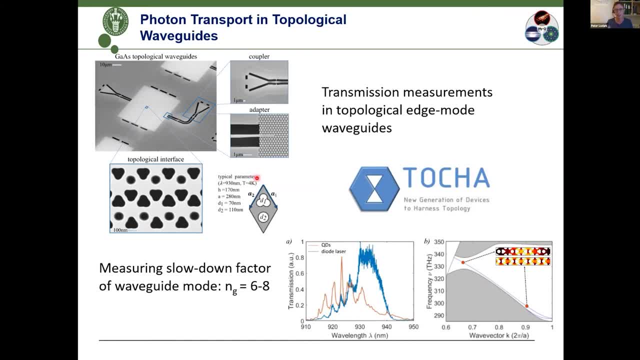 want to get photons out of that specifically. kill my horsepower here And if you have, if you called me, I could cut it, because you can cut it if you want to- from- and there's a lot of engineering going into that that you are starting to. 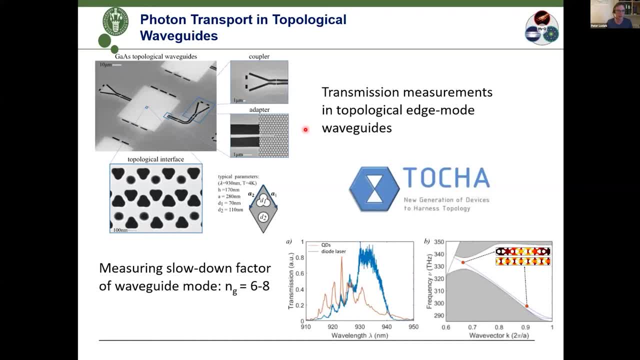 adiabatically transform these modes, these defect modes of these modes, between the two photonic crystals, photonic sections, and you're gradually changing this mode into something that you can couple into a nanobeam waveguide and eventually couple out with with a grading. so 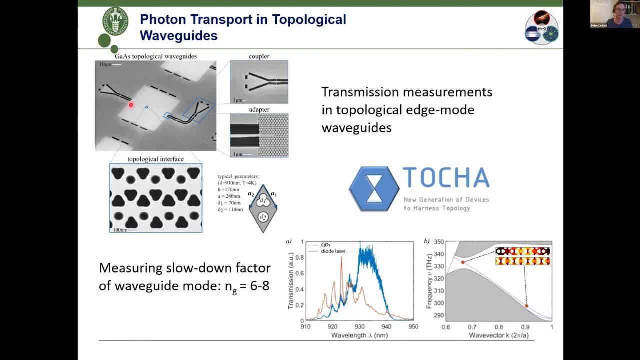 that's really mode engineering, adiabatic mode engineering- that works surprisingly well actually, that you can do it with quite some quite high efficiency- and this is all stuff we are working on at the moment- and and, but it looks surprisingly efficient actually in this particular experiment. 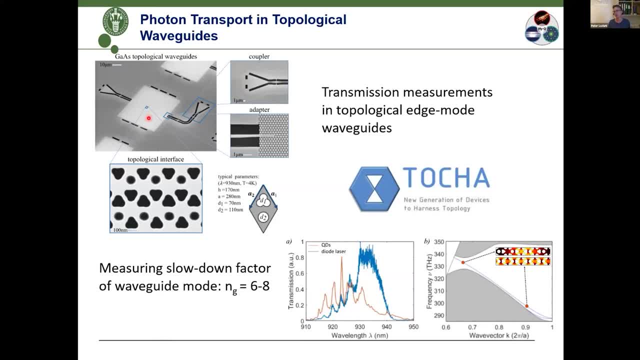 we have been after also this: how much slow light can i then ultimately achieve in these structures? and a way of measuring slow light is actually that you are you, that's, that you can have residual reflection at these interfaces, so that the reflection that says you have a weak cavity formed actually between the two output gradients, and you can use that. 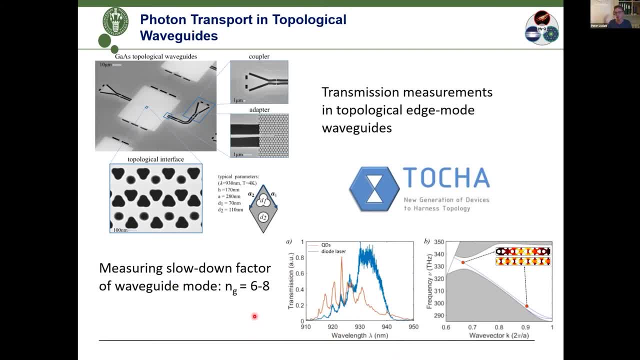 Fabry-Perot fringes to extract the group index. so the slow down factor of the of the photons transported in this, these advanced photonic waveguides, and those are the numbers that we're achieving at the moment. I mean slowdowns factors between six and eight, which enhances the light. 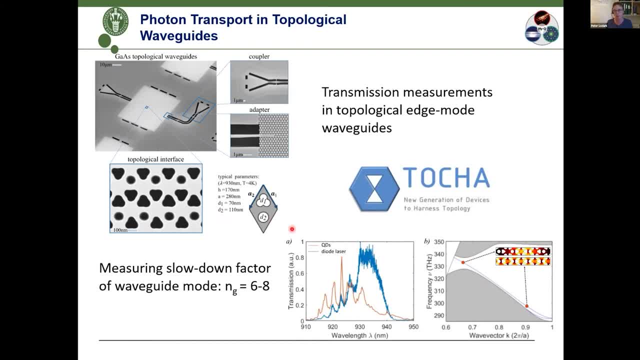 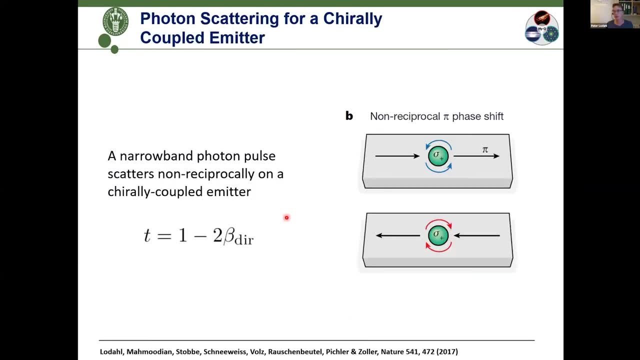 matter coupling into the waveguide, as I mentioned before, by the Purcell enhancement, okay so. so that was a lot about photon emission, directional photon emission in engineered photonic crystal based waveguides. so now we want to go one step further and and say, well, can I use that to do something else than just directional emission? that's good, but, but maybe 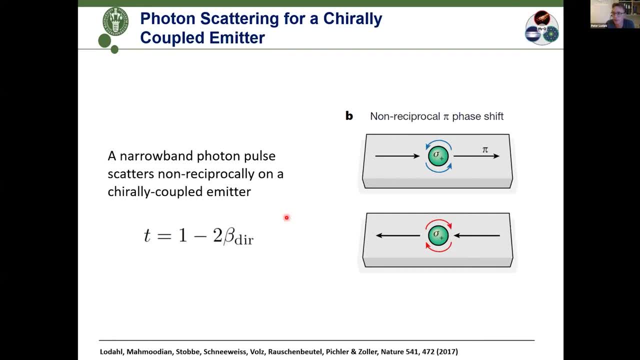 what else can I do? can I get photon transport to become directional so that that I can, you know, make non-reciprocal photonic devices where I send light in through one direction and and that does something else, and if I send it in from the other direction? can I break time reversal symmetry from? 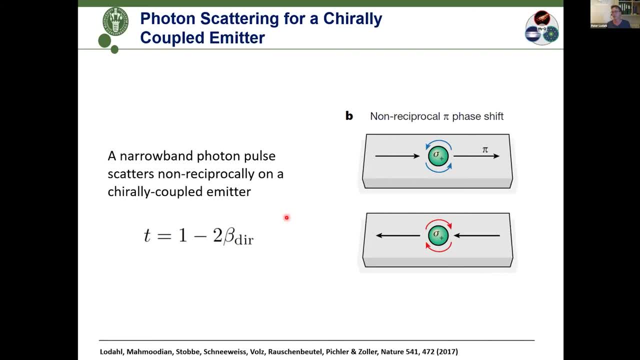 the point of view of light. well, the waveguide clearly doesn't do it right. I mean there is reciprocity in Maxwell's equation, so you have nothing like you know, if I send light at one direction in the way, but light cannot go through the other direction of the wave. but there 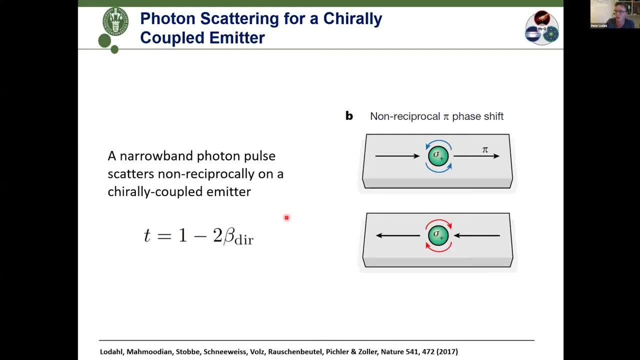 is light and then and then, and you know it just, you get a complex conjugation there that we spoke about in the beginning. the key is really the light matter interaction, because the light matter interaction is directional, de again that we spoke about at length. that is not just about how does 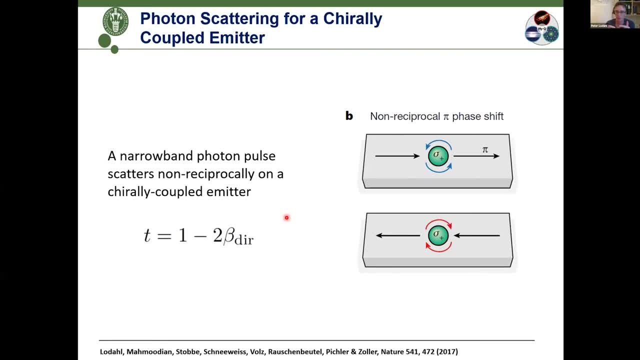 the emitter emit light, it's also about how. how does it emit a scatter light? so if I send in photons in the waveguide and have interaction with the emitter, that would be de that, that that determines this interaction and that will be directional. so there should be a difference if I'm going from left or going from. 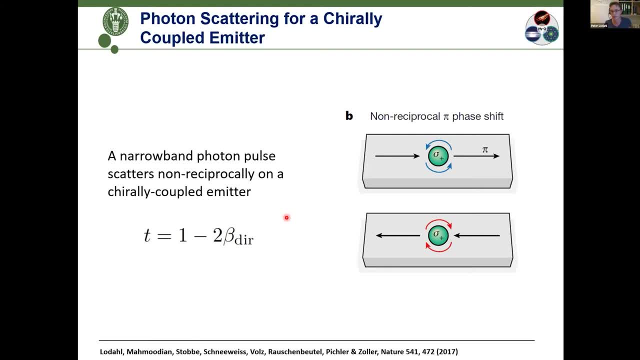 right, if I engineer de to be directional, and we we now know how to do that. I'll be speaking about quantum emitters, because that's that's that's what is close to my heart, but of course it doesn't have to be quantum, and so so I just have a coin, a single quantum dot and with a single 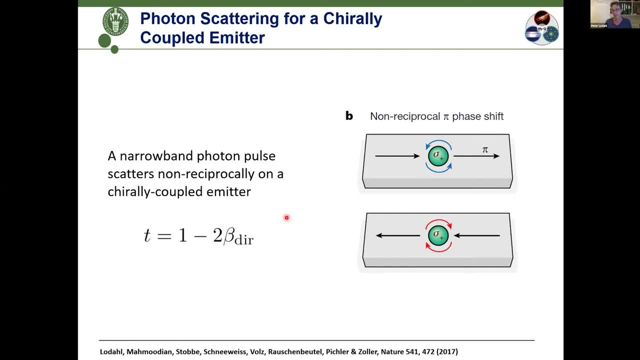 spin in there, but I could also have a polar, a classical polarizability, so that you could get this interaction to become directional. so it's a more general concept here than just for the for the quantum light matter interaction that I'll be speaking about. okay, so I already introduced it. 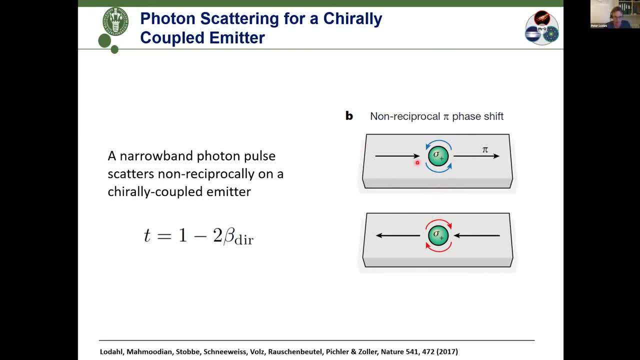 so now the idea is that that I have the emitter and I have it in the sigma plus polarized, a transition dipole. I sent light in from the right and de is set up so that this emitter can only emit to the right. that also means that that when I do scattering on on such a quantum emitter here, it 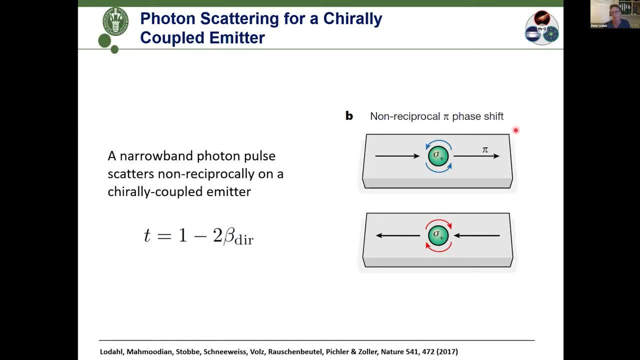 cannot scatter the photons off to the, to the left. it can only scatter in the forward direction, at least if the directional beta factor is perfect. of course, in reality it would be finite and there will be a little bit of probability of scattering backwards, but prominent dominating probability. 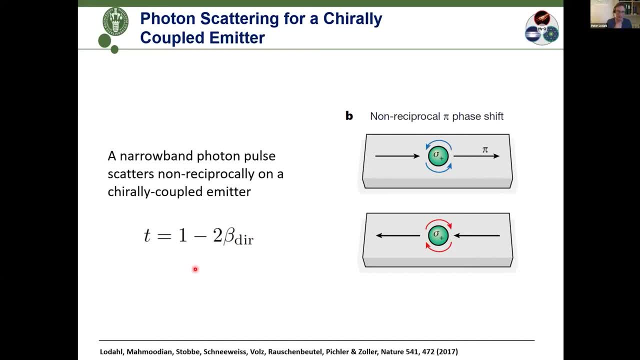 of scattering forward the transmission coefficient here. here it is: if I take a narrow band- classical field, laser field- but just attenuate it so much that on average only at max one photon interacts with the emitter at a time. narrow band, what does that mean? well, narrow band relative to. 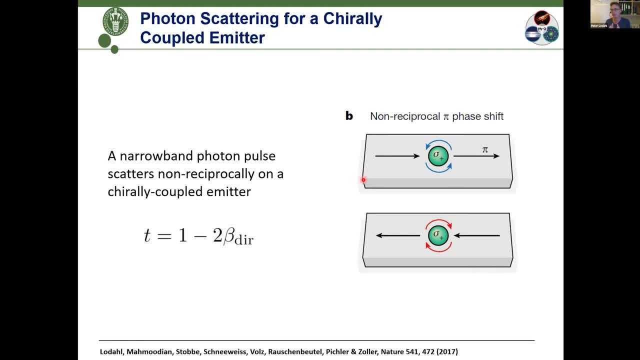 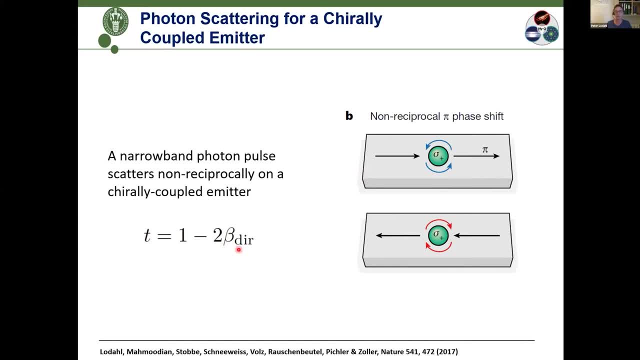 would be one divided by minus, sorry, one minus two times beta directional. beta directional could be close to unity, as we talked about already, 98 at least. so you see, if you put one into this equation, you'll get a minus one from that. and what does that mean? that means I get a. 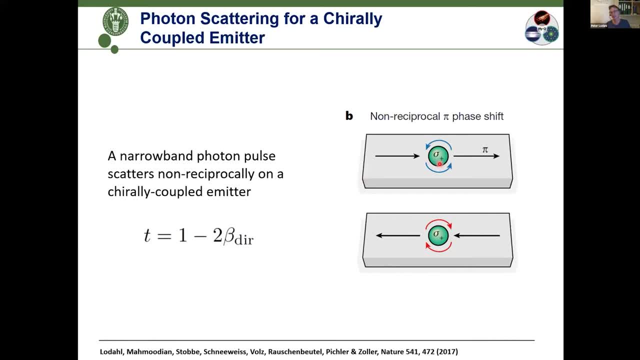 transmission coefficient in the that it scatters in the forward direction with a minus in front, so that means that the photon has expired, has acquired a pi phase shift in the in interaction. so that's what happens. to send the photon in beta directional is very, very high. so 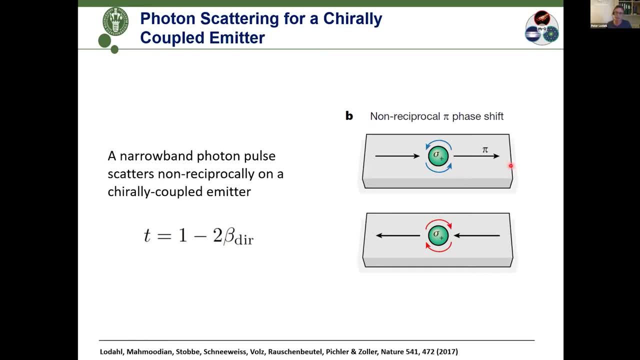 the photon scatters, it can only go forward. but in this scattering process it requires a pi phase shift. okay, now let's send the photon back again. d dot e was optimum for going forward. it comes from the wrong direction. d dot e would be zero. you're going in the backward direction, so it doesn't see. 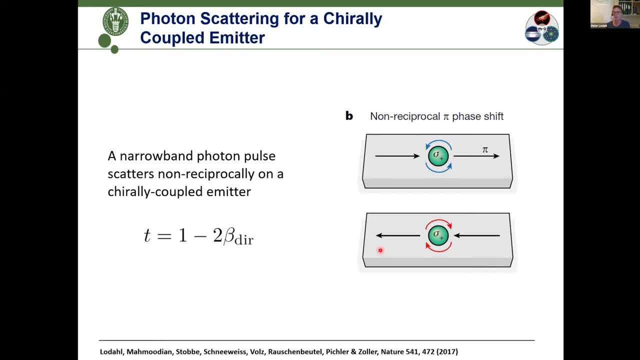 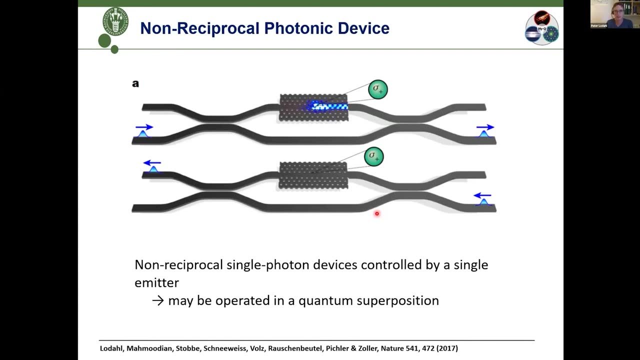 the emitter at all. d dot e is zero. no phase shift, no interaction with the emitter. so here you see, the difference between going forward and the difference between going backward: a pi phase shift. okay, so now I can make a non-reciprocal photonic device based on this. because how do I turn a phase? 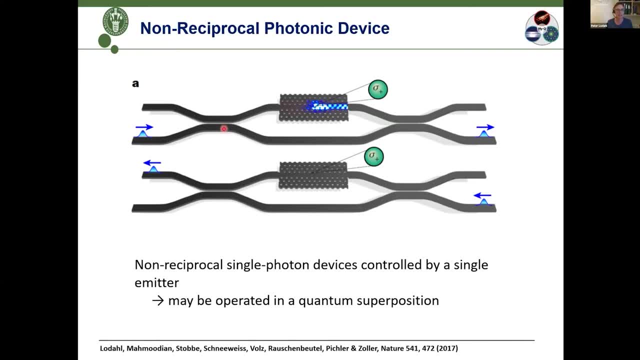 shift into a different direction. well, that's called a max center interferometer. I take two beam splitters and this is then stick in this glide plane wave guide. with the high directional beta factor and this directional light matter coupling, I send in a photon. this is a 50. 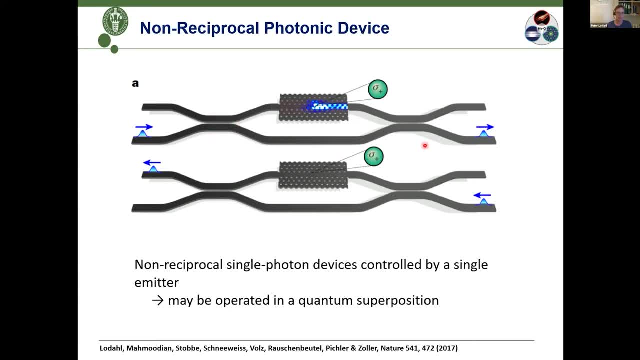 50 beam splitter, so 50 probability it goes either direction. if it comes here it acquires a pi phase shift and then the two arms combine again on the second beam splitter here. but now, due to the phase shift here, this will: this max center interferometer will be unbalanced. so 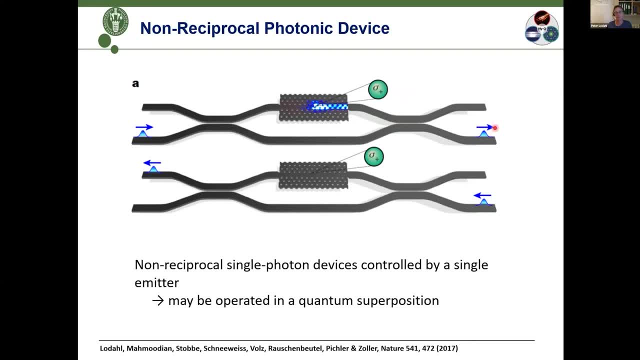 the photon will end up in the same port. so let's say the down port, as it ended, entered. if it entered in the down port it's asymmetric. now there's a pi phase shift in one arm. if I sent the photon back, well, it doesn't see the emitter anymore because d dot e is zero for 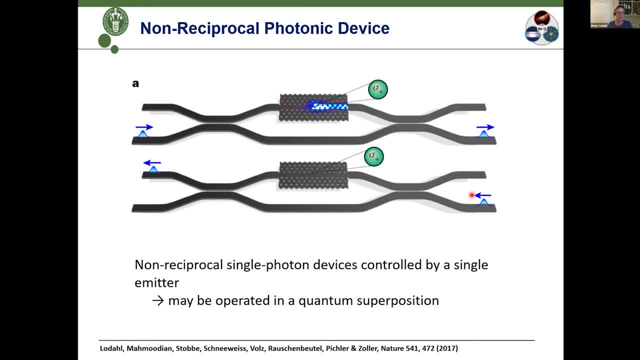 going backward. now it's a symmetric max center parameter, so a photon coming in in the down port will exit in the up port. so you see, I made a non-reciprocal device. I sent in the photon in this port and then, and when it when, I send it back again after two interactions with the emitter. 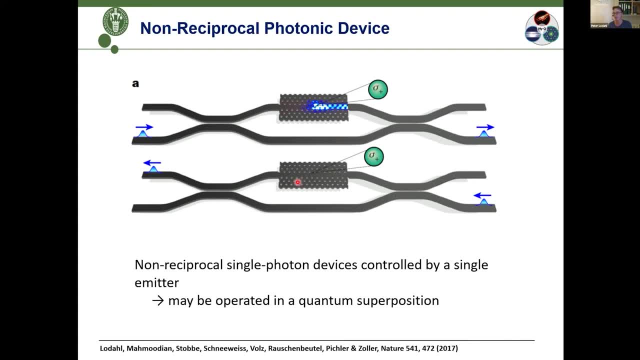 well, in one case it did intact, and when the other case it didn't interact at all because the coupling was zero. the photon ends up in another port that it enters. so that's a non-reciprocal photon device, a single photon device. um, it's controlled by just a single emitter, so it's just a single. 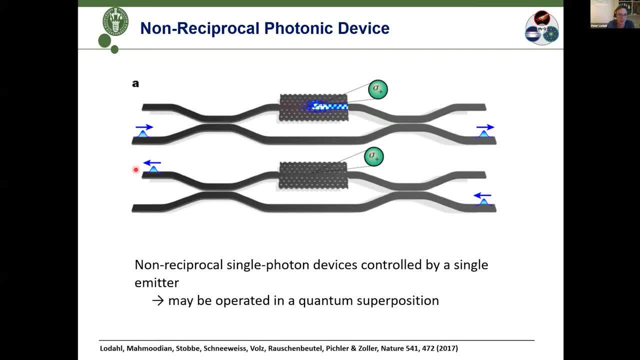 quantum but sitting there deciding, uh, what, what happens? and of course we know quantum systems. we may operate in quantum superpositions, so I could have prepared a spin state, for instance, where I both had a pi phase shift and not had a pi phase shift at the same time, and then you can. 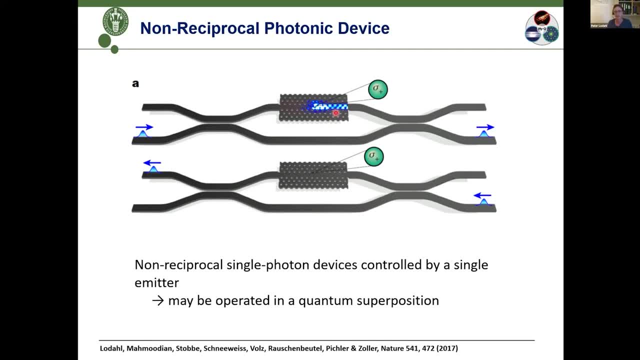 end up with these awkward situations that you both reflect and and or both get a phase shift and not get a phase shift. and now- and this is actually, and since, as I said also, it works even for classical fields- it doesn't have to be a single photon ascendant, it can also be just a weak classical. 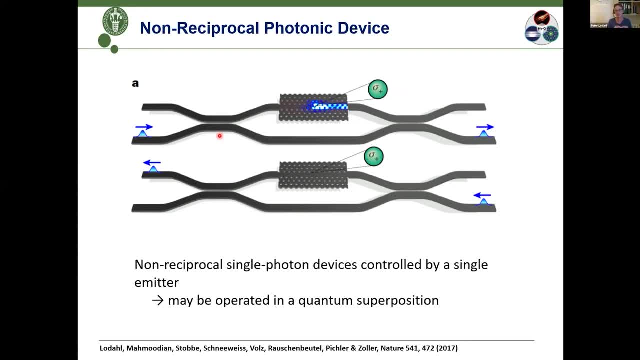 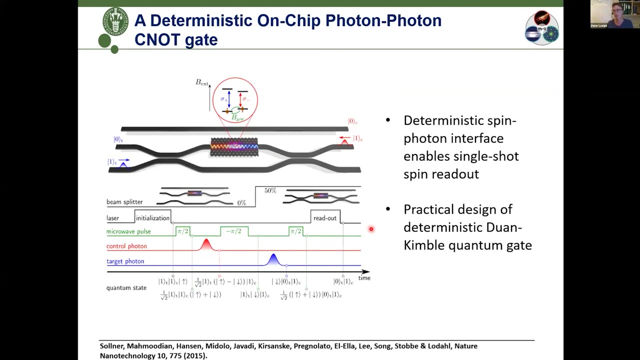 field, then this is actually a way of making us hurting a cat state where I both sent the, the the classical state, to this arm or that arm simultaneously, um, and it's controlled by just a single spin. okay, so, um, you can also make um quantum gates based on that. I think I will skip the details. 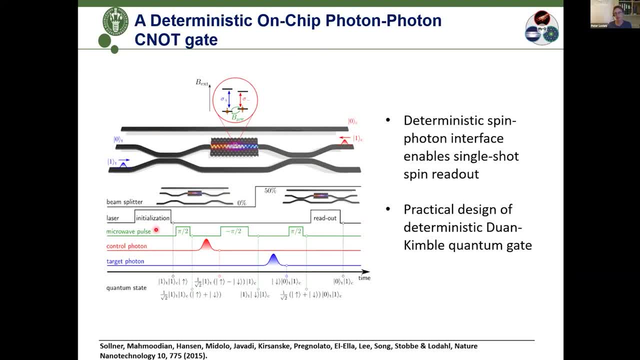 about this here, uh, but but these are actually quite handy tools. that's that, that tools. that's maybe the take-home message, uh, here, that, uh, that, that that you, you can make a, a quantum gate, a c, not gate for photons, where one photon being in a super 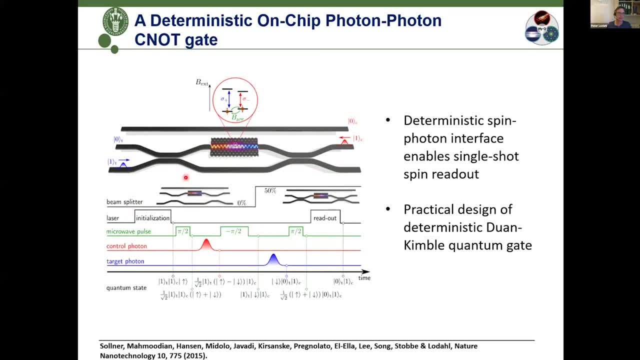 specific position between two waveguides here. a control photon actually controls the, the target photon that is sent in subsequently and I effectively mediate a photon photon operation c, not operation by the directional coupling to the spin or the the in the quantum dot here, and that is a way of of doing some of the things that is really really hard to do for photons. 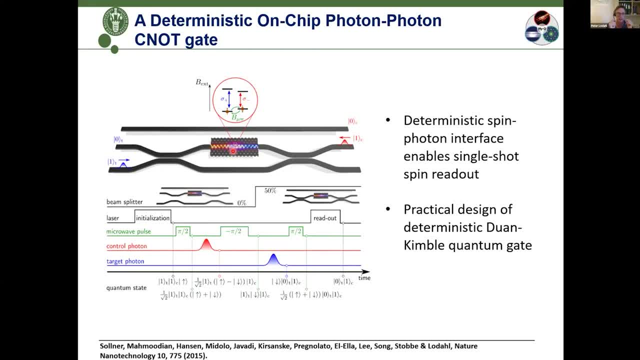 non-linear, inter non-linearly interact with each other. it's a two cubit gate between two photons, mediated by this coupling through the quantum dots, which is, uh yeah, the the the challenge also for quantum computing and advanced application of photons, that photons are good at really many. 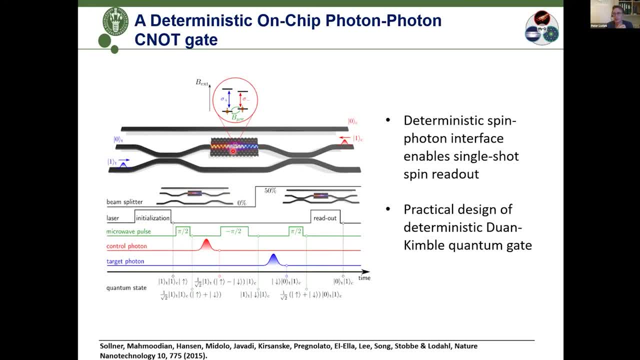 things but mechanical two qubit interactions. that is just really, really hard. the photon emitter interface here gives you a tool, a way to do that and the directionality. the kyle coupling comes in as a quite handy tool here, actually as quite practical tool to get the photons in and 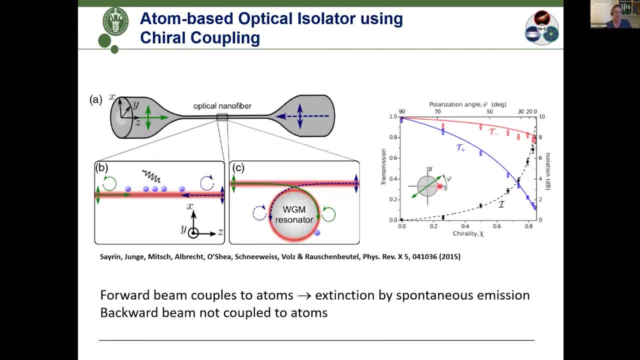 interact with very high efficiency. so, um, yeah, brought an example from about this non-directional photon transport, now a non-reciprocal photon transport. this is a beautiful experiment on atoms, done in arno rauschenberg's group, then in vienna, now and now in berlin. 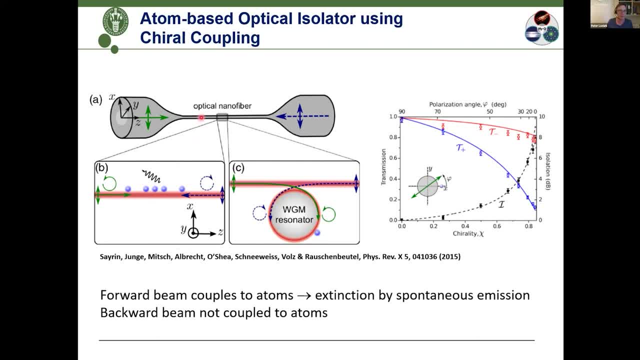 so they are trapping atoms in the vicinity of of these tapered optical nanofibers that i also mentioned in the beginning. they also have what's called whispering gallery mode resonator. so that's that's a resonator where you are sending the light through many rounds through such a- it's a ring cavity essentially, and and again you'll have the. 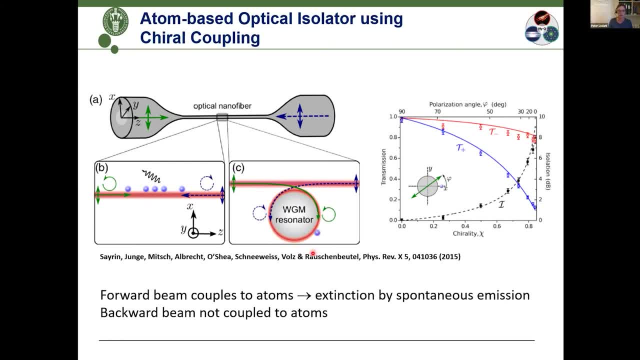 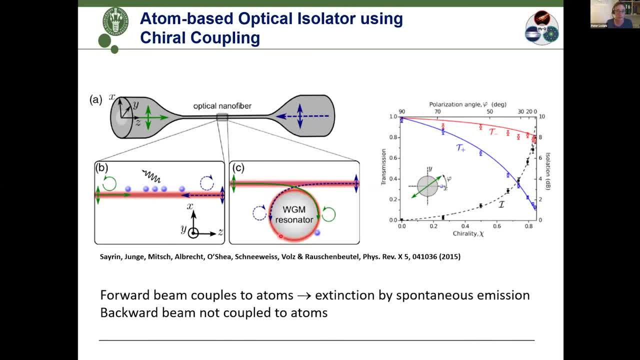 of the longitudinal component electric field And you can have close to circularly polarized electric fields there And that means directional emission, as we have learned. You can say, in the atomic systems the beta factor will not be so extremely high, because you can imagine that if I have an atom trapped here, 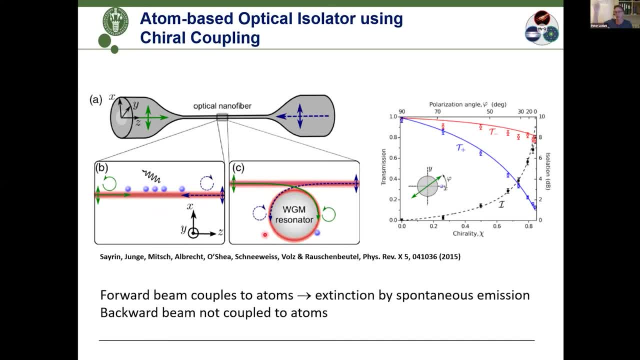 then that could radiate quite a lot out to free space and not just into the resonator, into the nanofiber. So these very high beta factors that we are talking about in the solid state systems with the quantum dots you won't have in atomic systems, 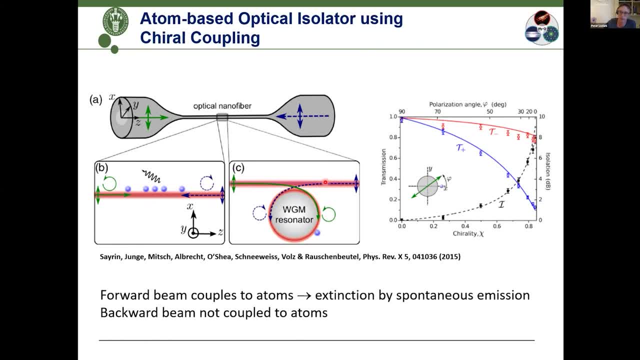 On the other hand, for them it would be much, much easier to take multiple emitters. So having many atom experiments is something that they can do. They can boost their coupling efficiencies in this manner. This is something that is much harder for us to do. 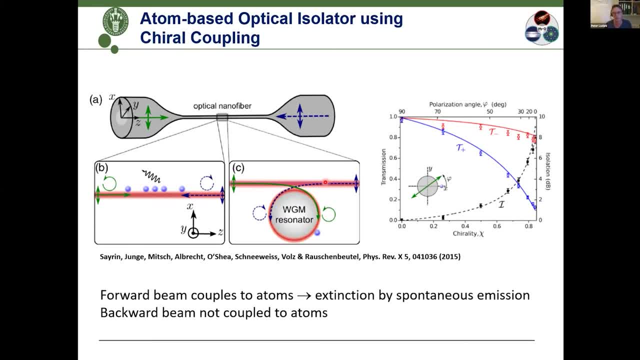 on the solid state platform, And that's just two different regimes. also, the applications of these kinds of systems. The physics is very much the same. Okay, so they did a great experiment here, where they're sending light through these nanoboom fibers. 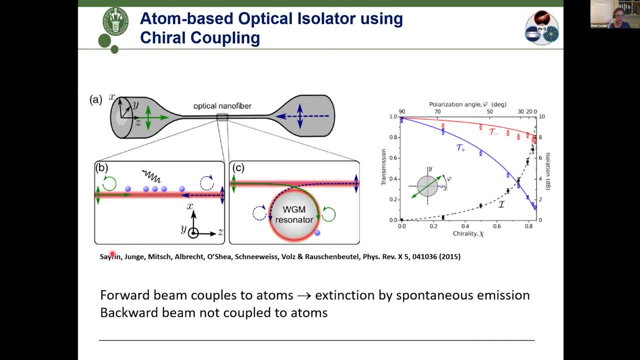 And I think they did both for the resonators fibers. Let's just look at the fiber case. for simplicity, They sent light in from left to right And in this case you have the circular polarization and polarized emitters here in this case. 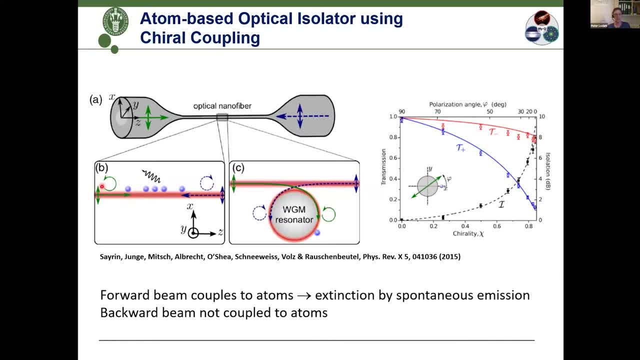 de is small, So you don't have much interaction with these atoms that are sitting there next to the fiber. If you send light in from the other direction, from right to left, you have the right circular polarization to interact with the emitter. 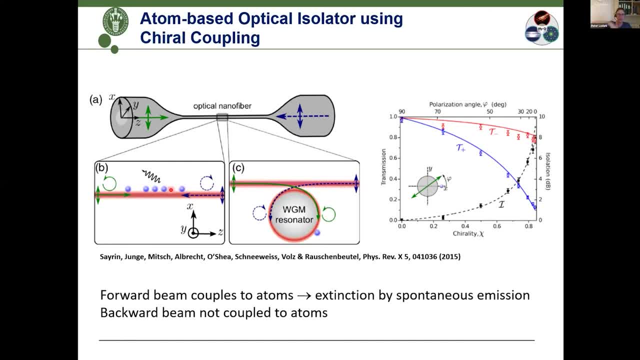 You're exciting. the atoms, And the atoms actually in most cases just radiate the photons out of the structure, So you lose the light in that case. So this is actually an optical isolator. You can get light through one direction. 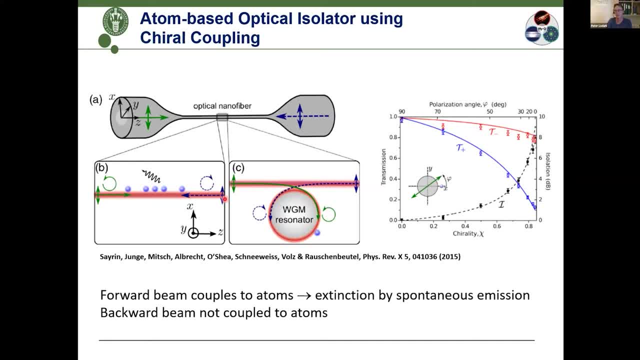 but if you try to send it in through the other direction, it's radiated out by the atoms to free space. So you're attenuating the field And it only works by this because of this chi-light matter interaction. that means that this de thing 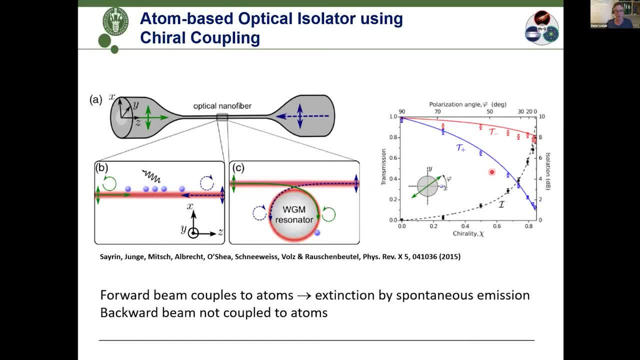 that we are playing with all the time Here. they have measured, then, the isolation of this going in the two different directions, versus a chirality where they change it. They're changing the polarization of the mode that they're sending in from the nanobeam waveguide. 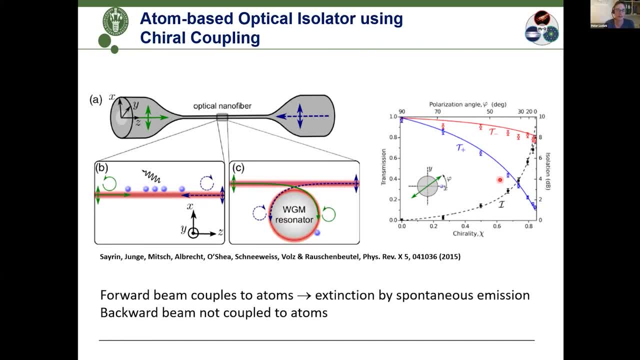 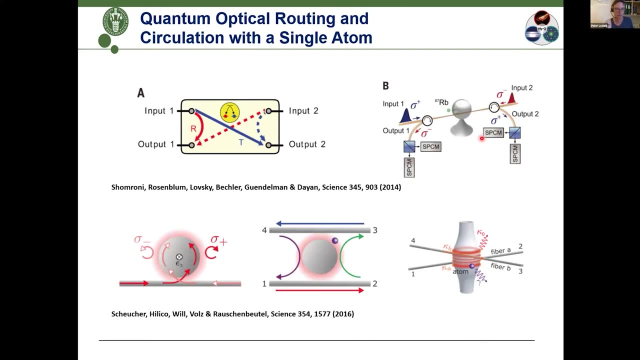 And they see that this directional coupling means that you can attenuate the beam simply by radiating out to other modes. Okay, Yeah, so these are other examples from Arno's group, Rausen-Beutel's group and also from Barak Dayang's group. 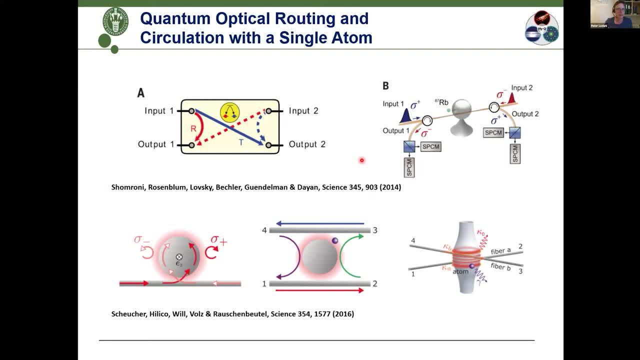 atomic physics groups that take it one step further and use this really to do optical routing, So then they can send in again light through one waveguide here. Now you're coupled to this resonator here, And in one direction. it does not interact with the atoms that are. 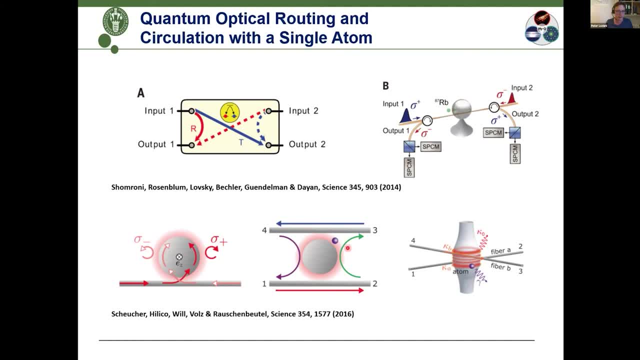 I mean that's one atom here that is trapped then in the vicinity of the ring, like here for instance. In the other case you do interact with the atom because de is optimized for it And you will get different phases. 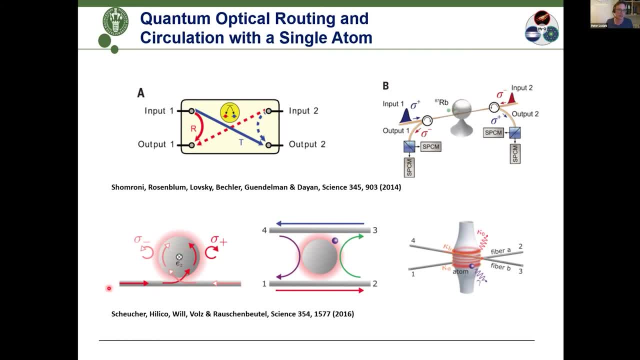 And you will get different phases And you will get different phase shifts in this resonator. So that means that you can, in one case you will pass right through, You will go from one to two. In the other case, if you send it in through the other direction, 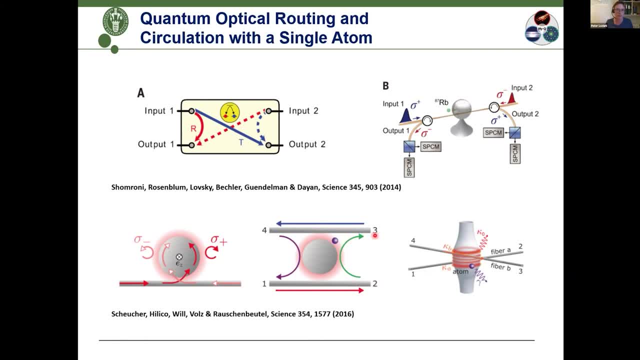 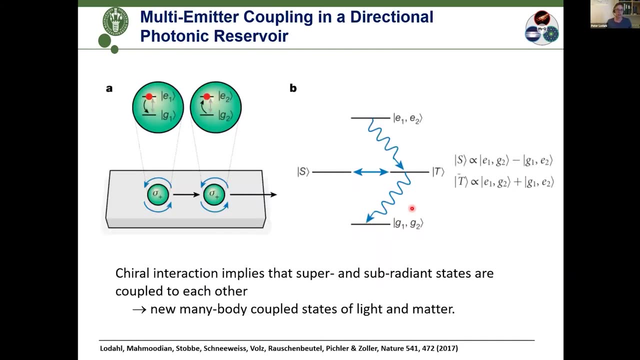 you will get a different phase shift from the interaction. to you You'll mean that you will go from d, from two, to three. So this is really routing with a single atom of the light sent in through different directions through the waveguide. So a little bit more details about some. 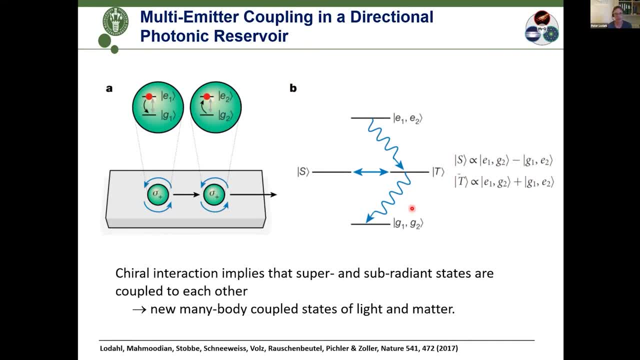 of the new opportunities here, also for new physics and also, yeah, quite open questions here, because it's really a new paradigm- you can say in light matter interaction- to have this directional emission, And so far I spoke just about a single emitter. 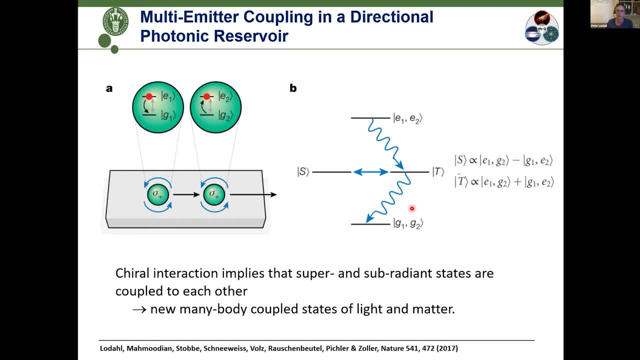 And it could give directional emission. It can also get directional scattering and these directional phase shifts that were used for non-reciprocal photonic devices. And you can ask about what happens if I start to take multiple emitters in these waveguide systems and start to directionally couple them to each other. 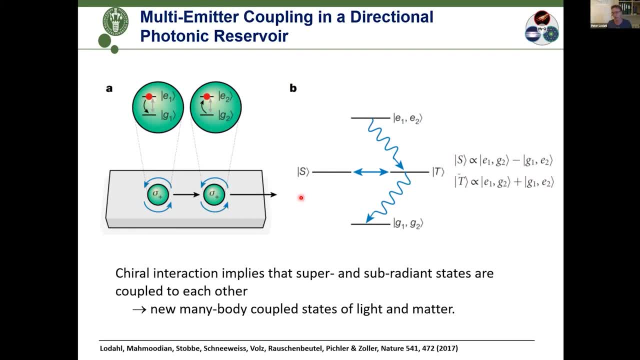 And I would say already two in a, without this chirality is quite interesting physics because, as I said also in the beginning, I think when the beta factor is so high, I think when the beta factor is so high, I think when the beta factor is so high, 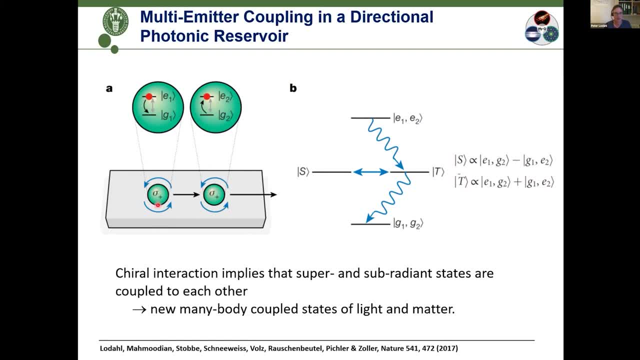 then it's like if the world was 1D. So how do two emitters interact with each other- that dipole-dipole interaction- and that decays quickly as you move these dipoles away from each other. the interaction decays as one of our cubed. 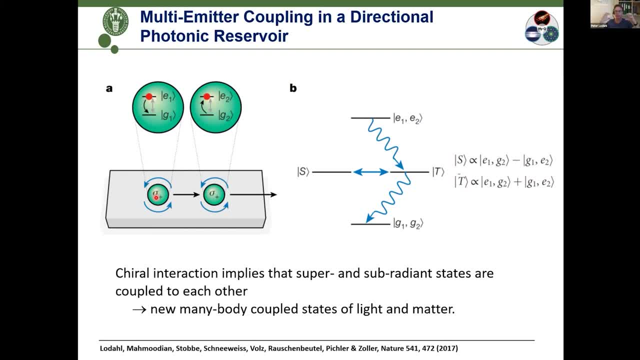 this dipole-dipole interaction, But in 1D it's not like that. You will actually have infinite arranging, dipole-dipole coupling. So when I have a beta factor that is so high, quantum emitter believes that it's in a 1D world. 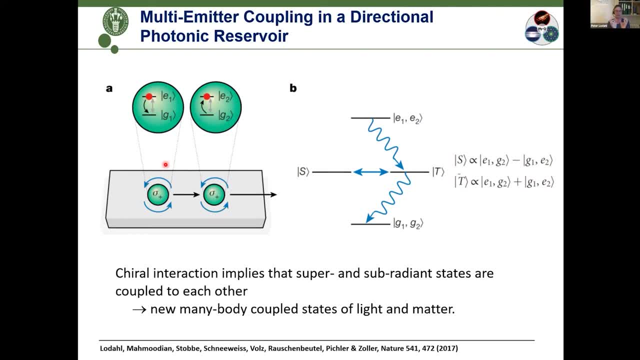 It can only interact with it with a single mode, And that means that, putting those two emitters even far away from each other, they would still interact through dipole-dipole interaction. Okay, So now we are adding this directionality to this game. 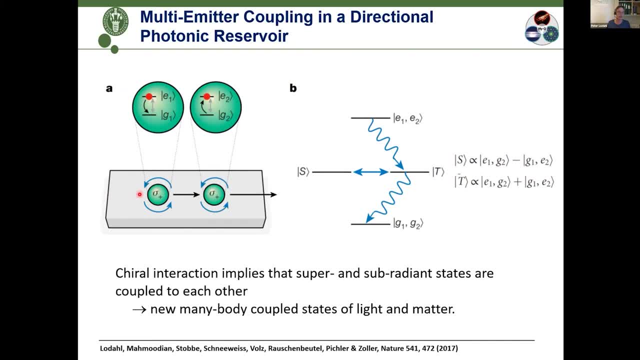 So now I'll have two emitters. They are circularly polarized emitter sigma plus- and they can only directionally couple to each other. So the one to the right here can see the one to the left, but the one to the left can't. 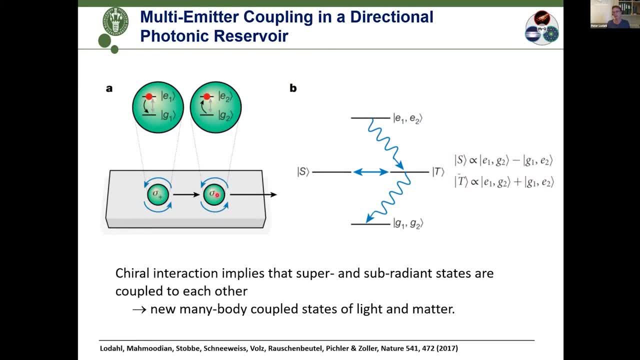 But the one to the left doesn't know that the one to the right exists because of the directional coupling, And that of course, changes the physics. So what happens with dipole-dipole interaction is it gets super-radian state and sub-radian state. 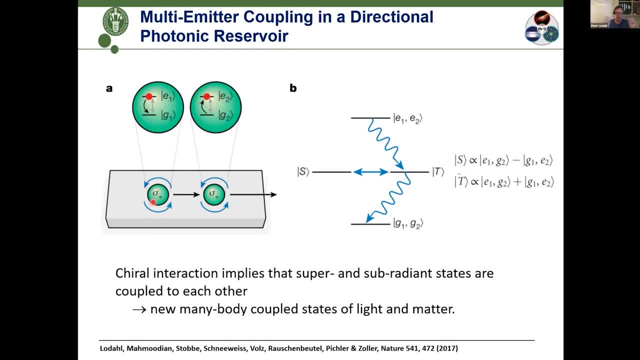 And that is really due to also that you have symmetric coupling between both directions, that you start to create these super and sub-radian, the eigenstates of two entangled, two coupled emitters with each other. When I have directional coupling, that changes. 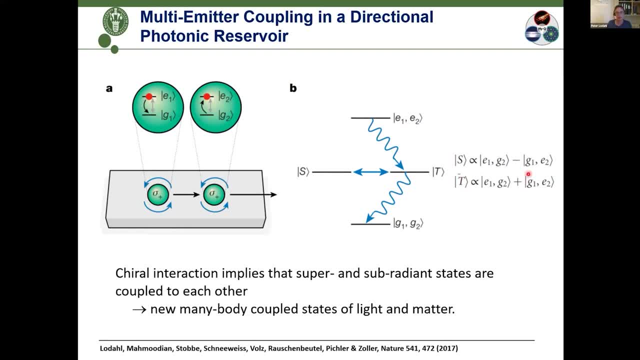 So you'll start to couple those two or you will start to interact and entangle those two quantum emitters differently. where this chirality becomes an additional complexity And more generally, I think there's really a bulk of new opportunities that can be explored here. 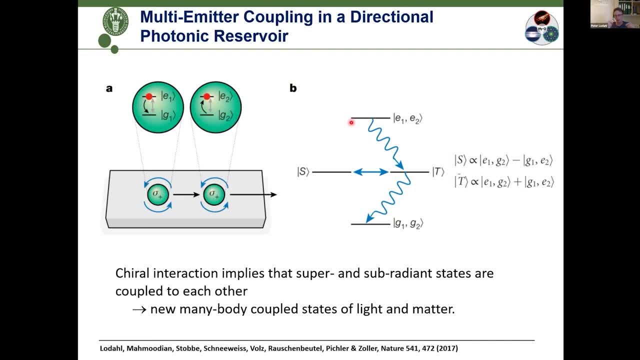 Because those are just these sub- and super-radian states, are just the matter states and how they can be coupled to each other, And that's only just a few excitations in the system, if I have one excitation shared by those two emitters. 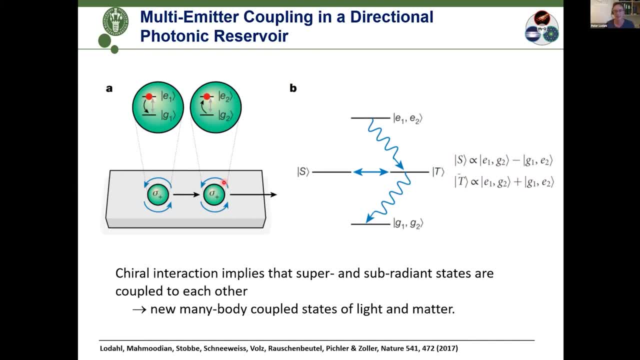 But now if I start to send photons in to these emitters, then I have the nonlinear interaction between those photons coming into the emitters and doing really a high-level interaction. So it's really nonlinear quantum interaction And it's really a very interesting and open research. 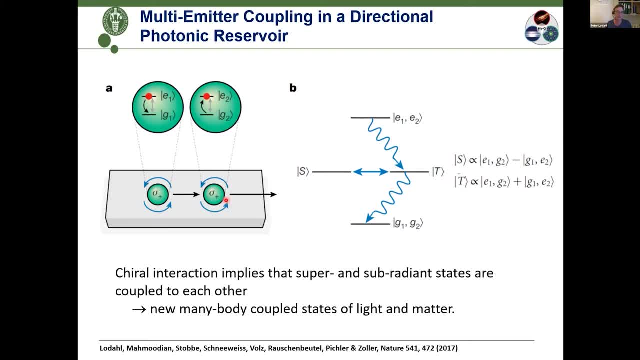 questions on what quantum states and what many-body couple states of light matter. can I engineer, can I possibly make where you are having that very efficient and directional coupling between emitters? And it's a really complex system because it's a big space. 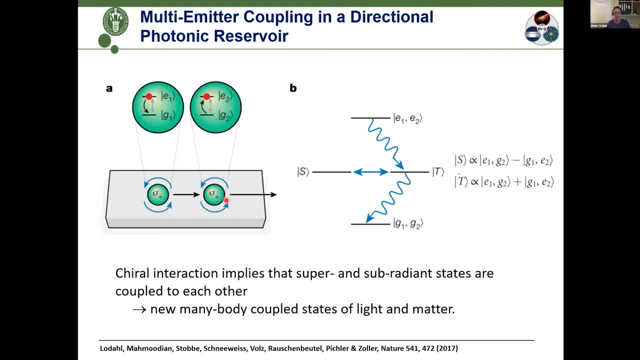 You send in photons And if you start to launch more photons, I have the nonlinear interacting with the emitters. here It's a quantum system that very quickly explodes And I think some analogies with electronic systems and electronic transport systems are really interesting to think about. where 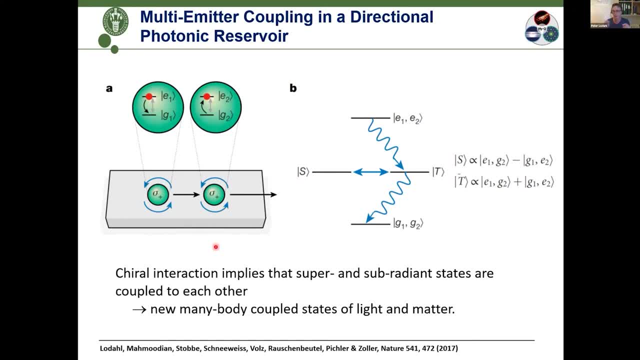 I think this directionality is something that directional coupling between emitters is something quite new and possible to engineer here on your photonics platform. So there are many people really looking into that and seeing also complex behavior like photon-photon bound states, how they're forming due to the interactions. 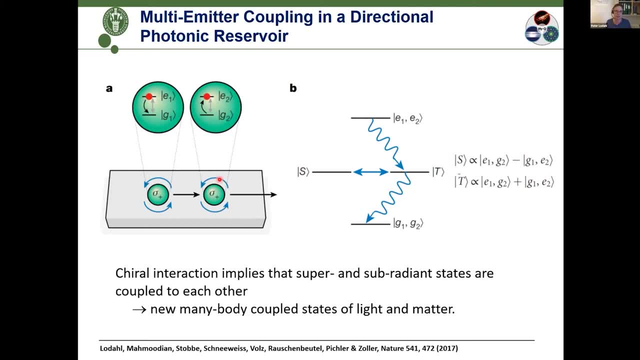 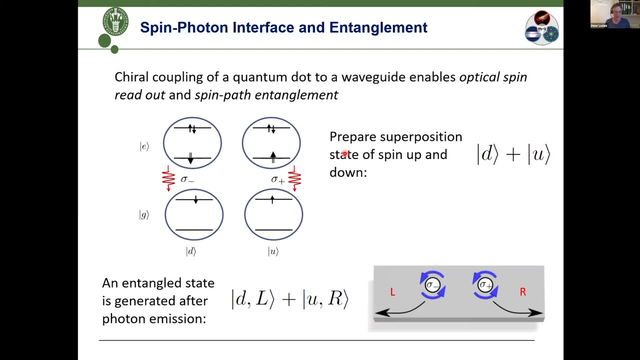 and the role of the chirality, for that- And that's a really hot research topic Peter Soller, Derrick Chang, many others are looking into. I will give you just an example of what we are particularly interested in and working on in this direction. 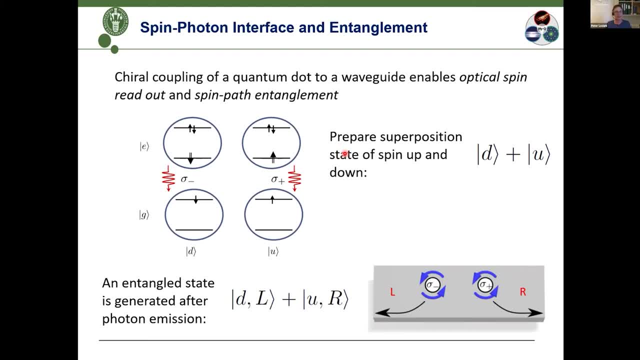 Because chirality and chiral coupling here gives you an interesting opportunity to do in the realm of spin physics. So I didn't speak about spins before, But I can also tunnel in a single spin inside the quantum dot, And now I'll have a four-level system like indicated here. 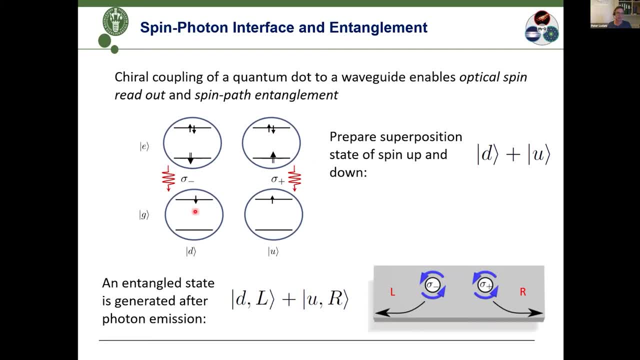 where the spin state could be. I prepared the quantum dot with spin state down or with spin state up, And then I can excite this system to what is called charged exciton, And I have those two different possibilities of that. So those transitions here this is a sigma minus transition. 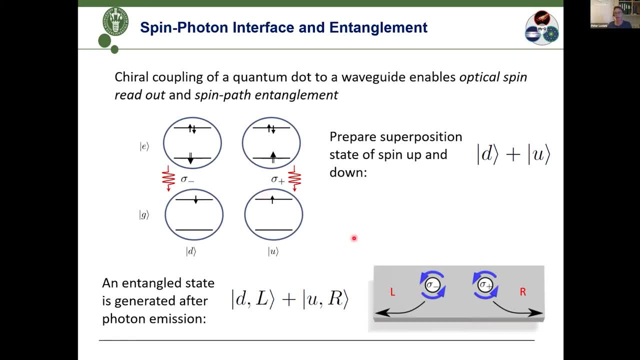 sigma plus transition, circularly polarized transition, So I can play all these tricks with directional emission. And then you see what I can do. I can apply as a very practical thing, apply that directional coupling forward And then I can actually read out the optical spin. 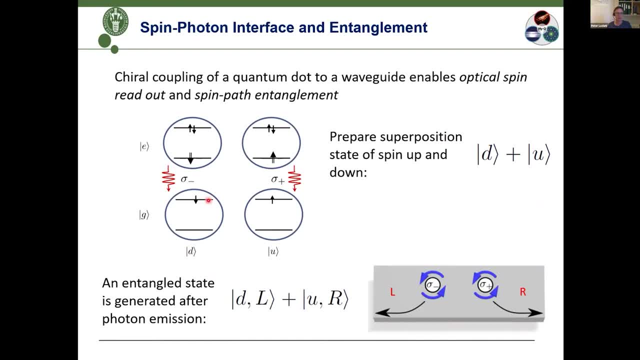 If I have some kind of spin state- I'm not really aware of which one it is- I will excite the system and emit a photon. If it emits a photon to the left. it was a sigma minus Spin, a sigma minus transition. the spin is pointing down. 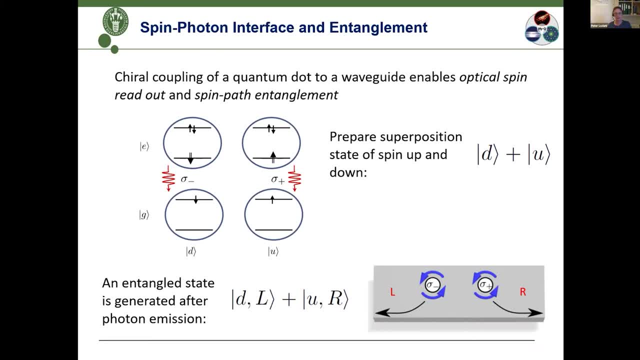 If I get a photon click in the detector out here, the photon in a click in the detector off here it will be in the spin state up. So it's really a one way way of reading out the spin state by just seeing at what direction did the photon go. 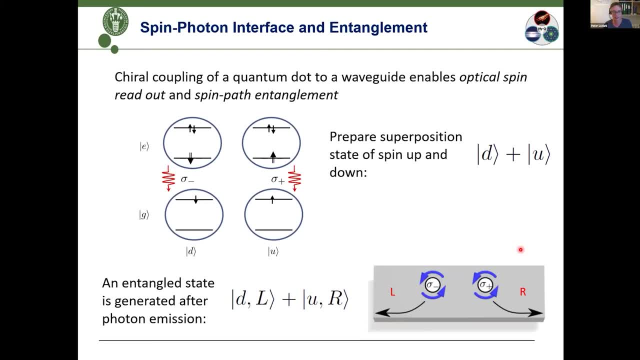 I can also actually use it to produce a path entangled state, because spins, of course we can prepare in superposition state of down and up at the same time. and if I then excite this system and it emits a photon, then well, it can emit on each of those transition and if it image on the 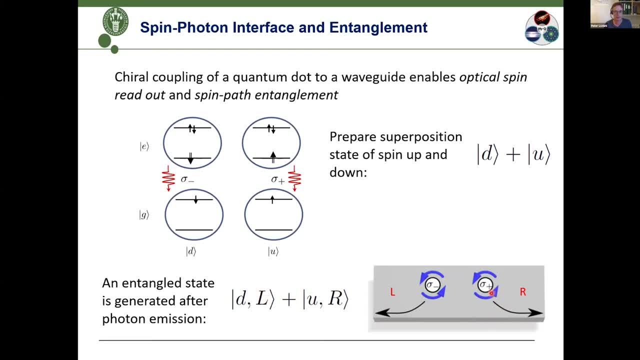 on the sigma minus transition goes to the left. if it emits on the up transition, it goes to the right. I do not know which one happened, so I'll end up in an entangled state. if the spin was down, it emitted a photon to the left. if the spin was up, it emitted a photon to the right. so that's a way of 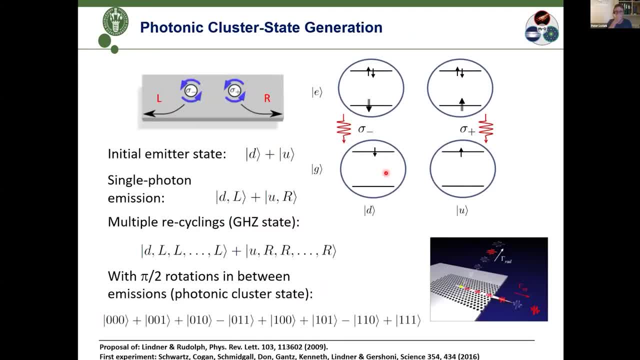 making spin photon entanglement. and then there's a very nice and interesting generalization of that: that you can use that actually to produce multi-photon entangled states. because I can repeat this many times- I can excite the system and emit it produces spin photon entangled state. I can do a. 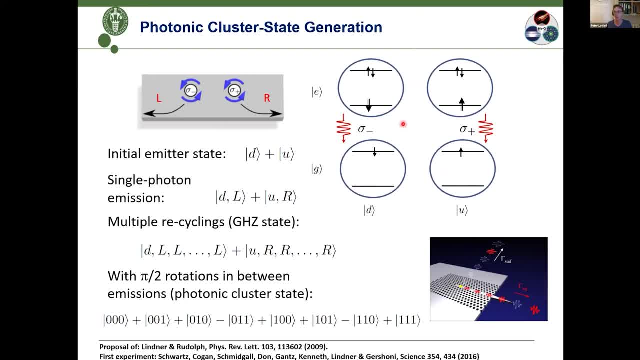 rotation on the spin, and then I can do it again: excite, emit, excite, emit, excite, emit. this is what we're very good at on the quantum dot platform, because of these beta factors are so high that I can collect the photons with very high efficiency and it turns out, if I, if I do it. 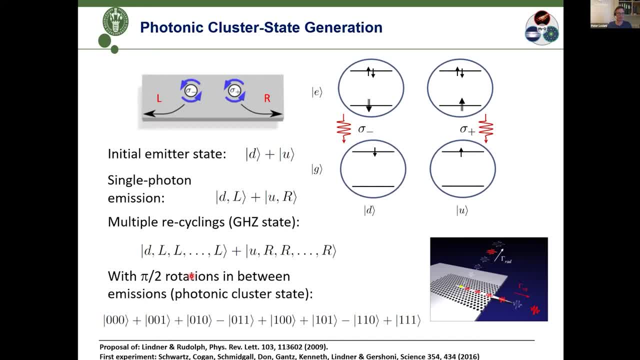 n times then I'll get an n photon entangled state. it's called a GHC state Green-Burger-Horn-Seilinger. that's really a multi-photon entangled state that if the spin was pointing down, then the first photon was emitted to the left, and so was the second, so was the third and so on. but if the spin was pointing 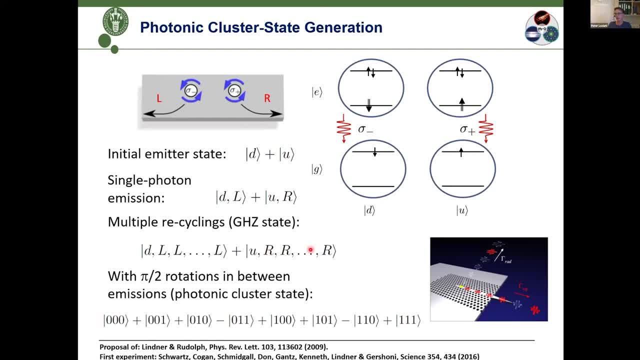 up. then the first photon was emitted to the right and that hold for all subsequently emitted photons as well. yeah, five minutes, thank you, um. so yeah, that's. that's just a very practical application of this photon emitter interface and the Kyle coupling there to to to start introducing and, and and. 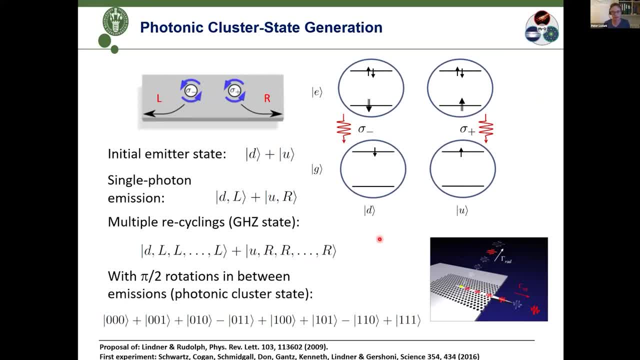 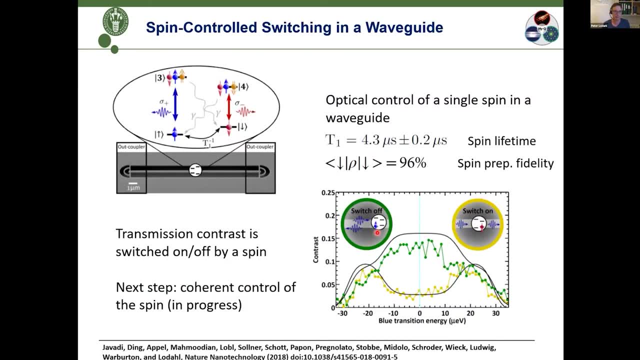 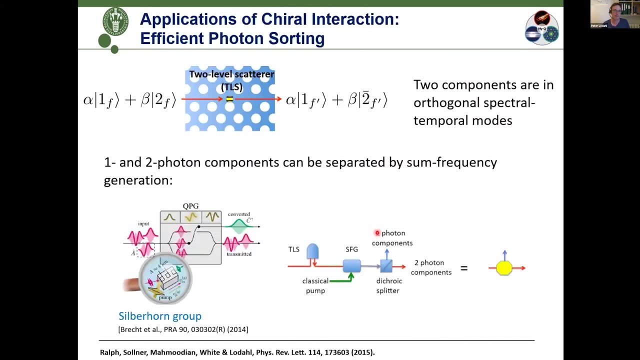 making entangled states, multi-photon entangled states? okay, I think I will, let's see. sorry, um, I think I will end with this one, as I as another little application of um, of the, the directional coupling, and that is emphasizing also the non-linear properties of this. I already said something about it that I had. 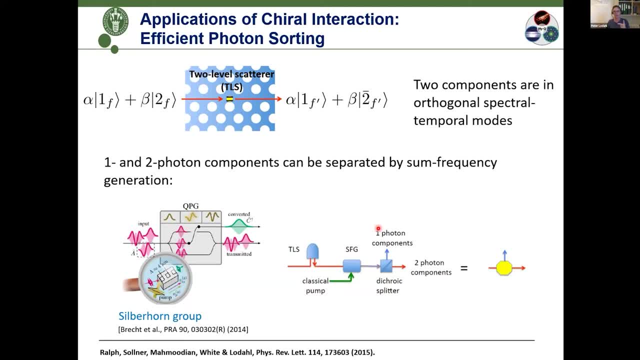 one photon- I just very briefly said one photon interacting with an emitter. that that, that this interaction means that if I send in another photon at a different time, then I effectively mediate a non-linear quantum gate between those two photons and and I can do something else. I can. 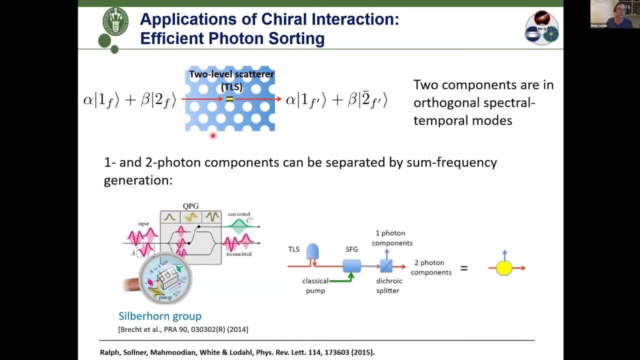 actually send two photons, or superposition of one and two photons, in on the, on the quantum emitter at the same time, and because the beta factor is so high and I have a quantized emitter, two level system in the most simple case here, um, then the only one it can only interact with. 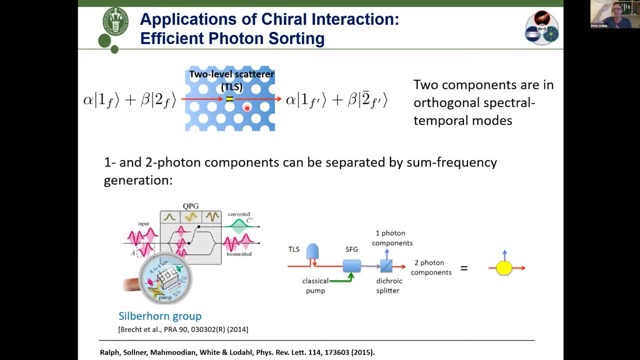 one photon at a time. I cannot interact with. I cannot excite an, an atom quantum dot with, with, with two excitations. it can only one at a time. it's a quantized emitter, that's a poli-excitation solution principle. that prevents me from doing that. so that means if the beta is so high, then 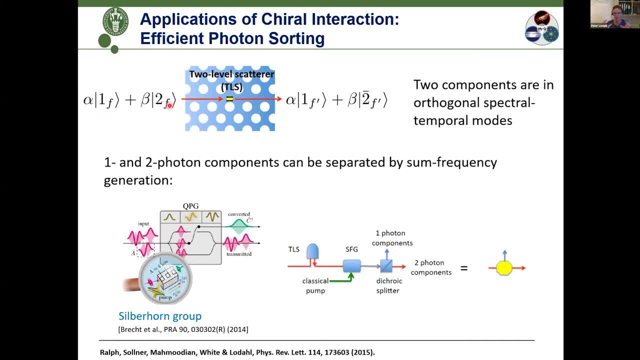 there should be a difference. if i try to, if i come in with a superposition of one and two photons, it will have to do something differently to them. it will scatter. we talked about that already we in this kyle coupling: if i send in a photon i'll get a pi phase shift on the one photon component. 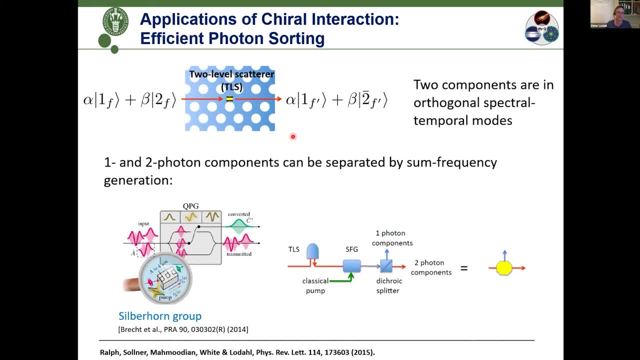 and that's not. much else is happening to that, but the two photons. they will have to be distorted by the, by the coupling with the emitter coming with the two photon pulse and, and, and there's some probability that the photon comes first in this pulse or late on the pulse and that will distort. 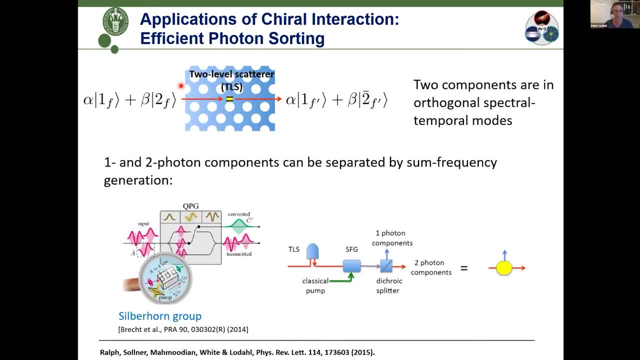 this pulse because it will create quantum correlations and quantum entanglement by the distorted by the interaction with the emitter. so one and two photons will be scattered into different spectral temporal modes simply because of the poly exclusion principle prevents the quantum emitter from interacting with with with more photons at the same time. and what we worked out here is. 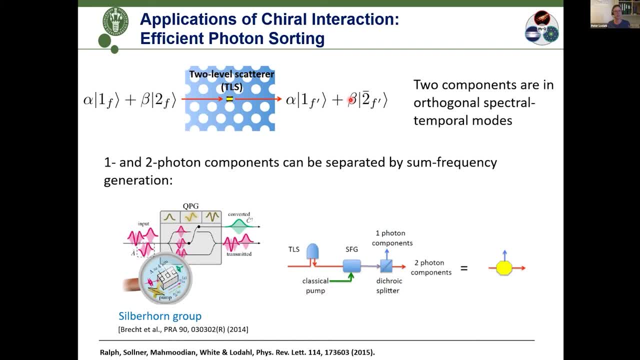 actually a way of making use of that distortion. it's a. it's a highly complex thing. i send in a pulse of light that's a multi-mode system and i start to change that pulse of light due to the interaction with the emitter. it's. it's surprisingly rich and complex even that system. um, and it and. 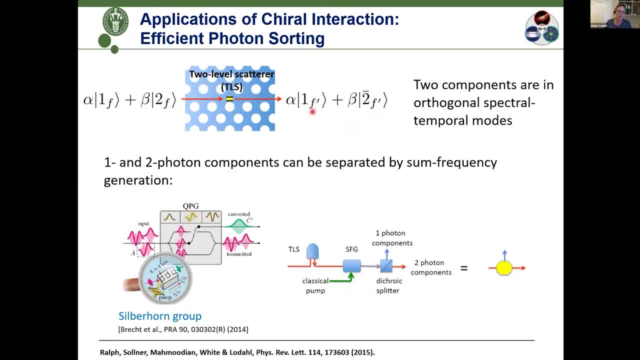 here we worked out a way that that you can actually make use of that distortion. um. so if the i, if i control the, the pulse length here, probably i can actually end up in a situation where these one and two photon components are scattered into two different spectral temple modes. 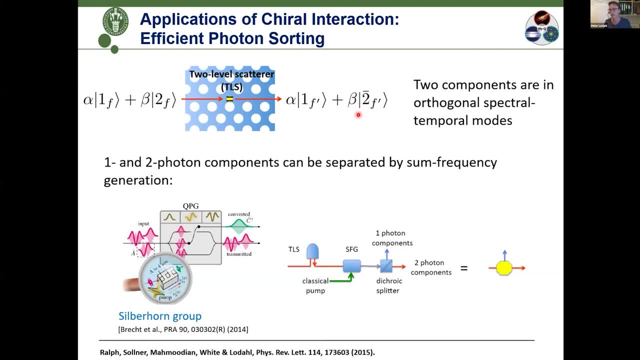 that i could possibly um separate from each other, so that's what's called a photon sorter. i could have a device that i send a supposition of one and two photons into and out in one mode goes one photon and out in another mode and then i can actually change the propulsion length. so i can actually 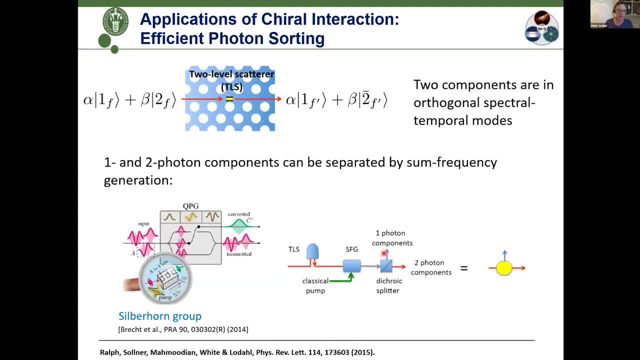 mode goes two photons, and it turns out that for to get this to work, you actually also need something that, that, um, that that that that selects us a a specific spectral temporal mode and we can do non-linear conversion to. to actually do that, i think i'll skip the details here, but the bottom. 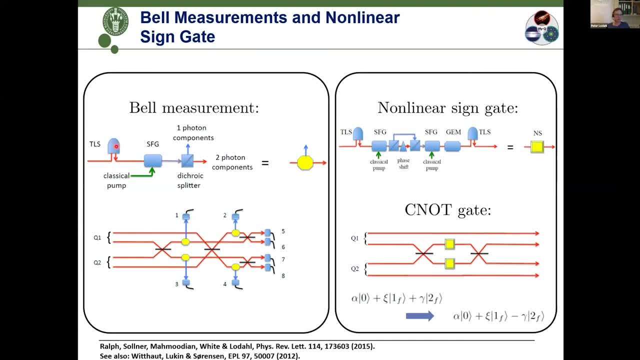 line is the following: uh, that that now i'll have a photon sorter, a scatterer, that i send in a two position, one and two. i do spectral temporal mode selection, and then i will have one photon component going out in one direction, two photon components going out in another direction. 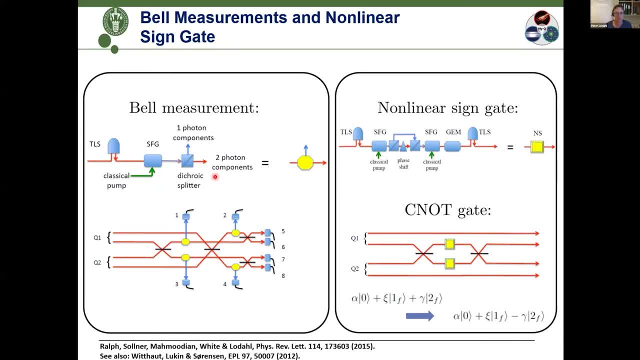 the modes are being- uh, the one and two photo components are being split into two different spatial modes, and that is one of the things that that is hard to do in photonics because it's a non-linear interaction. right, i have to position in, i get one out and one out. 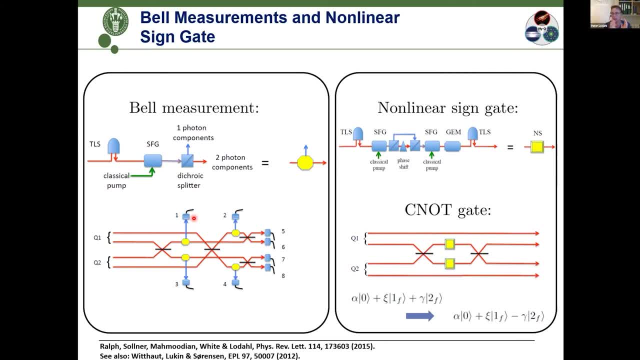 arm and two out in another arm, so that that's exactly what photons are have have troubles with, and that means that many of the quantum computing or quantum application of photons are trying to circumvent that. these kind of challenges that they don't have have good non-linear interaction and 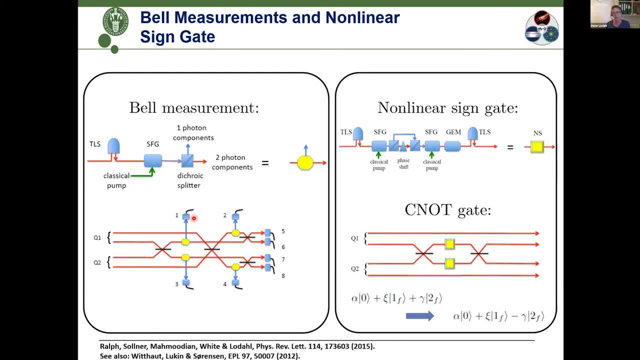 that's actually the reason why many quantum computing architectures, and so i mean the resources, are dramatic when scaling it up to to, to to advanced applications. you need ancillary photons in order to to do that. so now the interaction with the emitter, here the light matter interaction. 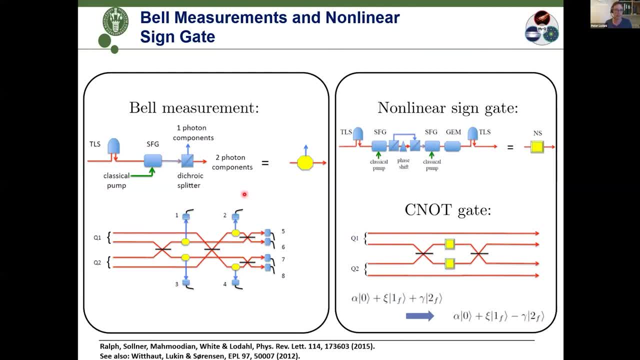 with the emitter is actually way of of of doing it, and here you have worked out that's a technical thing but but a way of exploiting particularly this photon, sort of x to what's called a bell measurement. that you can, if i send in any com combinations of of path encoded bell states. 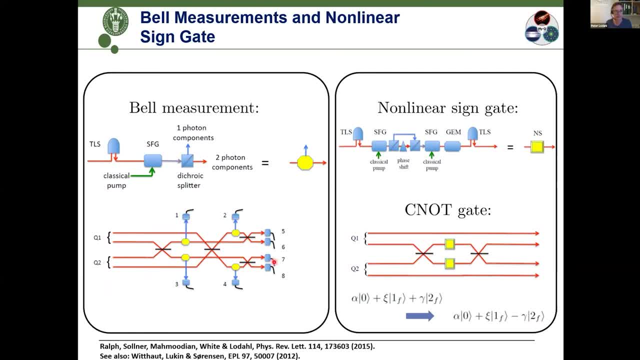 in these four waveguide modes. here i can. with photon detection events, here i can actually say i can, i can. i can with certainty say, depending on where the photons end up, what bell state, uh, did i actually send into the system? so that's called a bell analyzer, a deterministic bell analyzer, and it also even enables you to make 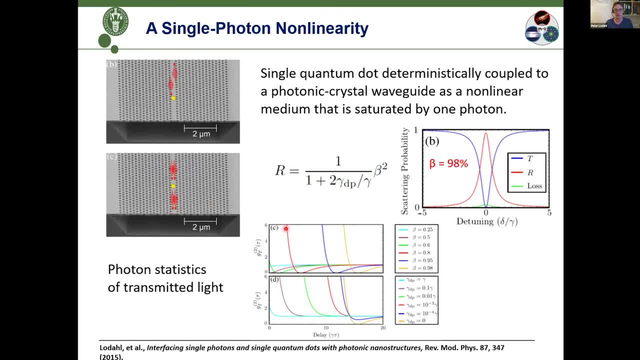 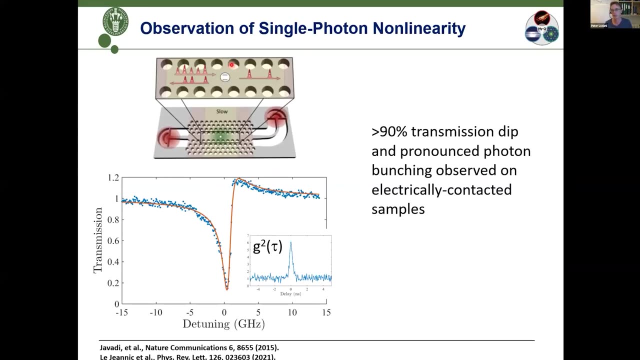 quantum gates. but let's skip this. um, i think i will. i will wrap it up here. i think we have covered most of what i wanted to say. some of these things with the photon non-linearity- that's what these slides about- also work in the lab. so we see single photon non-linear operation very well in these systems. 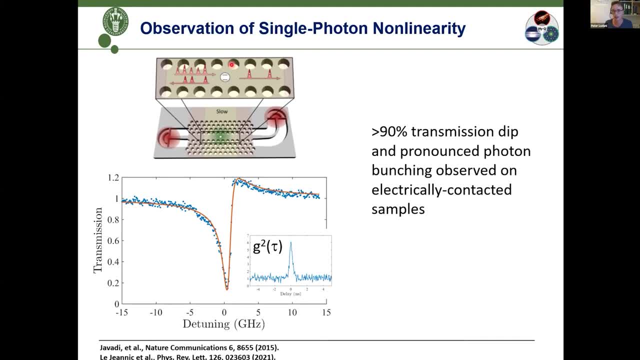 decoherence that i said absolutely nothing about- and today is key to get these things to work- and also the multi-photon entanglement uh sources that i briefly mentioned. any decoherence processes uh needs to really be be dealt with seriously and and that is uh that, that. that, that is another. 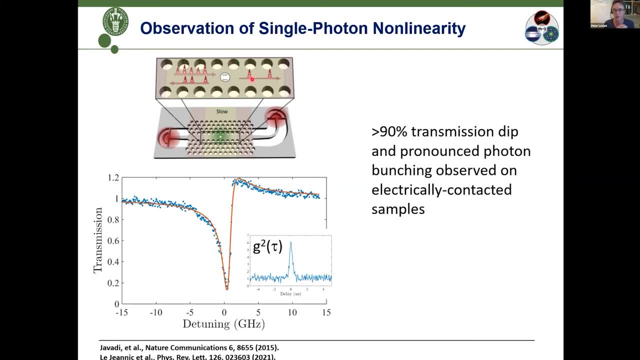 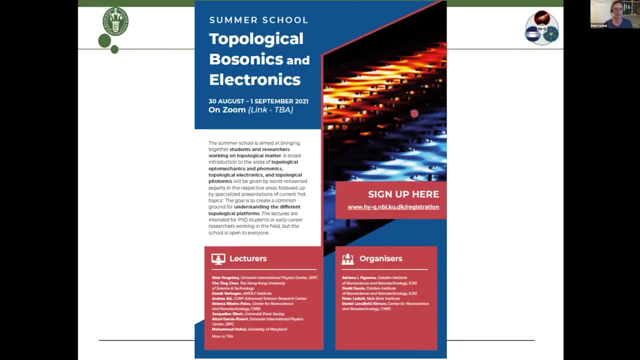 part of un 새로운 ge ми mensch by secretary deutsche z social tournament. uh, so the idea is exactly what uh, sergio was was alluding to: bringing together together communities in photonics, phononics and electronics to start first attempt to, to start getting a. 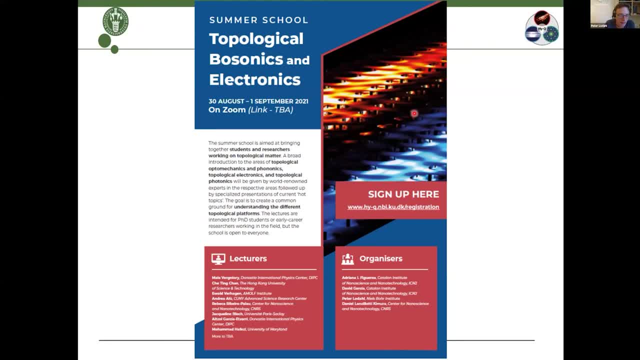 common language and and maybe exploiting some of the um concepts, uh, and, and also some opportunities for interfacing systems. that would be really interesting to do. so this is within torture, and you see the lineup of excellent speakers here, and i encourage you to to sign up for the. 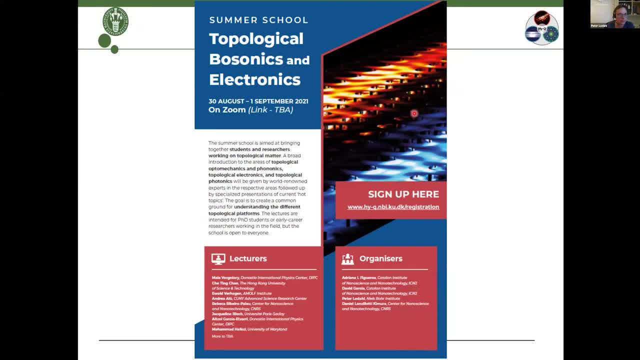 school. it will be a three-day school, all on zoom from the 30s of august to first of september, so thank you very much and i'm happy to take more questions. thank you, there is a wonderful tutorial and now we have several minutes for questions. please go ahead. 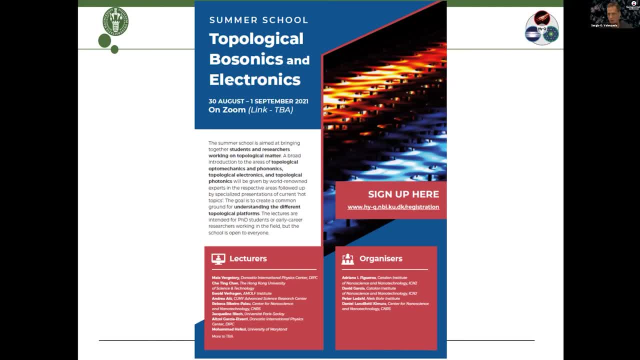 type in the questions or directly raise your hand and then, if there are more questions, you will have the opportunity to have a coffee with peter in the coffee break. please, i'll let you know if you have any questions. or if you have any other questions, please feel free to put them in the. 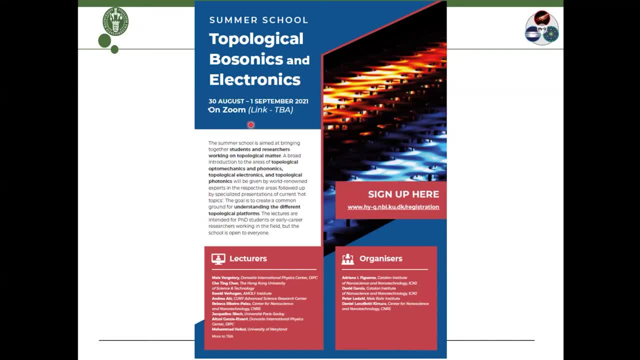 chat box and i will try to answer them as soon as possible. i don't see any questions immediately. i don't see any questions immediately, please. you're also welcome to unmute your microphone, if that is easier. you need to raise your hand and then we will unmute your, your mic, okay. 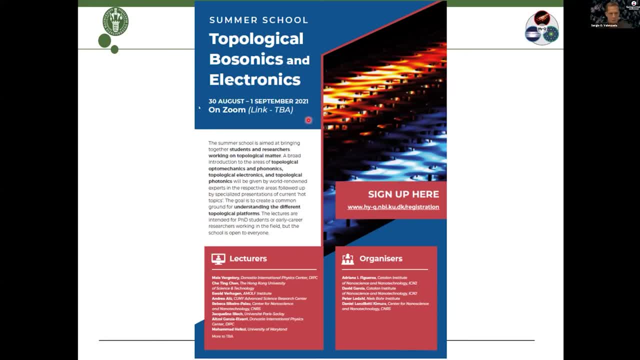 there is a thanasis that has a question. uh, you, you can. you can talk directly, thanasis. yes, um, thank you very much for this. um, very nice talk. uh, personally, i'm not in the field, so i have a very uh naive question. um, what about the temporal? um relation between? 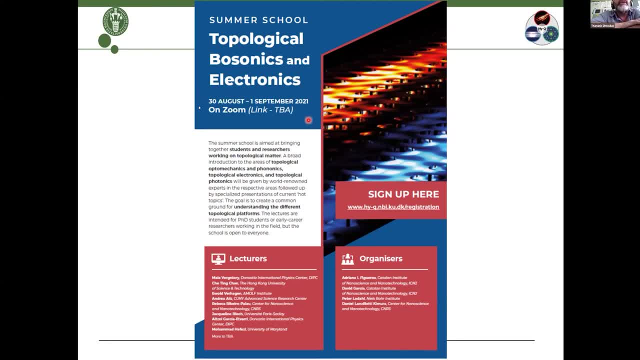 the different photons, uh, whether the photons are uh interacting sequentially or after a time delay between each other, and so on. probably you mentioned that, but i i may have missed the point. yes, is there some um information at all? oh yeah, this is. this is a beautiful question, um, and and a very deep one. 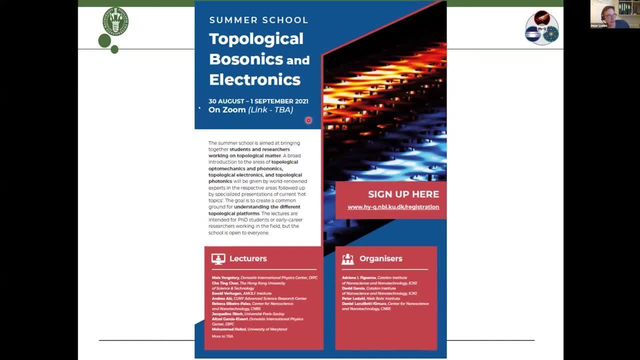 actually so, um. so it really depends on um, on it's something we can control in the experiments- um, so, um, and there are two regimes essentially so. so there's regime where we start with just um, an empty quantum dot, so then it's just a two level system, and then there is a time, um, 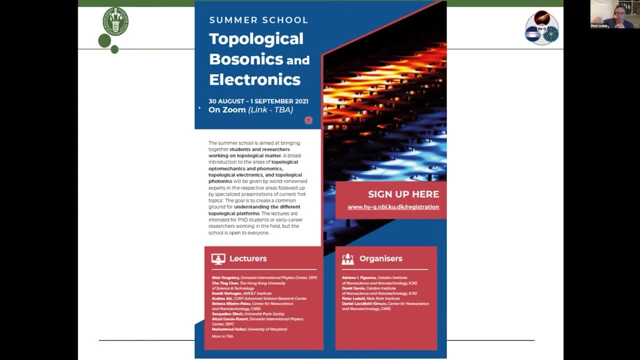 memory. you can say of your quantum dot, which is the lifetime of a quantum dot, so that's the time that you can control it. um, and then there is a time um memory. you can say of your quantum dot, which is the lifetime of the quantum dot. um, and then there is a time um memory. you can say of your quantum dot, so that's the lifetime of the quantum dot. 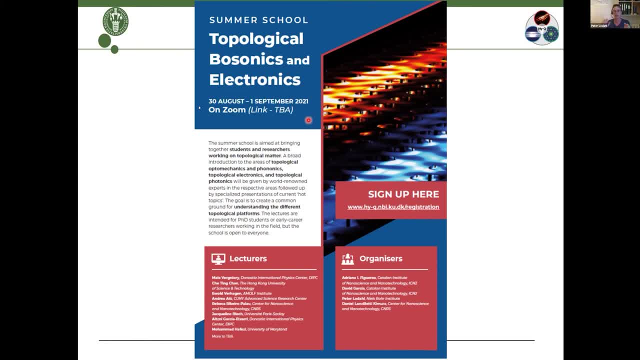 so that's about a nanosecond or so. uh, so so that would be the that would be the time that that so that the quantum dot can introduce interaction between two photons, so everything that goes on on sub one nanosecond timescale will give rise to very complicated correlations actually between 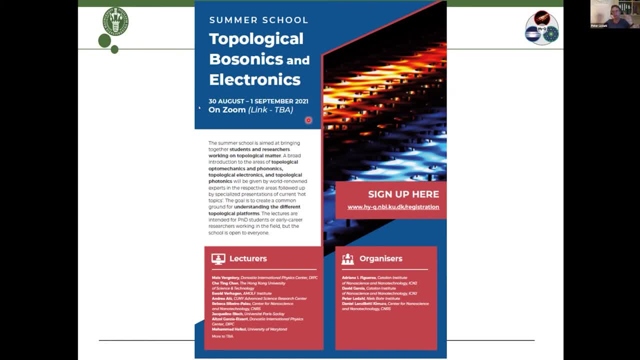 the two photons. if they're further away than one nanosecond, then it will just uh independent. it would be like two independent photons interacting with each other. if they're within the one nanosecond second time scale, then you get the the. those can be two pulses. it could be 200 picosecond pulses. 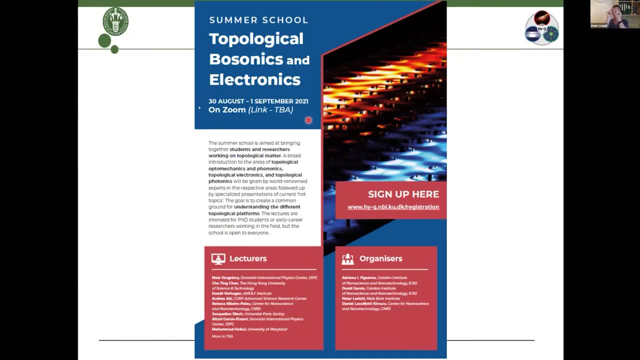 that you're controlling the the time in between, and then you can really start to to play with these advanced correlations, and that's a surprisingly complicated system. it could also be a pulse containing two photons, but then it was was like a 500 picosecond pulse or something that. 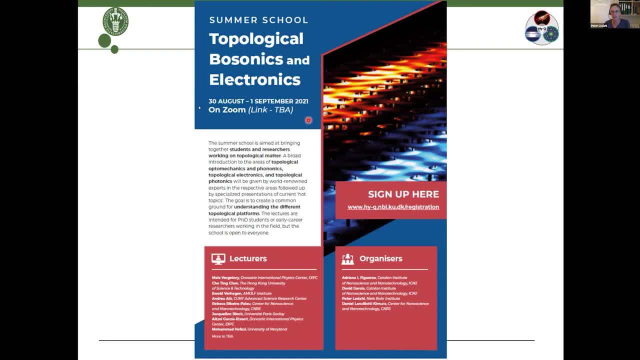 you're, you're changing this pulse with, and those are two different experiments where you're probing some of the same physics of, really you know, two pulses of light interacting with something with a bandwidth of a nanosecond. so there's another opportunity that also briefly said, that is, if 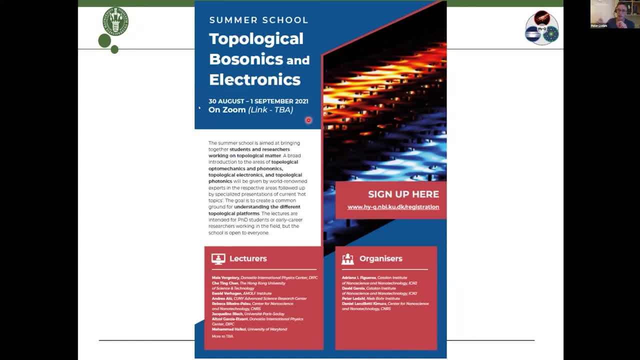 you have a spin. if you have a spin, then you have a longer memory time in the system. that would be a microsecond time scale and then, and then you can start to to also have, have, have, have more advanced. you can say photon, photon interaction, also on longer time scales, and 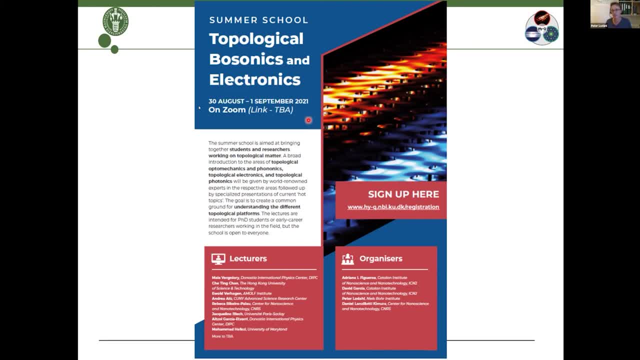 you can start to have more advanced. you can say photon, photon interaction, also on longer time scales, and exploiting this, the spin degree of freedom. um, i don't know if that's uh answer your question. yeah, i understand that this is a very complex, uh complex situation, yes, but you can. you can think of maybe, in the simplest case, if you say, a two photon pulse. 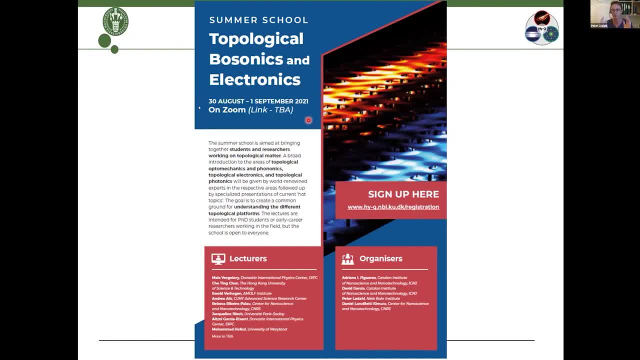 um, so, uh, that send up that that would have a certain duration. i'll say it's 100 picosecond, so that that that means that there would be a probability that the photon comes in the in the tail of the pulse, that comes early in the pulse, and that's all described by 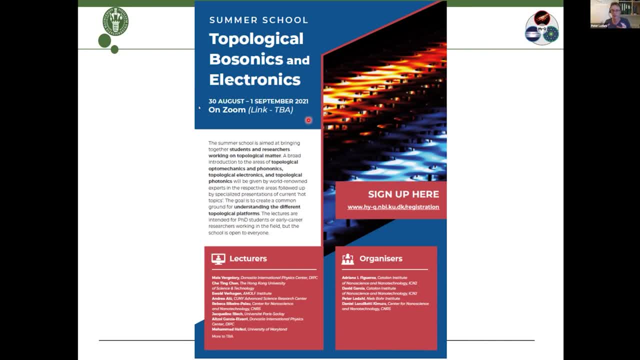 by this wave function that that you're sending into the emitter, and that is that that is this photon pulse interacting with, with, with the two level system that is, that is a. that is what you're describing, and it matters if you have two photons in this pulse, or three photons, or four photons, or 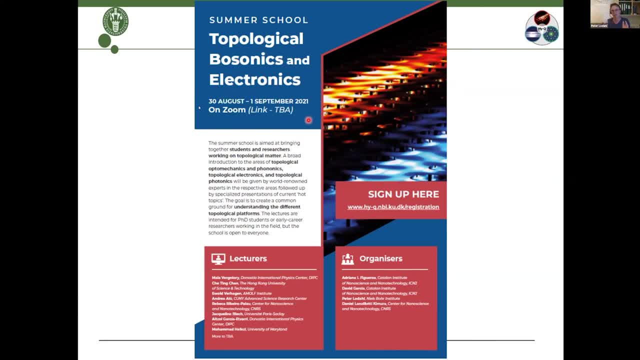 one photon, uh, and you, because you can think of the photons as not. they're not localized in time, it's not here, it comes right. it has a probability amplitude, uh, a wave function, and that is what goes into your, to your, when you're calculating that. that's a kind of the physical picture. two photon pulse will be distributed, uh, in time, and and and. 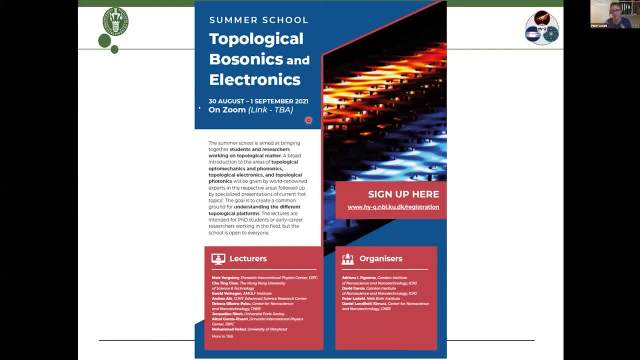 you, you should, you should have this and that's a. that's interaction with a, with with a two level system that has a bandwidth also, because that's the uncertainty on the transition. that's just one nanosecond i was talking about. that's gigahertz, bandwidth and frequency and it's those two. 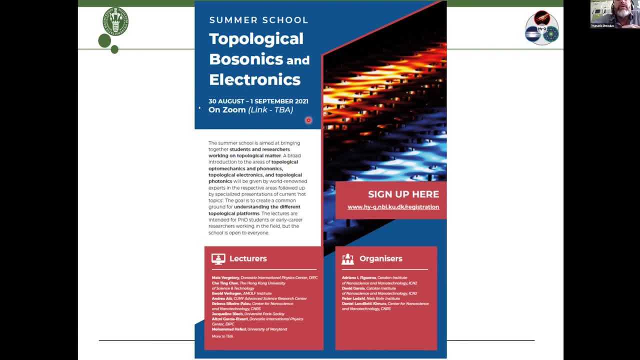 systems you're interacting with each other. can we also talk about amplification in this? uh, interaction between photons? oh, yes, yes, this is a wonderful question, uh, so, and a very non-trivial one, um, so, um, stimulated emission. so so i mean, we, we all talk, we all, we all see textbooks of 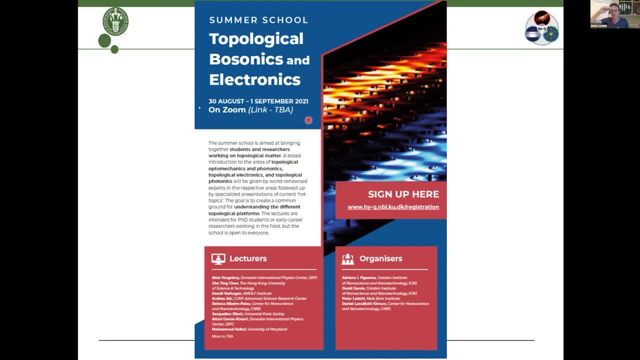 stimulating emission. there's a photon going in and there's an excited emitter, and how does that stimulate? and then a copy comes out of two, four. it's much, much more complicated in reality and that's exactly the physics you can describe here, because now we have interaction at the at. 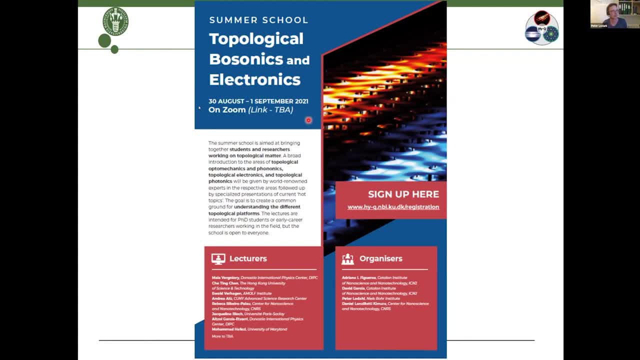 the few photon level so you can actually see and you can get a little um overselling it maybe, but but you, but you're rewriting the textbooks here and and really understanding how does, how does this picture really look like of of of one photon stimulating one photon stimulating one photon? 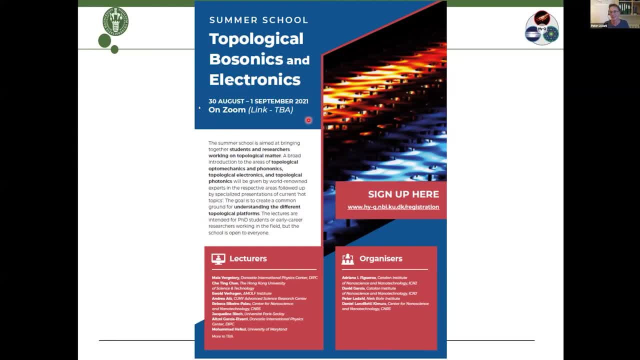 emitter. that that is. that is not the textbook. uh, drawing, it's something much, much more advanced and with degrees of freedom. asking this question, i didn't have in mind- so much sorry, you are falling out- the fact that in order to so you're, you're falling out. i. 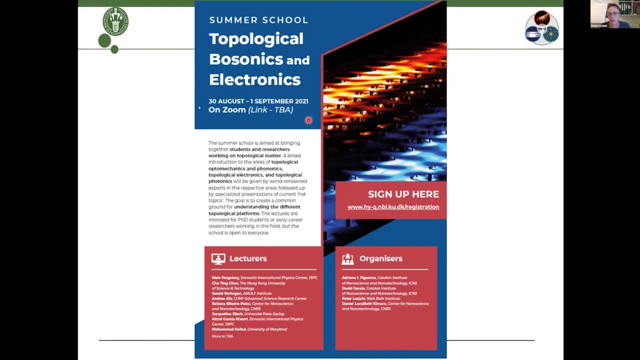 can add you, yeah, yeah, well, now you're better. i think now it works okay, uh, okay, when i uh, when i asked this question, i didn't have in mind, uh, so much the stimulated emission, but rather, uh, the um. i had in mind whether you can cascade. 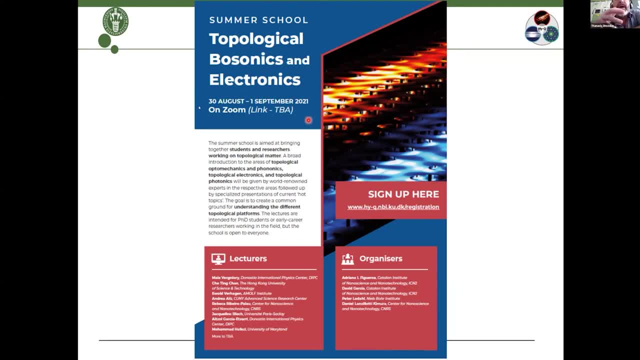 basically the uh, um, let's say the photon propagation over several um devices, to say so uh, because I expect to have also some losses, and so how you can compensate about these losses. I was wondering whether you have some amplification so that you don't need to. 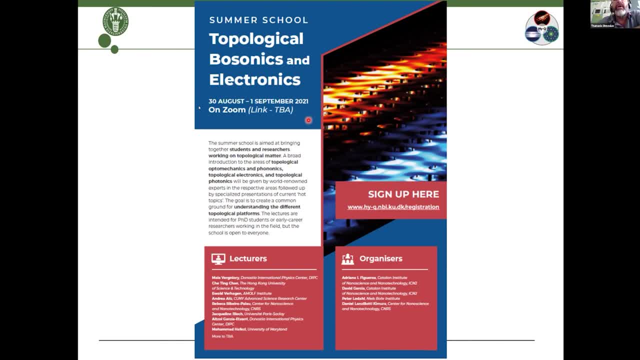 to worry too much about cascading the operation over several devices. Yes, so it very much depends on what you are after. So you can say in the: we are doing quantum information processing, so we want qubits, and qubits we cannot amplify, so there's no clone in CRM. and so I think 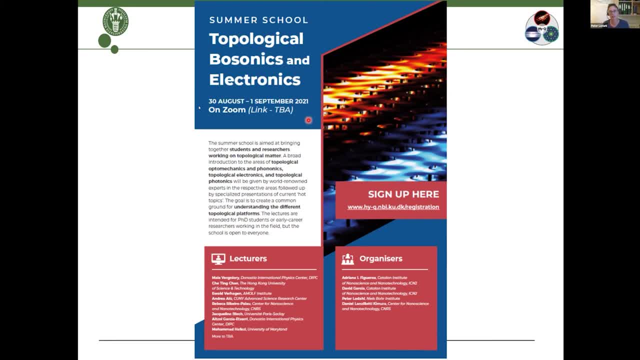 if there are other things, I think it depends on what you want to do So for, in general, these things that I'm talking about works pretty well for single emitters and few emitters, because it's really this local light matter interaction that you're. 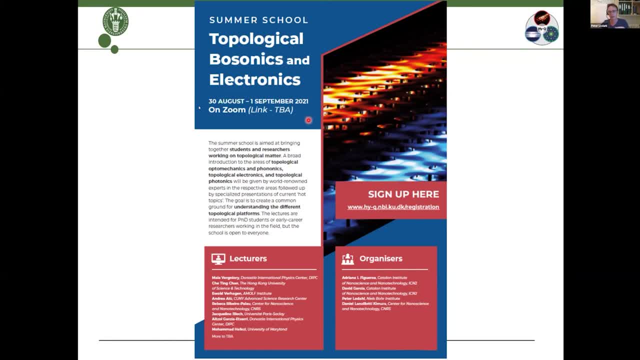 exploiting. If you want to take a much more bulky device, for instance, and make an amplifier out of that and make that directional, I would not say it's impossible, but it's a much more tougher challenge of getting this directional coupling over there. It's a much more tougher challenge of getting this directional coupling over there. 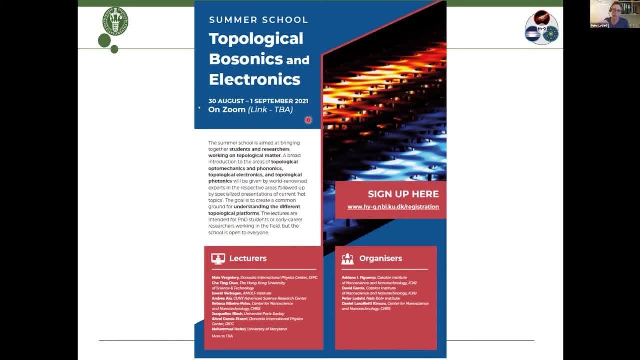 it's a much more tougher challenge of getting this directional coupling over there very extended spatial area. It works so extremely well in my case because it's just a few nanometer quantum dot. That's the interaction that we are engineering. If we wanted over 100, 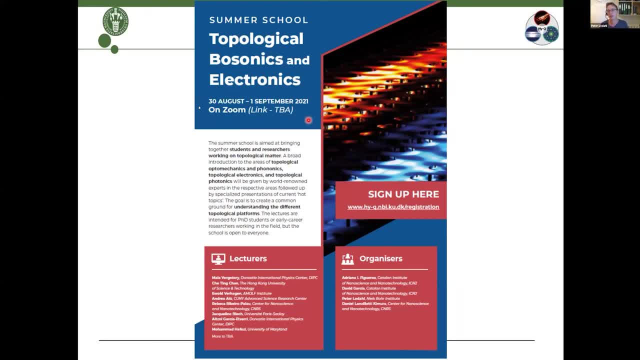 microns. it's a different. it's a quite different game. It's not something we have been looking into at all. I would not say it's impossible, but one would have to certainly not jump to conclusions that this could just be absolutely a game changer or anything. 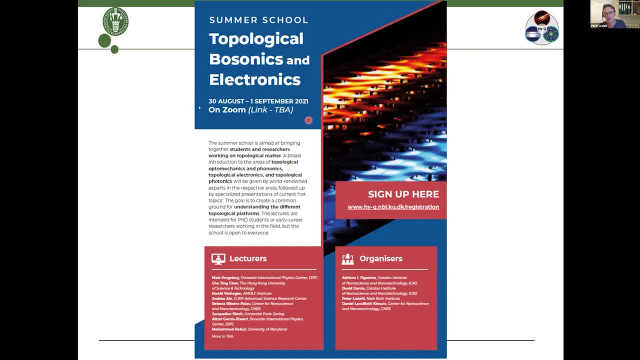 like that, My suspicion would be there will be no free launches there. Thank you very much for this inspiring talk. Thank you, So you have two questions to raise hands. Okay, On the right, So can please just speak the? I'm not sure I see them. 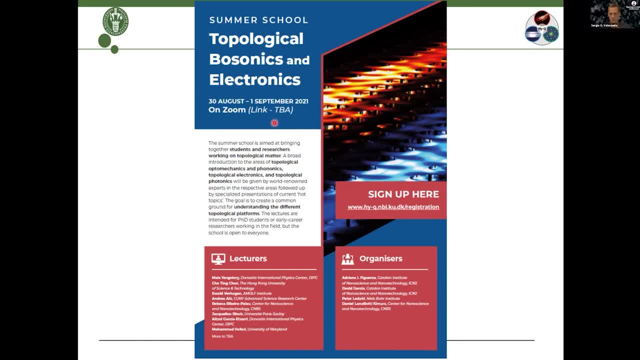 Clivia Sotomayor is the first. Yeah, Is that okay? Yes, Good, Okay. Well, thank you very much for this very entertaining and very comprehensive lecture, Peter, Thank you. I have a question concerning, like in the spirit of torture. Well, you have two questions. One is the size of these structures. 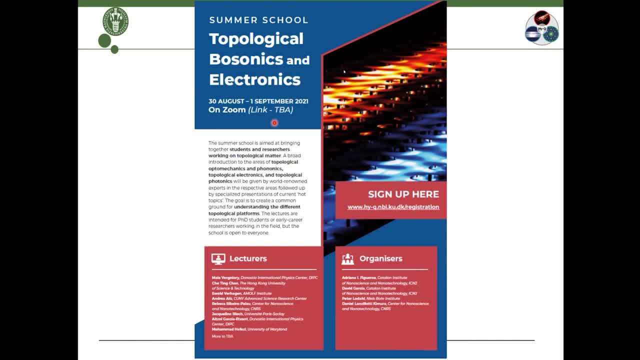 what technically is people call footprint and how one can integrate it into something that will be looking like an application. I mean, you have some examples of integration, but it's very partial, and when it's a schematic, I think Yes, Yes. 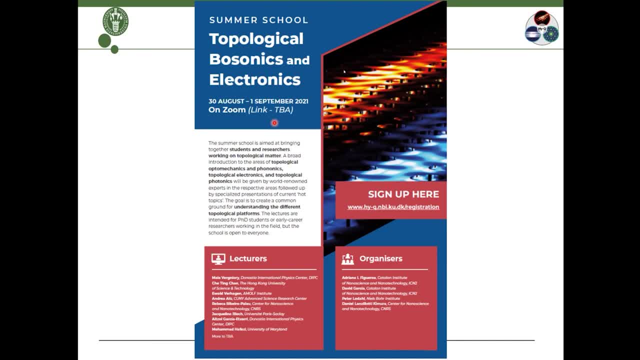 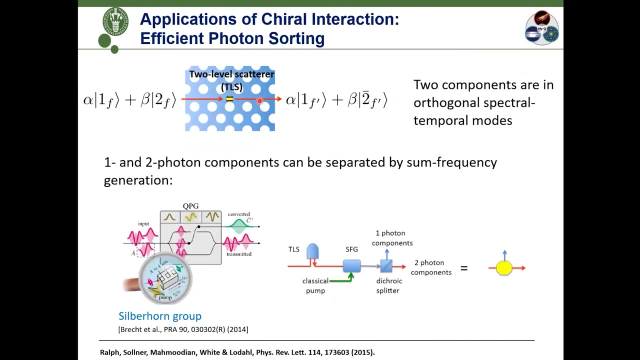 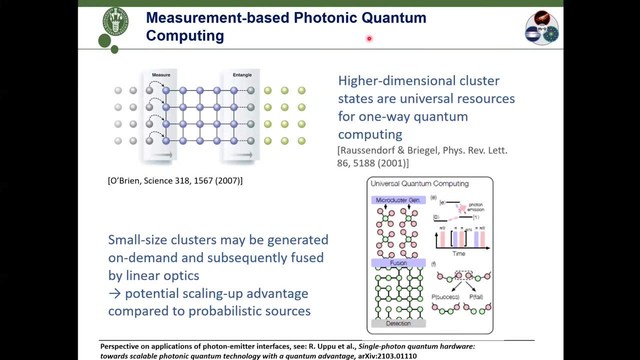 Yeah, So that's my first. My first question And my second question is: there are concepts which are intrinsic to topological matter and concepts that are intrinsic to quantum optics or quantum photonics. What would you say are the key concepts we need to have in mind concerning topological photons? 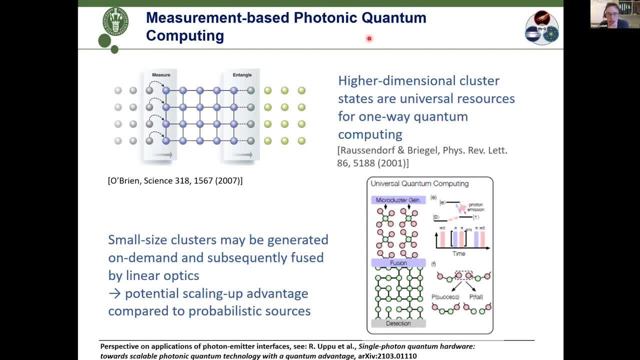 That's the second question. Yes, Let me start with the first one. So, yeah, sorry, just to hear. So what was your question? Footprint, Footprint, Yes, Yes, Thank you, Yes, Sorry, Yeah, So these devices are small, So typically. 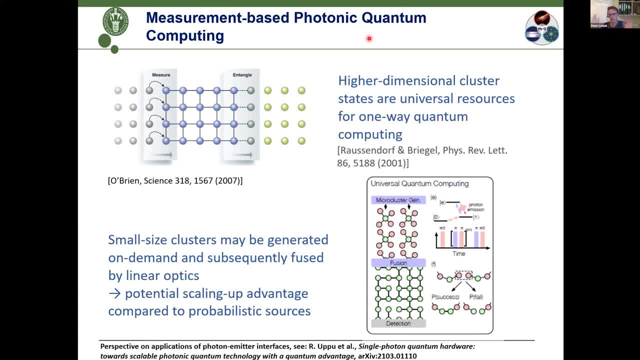 you know the short waveguides would be, I mean, 10 microns or so. That is perfectly fine to get this very, very high light matter interaction strength, Yeah, And it's also fine in relation to the disorder in the system. So 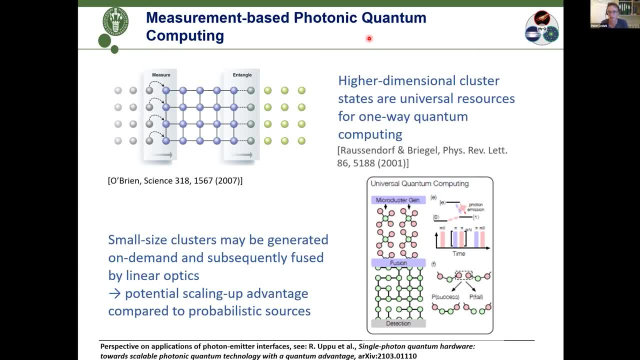 this is one of the things that we are very interested in touch here also. you know scattering mean-free paths, So maybe it's 20 microns or 30 microns, depending on how much low light you have, and so on. Maybe I can push these boundaries so I can get a. 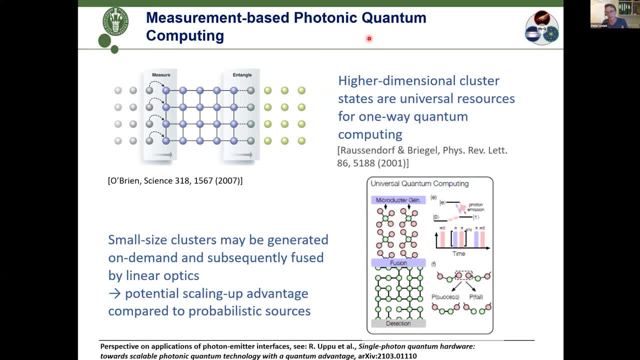 longer scattering mean-free path and still have slow light and I can push the numbers a little bit. And I think that's important to do, because there is room already, because we can make short devices and we can get excellent single photon source, multifoliam entanglement sources, But giving us 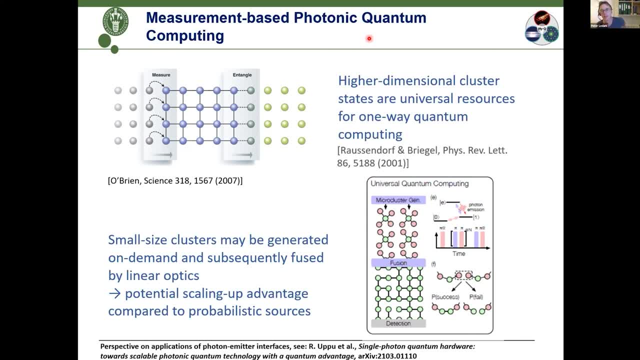 more space. I think it's an important thing, And even a factor of 5 or 10 or improvement could be quite substantial and important. I mean, it's also about, of course, improving your fabrication process even further. This is something that we are just starting on. 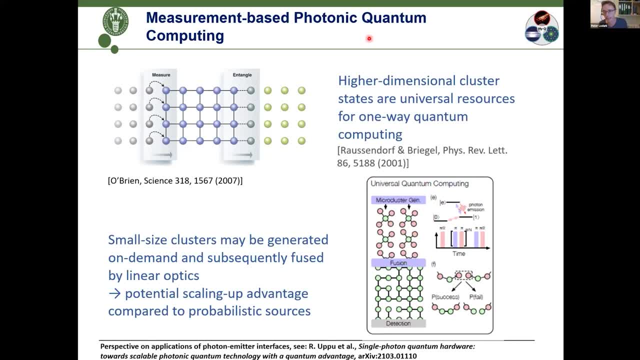 OK, Yeah, Right, Yeah, Yeah, Yeah, Yeah. all is done in university labs and so on. so i think it's quite nice what can be done already there, and if you really push some, put some engineering efforts into that, i'm sure you could. 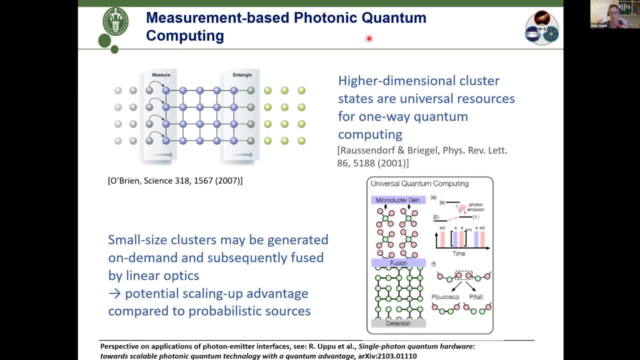 be doing much better, so, uh, so so the footprint is is really, you know, small devices and and, and there is already room uh, to, to, to to produce hardware for, uh, i mean this little non-reciprocal uh device that i showed would be something that is, uh, you know, 10 micron long, um, and, uh, and and. 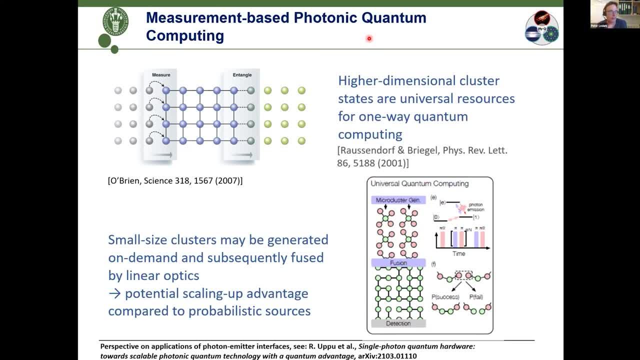 that you could interface, because i think that that's that's the other important point here and that's a very good point. uh, i i'm not imagining that, that we would, you know, build on this, on this platform gallium arsenide platform, the whole photonic quantum computer, or anything like that. 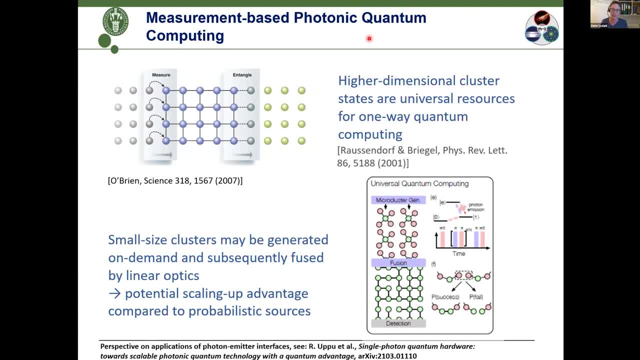 i think you would like to interface like a, a hetero, um, uh structure, or what you call it um. i mean interface the, the, the active devices that we are having here, to to, for instance, uh, silicon nitrite and and ultimately silicon photonics. i mean, our wavelength is not that silicon compatible with silicon electronics? 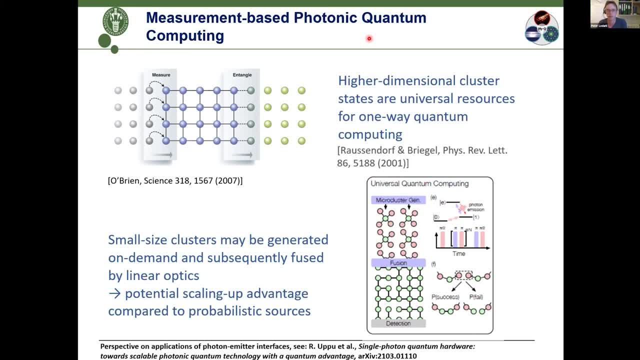 today, but this is something that that will change in the future. i'm not, i'm not worried about that, so i'm we're thinking about um, an approach where we are making these source devices and we're interfacing it with advanced quantum uh, with advanced um, um, photonic integrated circuits, uh- to do advanced quantum processes there. 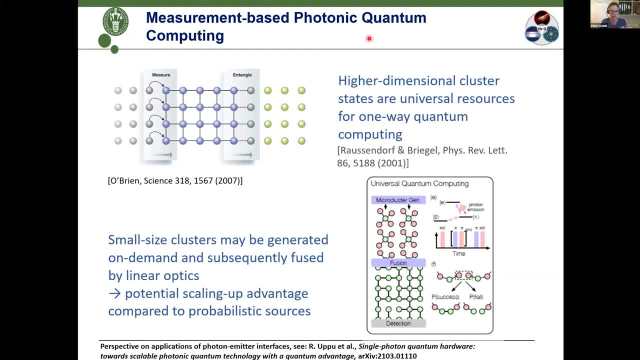 so really in a heterogeneous approach where you have sources, you're building more and more functionalities on the sources and then you're coupling that to silicon nitrite and silicon photonics for for for more advanced photonic processing. that that is very much the opportunity that i see and i i think that's a very good point. um, i think that's a very good point and i think 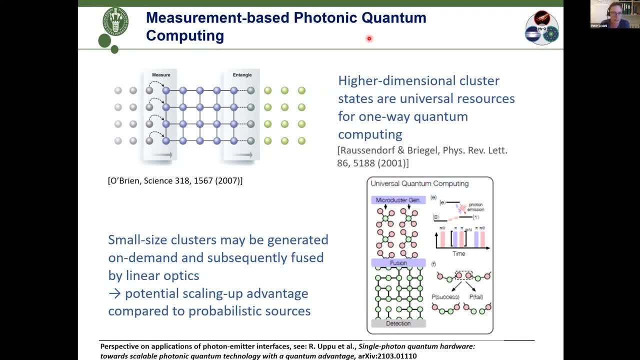 i i went to this slide here because this paper that we put an archive is is exactly on on this vision about heterogeneous um approach to quantum computing: uh, ultimately, where we think we can produce deterministically with these small devices, uh, advanced photonic resources in a much. 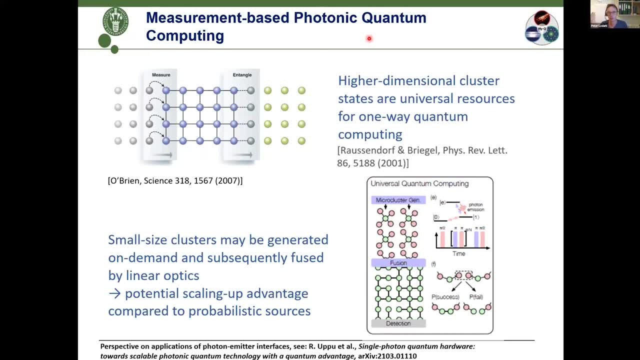 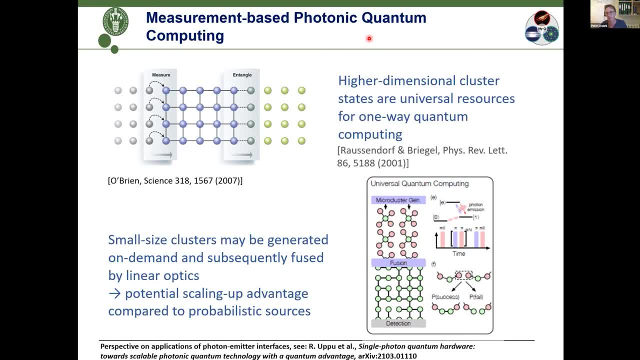 in the us as i quantum, uh, that is really, you know, pushing photonic based quantum computing and making lots of effort on the on the processing side and, i think, our deterministic sources. there could really be an add-on, uh that that would fit very well into to their architect, as you can say. 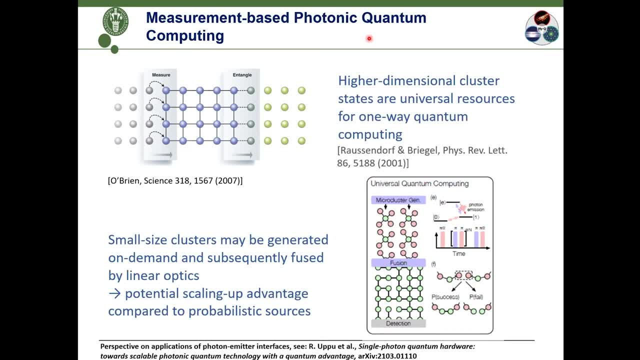 um, i don't know, did that answer your question, clevia? yeah, yeah, to some degree, but i think basically, the bottom line is that we are going to vary heterogeneously- material wise, technology wise, yes- in order to meet, uh, integration, compactness and, of course, 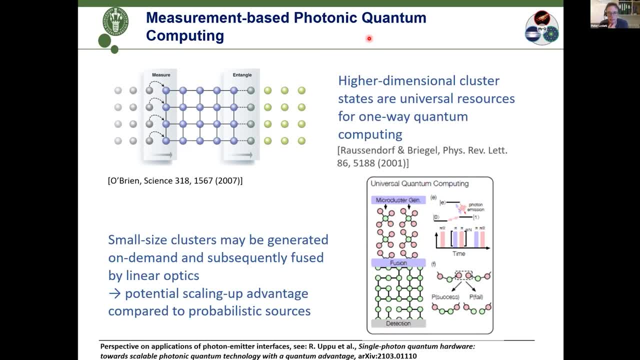 the performance? yes, quantum computing type: uh, photonics application: yeah, so my second question was on the concept. so yeah, topological matter, topological bosons and the quantum photonics, quantum computing, the overlap: where do you see the overlap? yes, um, yeah, there, i'm, um, i'm also. uh, i don't have very clear visions there. i would say i. 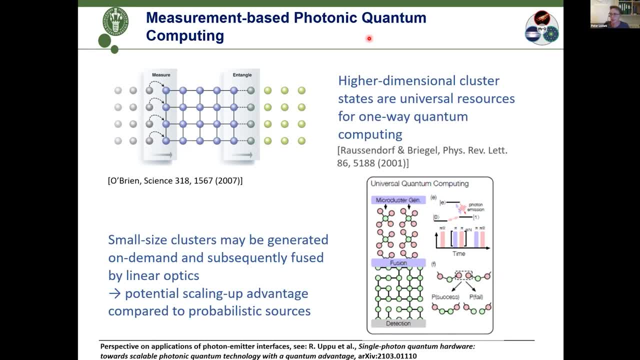 so for the, for the directional emission, uh, so this kyle light matter interaction, this is, this is a neat tool. uh, that that that that is very practical also for for many of the devices. topological photonics enables that, uh, but, and you don't need topological uh devices in order to do that. 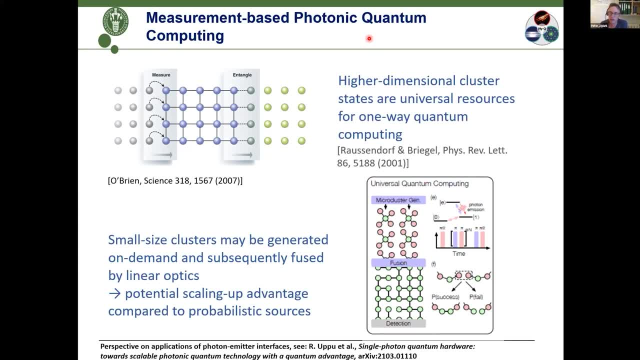 i think that what i was saying there in the beginning, the the uh, back scattering, uh, if you, if you can in, if you can use some of the, the notions or ideas from topological electronics and topological transport there to to uh, to reduce back scattering in the devices. and therefore i'm 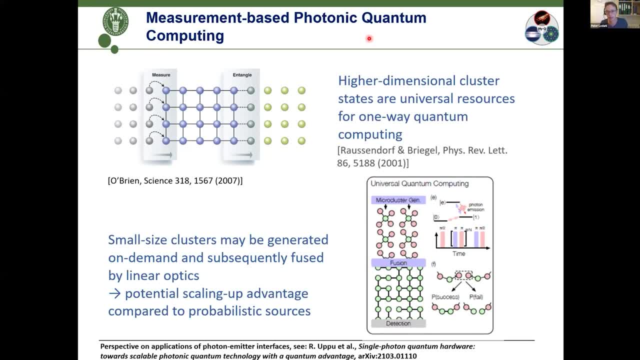 increasing uh, the, the, the length, and you, uh, clevia and david, have been doing- uh, i see i've been doing interesting work really, really on this. if, if you can, if you can exploit that, i think that could be all. that could be a nice thing and a practical thing. um, i, i i'm also actually uh, um, surprised how. 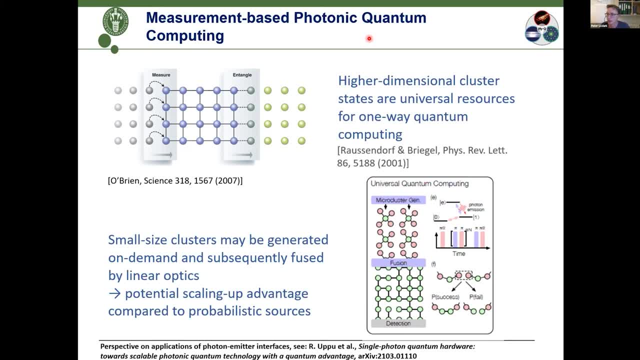 how, uh, we're just starting, as you know, and also these kind of measurements, and, and actually it works better than what i had thought, because you have a quite advanced um structure, quite a ranch wave guide there, and, and, uh, and and. this mode is quite complex, but we actually managed to couple it, it seems quite 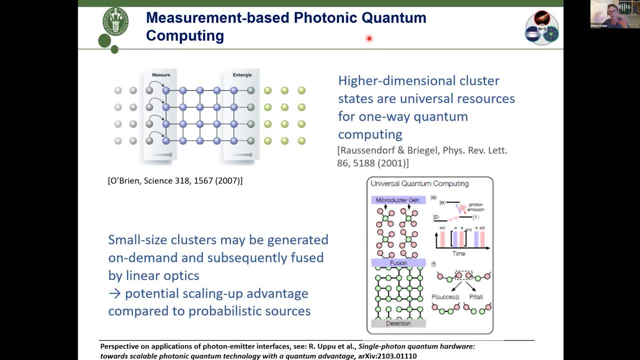 efficiently also out of the device, because that's one thing you have to worry about. you have an advanced mode, but can you actually couple it to something so that you just don't lose it somewhere at the interfaces? and so that seems to work better than expected. so it could be that some of these um 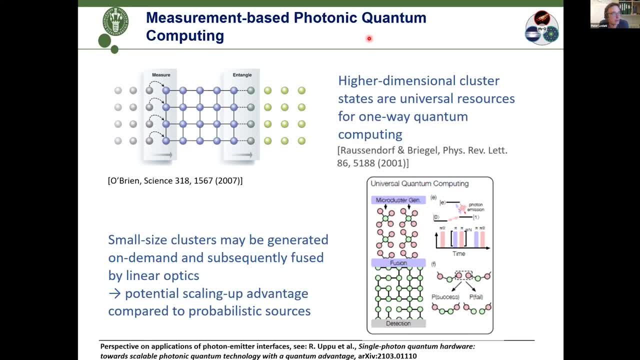 isolators that i also mentioned, um, that, that and that there could be some opportunities there. um and uh, as i think we also talked about, you know, trying to engineer a structure that absorbs very well by coupling it to an electronic, uh degrees of freedom, potentially that, that that would be. 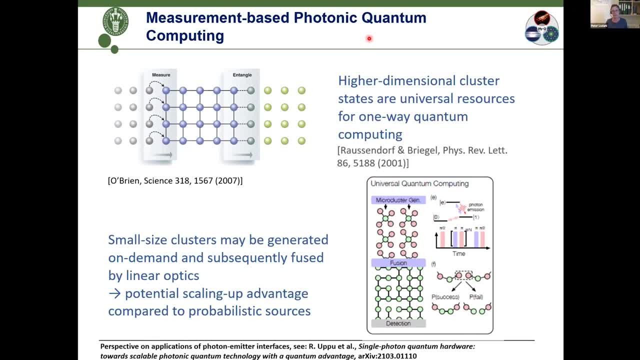 interesting to look into, uh, and that it was very much this idea that that i also presented- from whether you use atoms as a as a absorber, as a as a dissipation that just scatters the photons out of the system. but that could be done in. 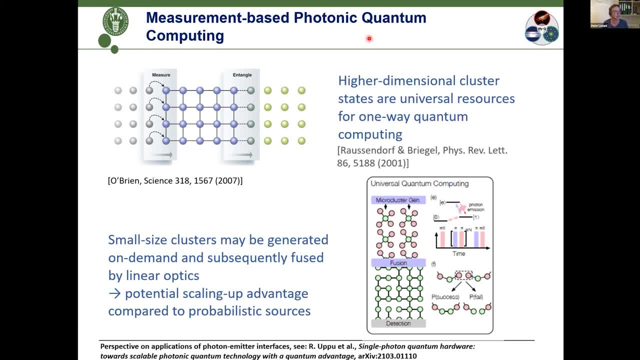 in other manners as well, and i think that that would be interesting to to look at. um, yeah, that's probably the best i can think of. thank you, peter. we can discuss some other time. absolutely, yes. there is another question from uh nutachai judong. are you there? 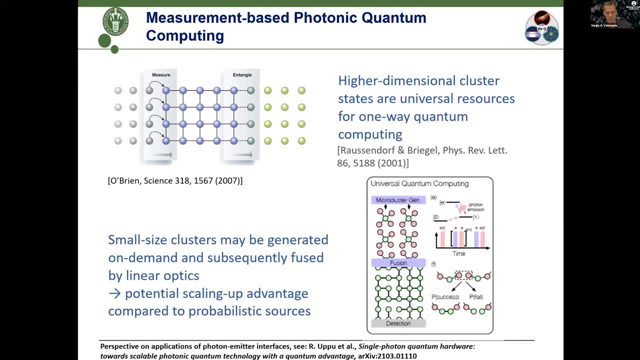 we give you the microphone, you can go ahead and and, uh, unmute your microphone and ask your question. um, okay, it seems that it's not there. i think there are some people coming in and out on the. on the link, open discussions with peter. you have the link in the email that was sent a few days back, but 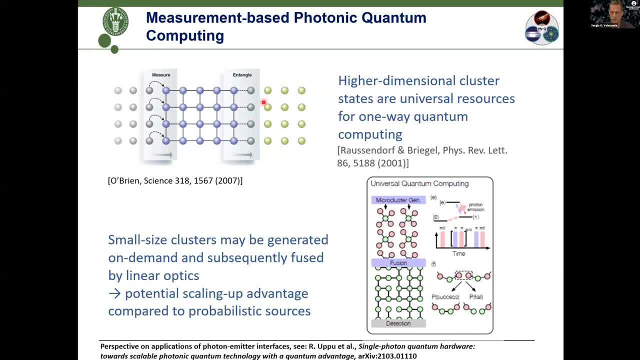 also you can find it directly on the on the zoom chat, so you can click on there and and they go to to that link. okay, sure, we'll do that, okay. so it seems that, yeah, you should. yeah, so this is for, uh, for nautica ideas. go ahead and and go to. 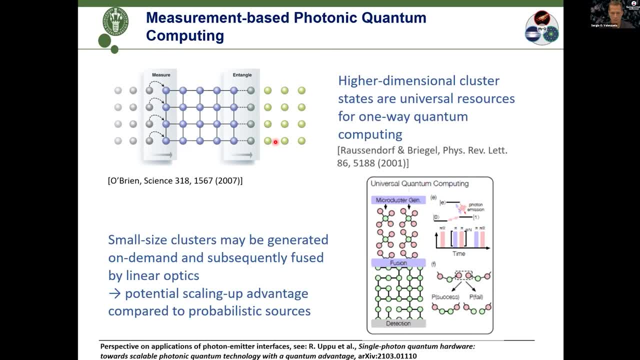 the to the to the other meeting to ask your questions there. sorry about this. see ya bye.